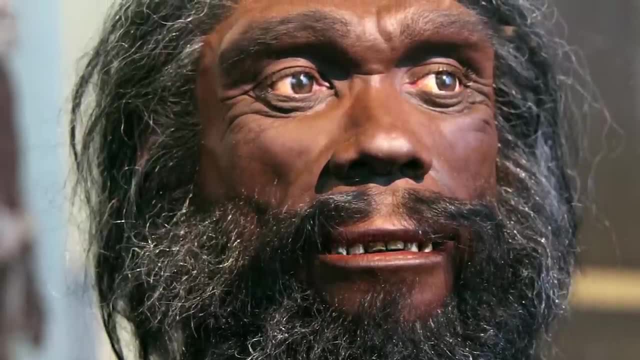 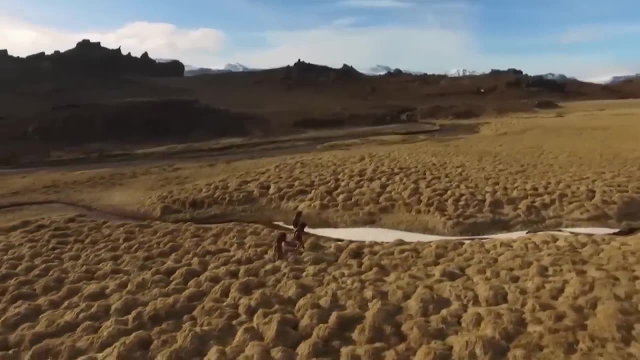 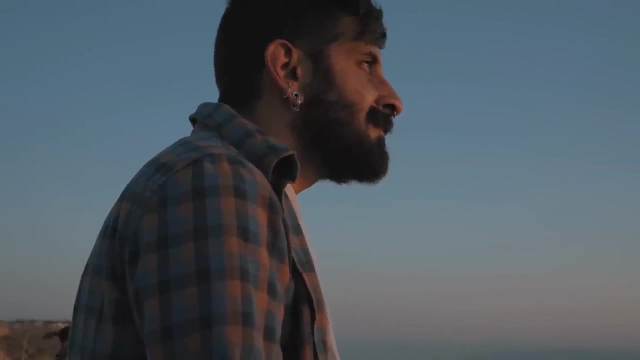 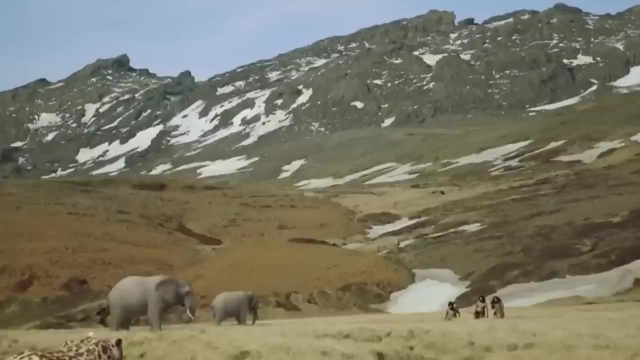 the idea that Heidelbergensis could indeed be a subspecies of Homo sapiens. In today's video, we will be exploring the life and evolution of Homo heidelbergensis, examining just what makes it so similar to our own species. We will look at how this species may have lived, where it lived and how it was discovered. 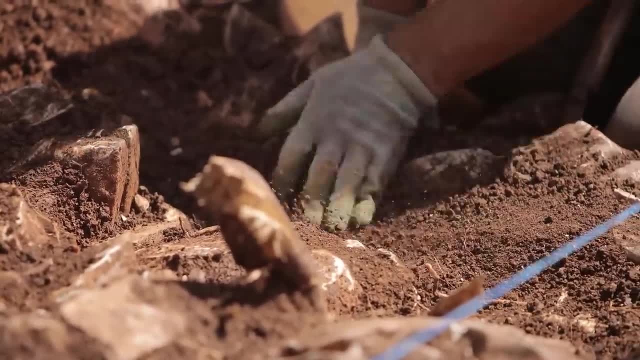 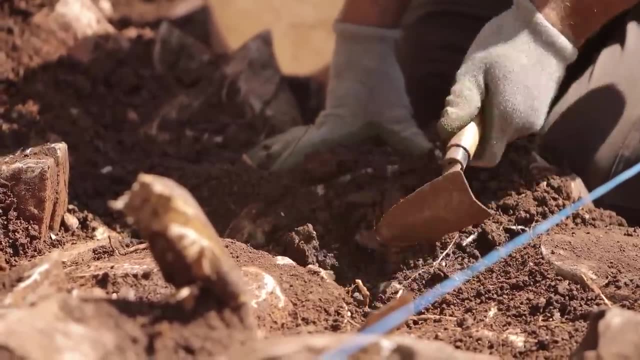 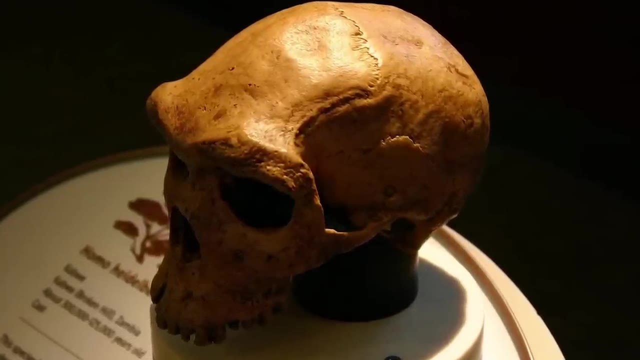 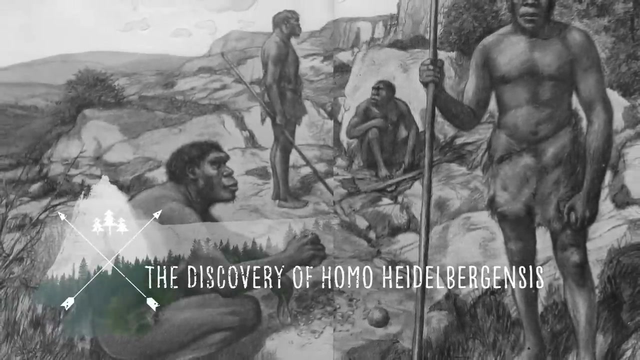 Although this is an archaic human with much to teach us. a wealth of information has been discerned from skeletal evidence And we will be examining this information to put together Homo heidelbergensis' story. The mysterious and disputed Homo heidelbergensis has been known to modern humans since 1907,. 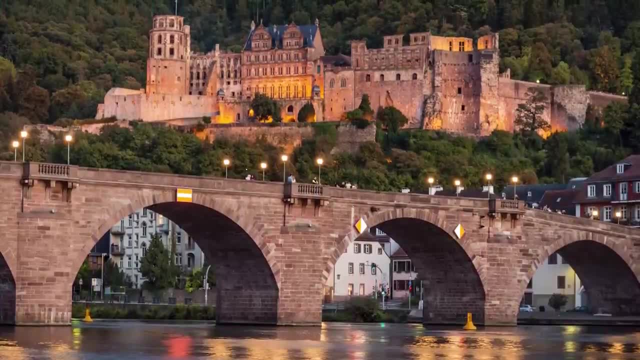 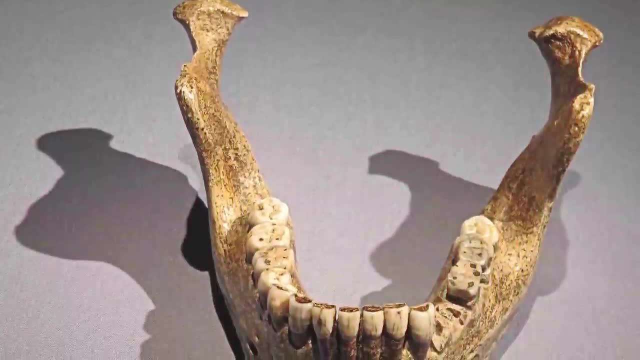 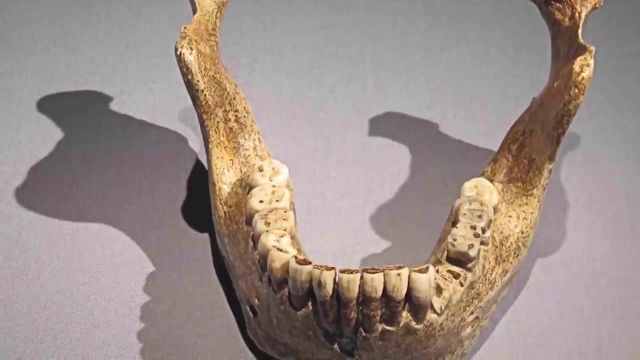 when an industrial worker in Mawa, a village not too far from the larger city of Heidelberg in Germany, uncovered a fossil jawbone jutting out from the rocks he was working in. Noting the importance of the find, the man extracted the bone from the rock and brought 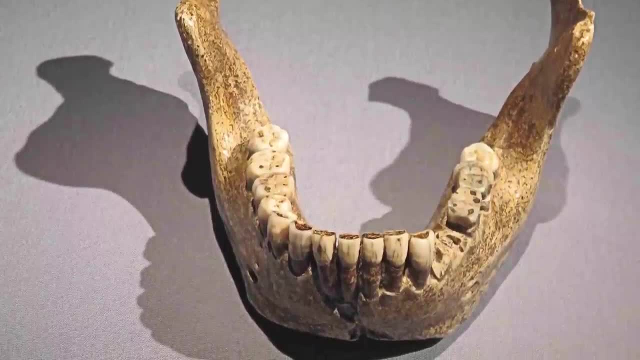 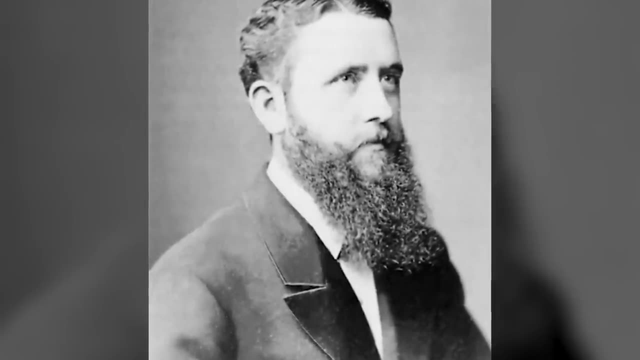 it to the famed anthropologist Otto Schottensock, who in the following year officially named and described this species as a new archaic human, giving it the name Homo heidelbergensis. Translating into German, the name Homo heidelbergensis is the name of a human who was born in the 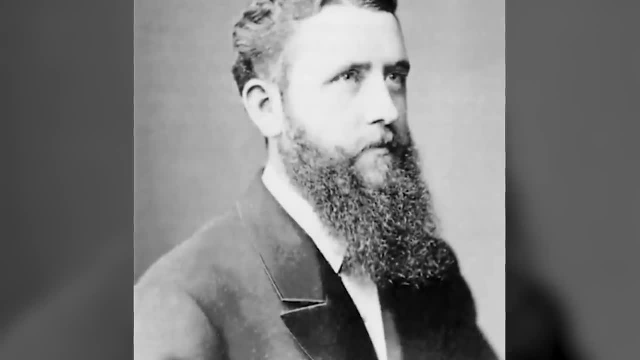 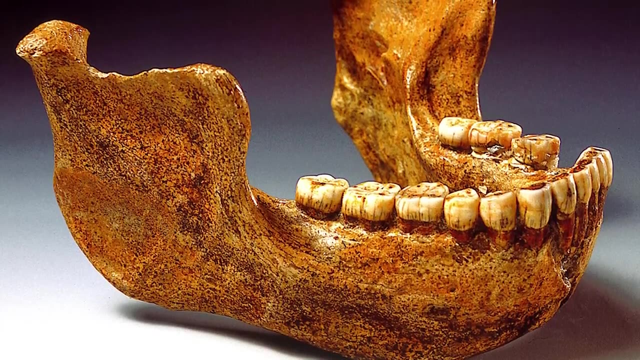 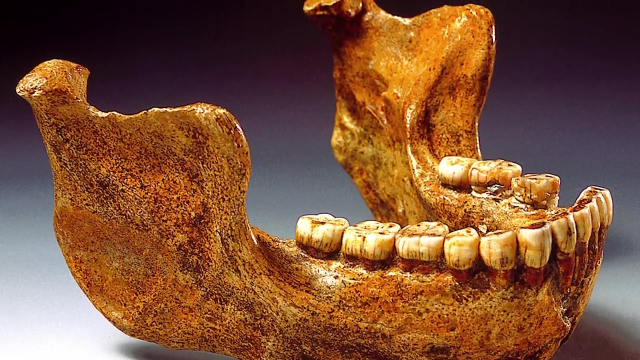 19th century, Translating to English as Heidelberg man or the man from Heidelberg. The bone in question, a lower mandible jawbone complete with a nearly full set of teeth, is thought to have belonged to a young adult of the species in life determined by Otto. 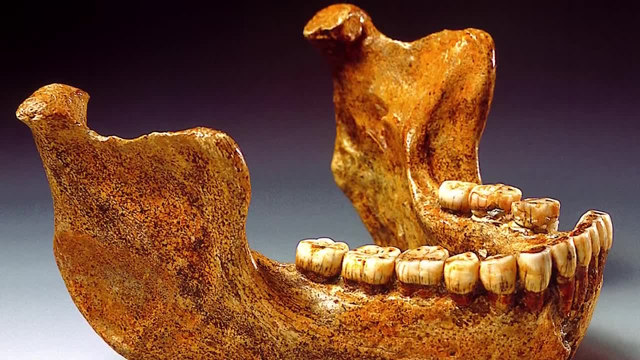 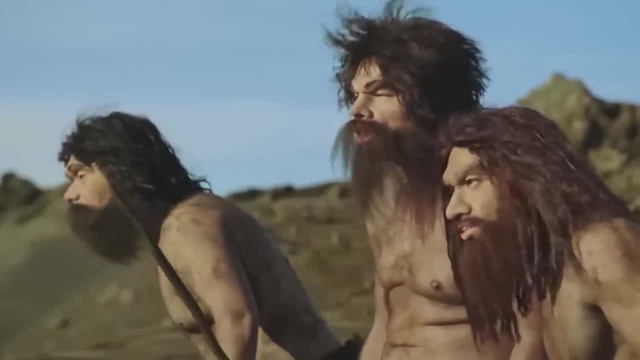 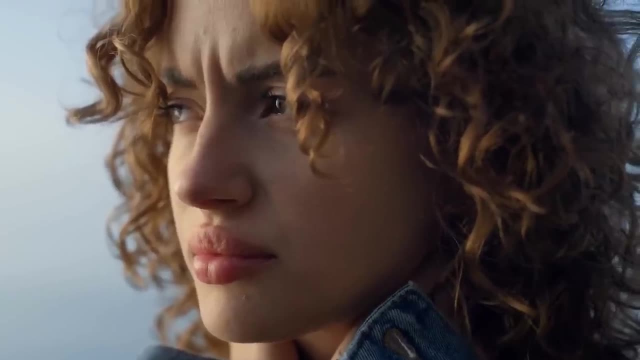 Schottensock, based on the lack of wear and tear on the teeth. What prompted Otto to classify the Heidelberg man as a new species of archaic human was the proportions of this jawbone, Compared to the mandible of a modern human. Homo heidelbergensis was huge, with a much 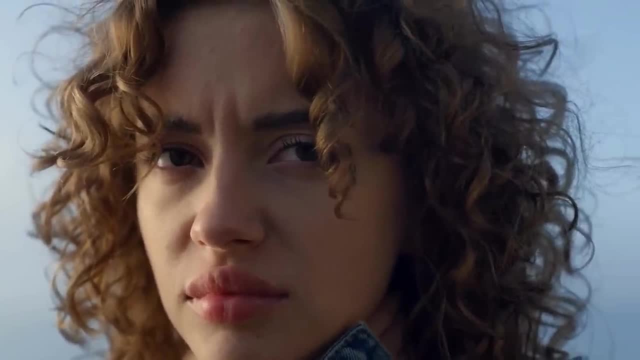 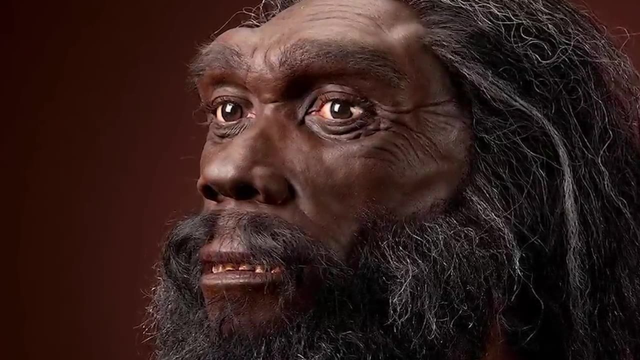 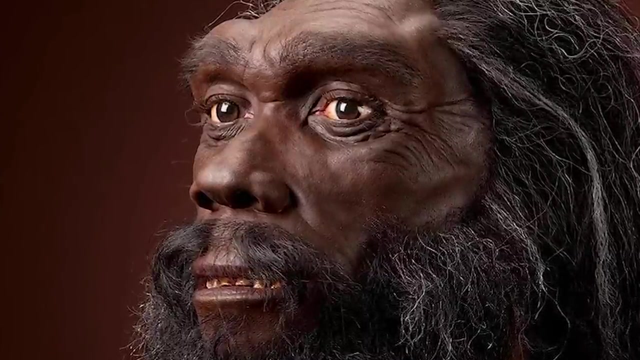 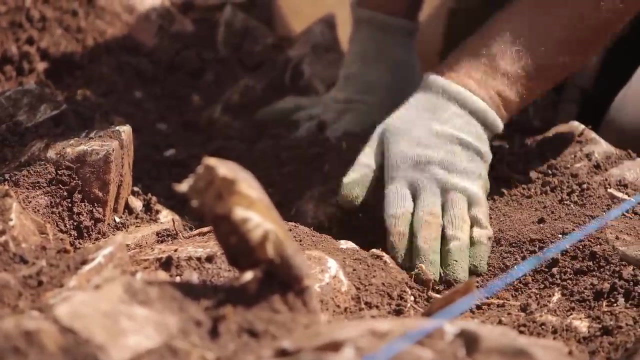 bulkier form and shape to it than ours. If we ignore the controversies that have come out of this convoluted discovery for now, then several other specimens have previously been assigned to Homo heidelbergensis. The best known of these specimens are fossils, mainly skull remains discovered from various 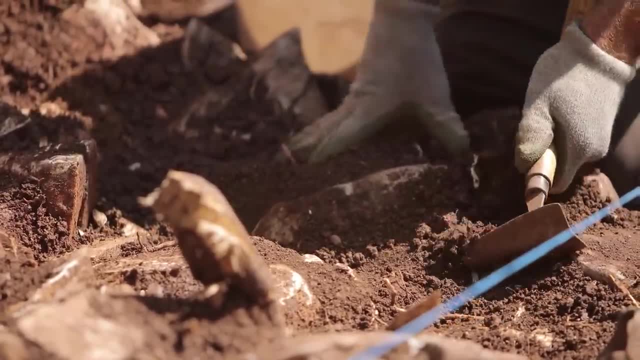 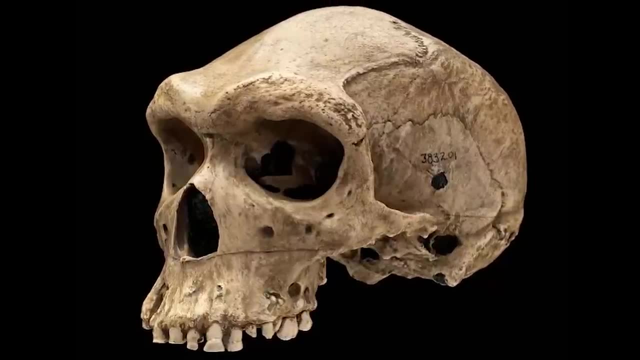 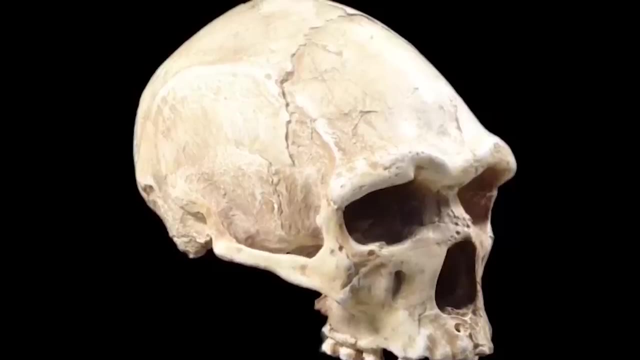 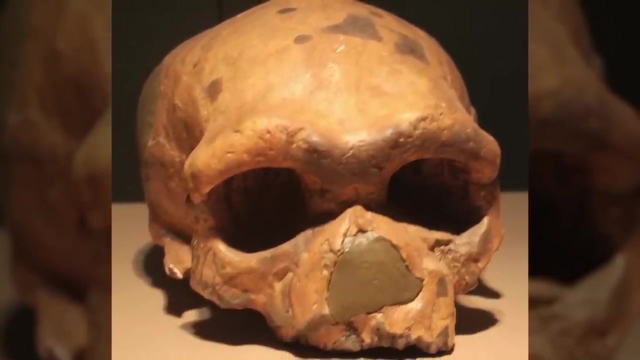 locations across Africa and Eurasia. Bones from Bodo in Ethiopia, Kobwe in Zambia, Ndutu in Tanzania, Petrolona in Greece, Aragu in France and Dali in China have been uncovered across the course of time Since the original mandible was discovered. 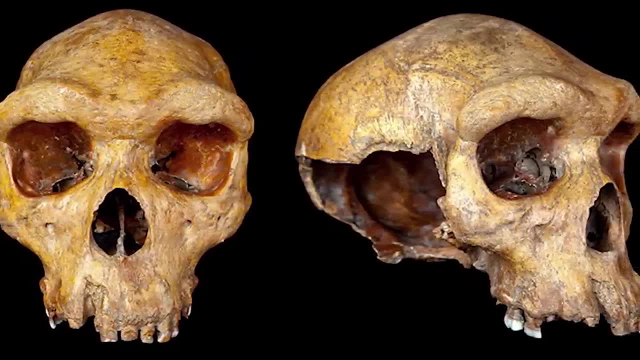 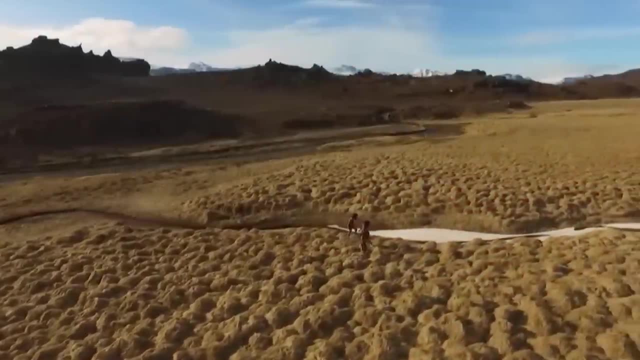 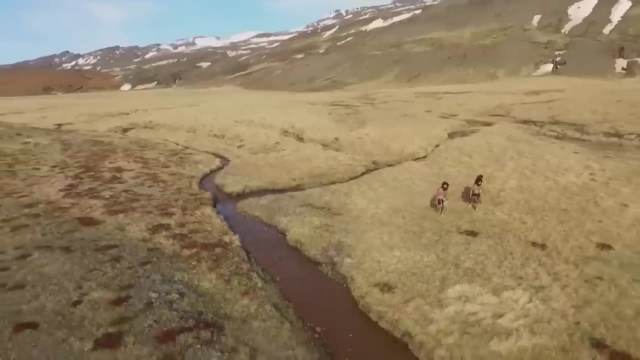 All these bones share remarkable similarities, specifically in the brow, ridges and brain cases of the cranium bones. But Homo heidelbergensis is a species with a long and complicated history of debate, as we shall soon discover. Before we explore the complications of the long history of Homo heidelbergensis, there is a small point to be made. 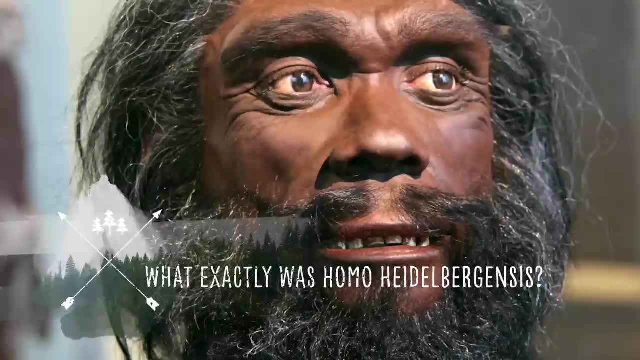 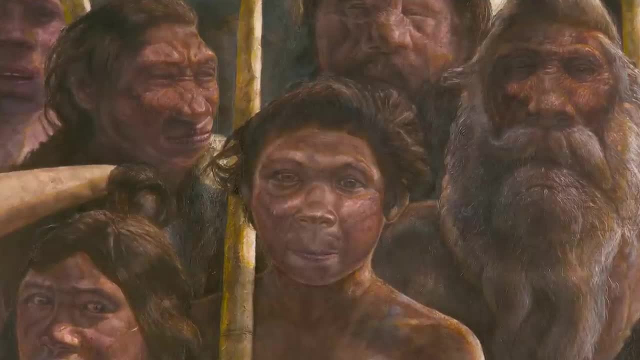 I will first discuss the warum Leibniz-Tuber, but before this I will comment on reasons for the use of the name, for the name of this heavily disputed species. let's take a look at what these scientists are working with. what actually was homo heidelbergensis? what did it look like and what can we discern about the? 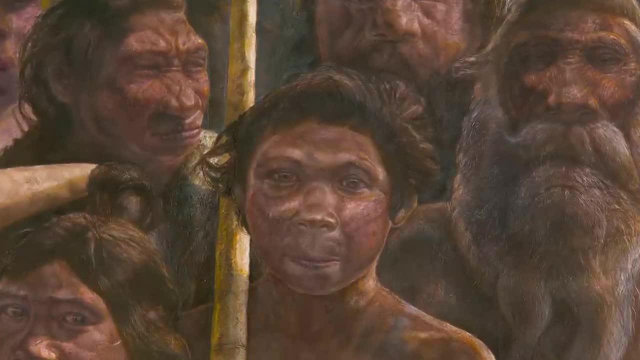 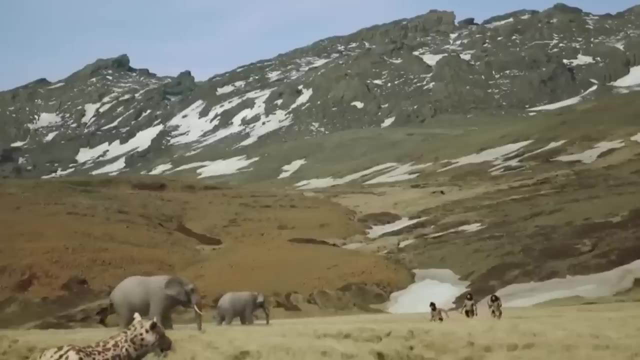 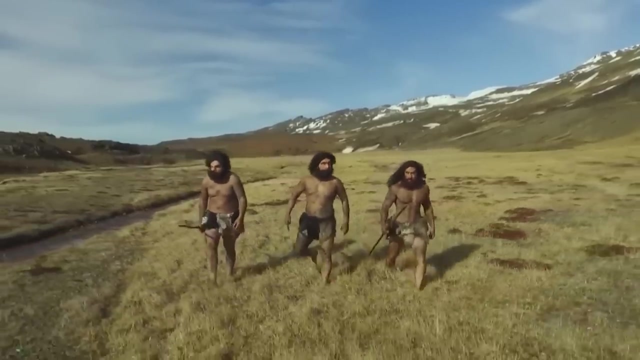 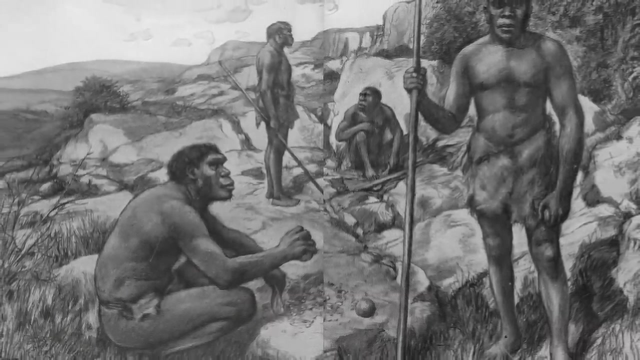 species appearance from the bones we have assigned to the species so far. firstly, the basics: homo heidelbergensis was a species of archaic human who existed in the middle pleistocene epoch of the cenozoic era from around 700 000 to 200 000 years ago. from the skull bones discovered across: 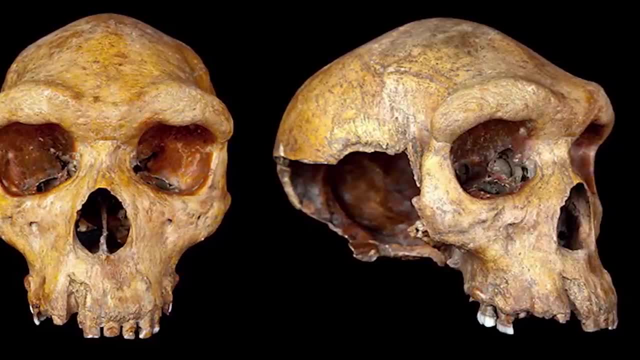 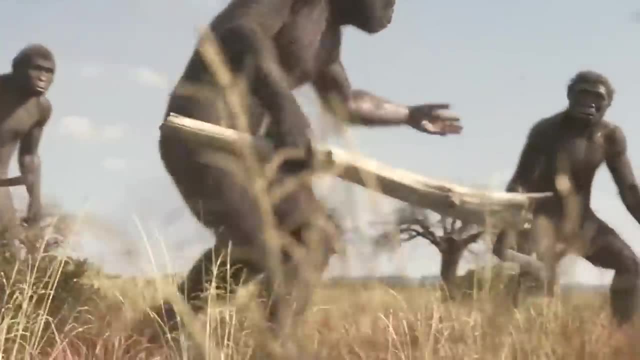 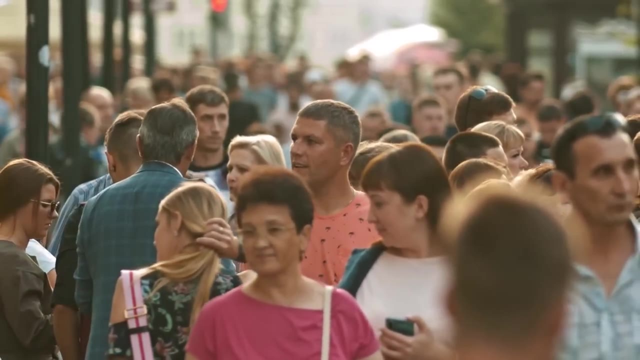 africa and eurasia. scientists have been able to determine that, in contrast to earlier species such as homo erectus and homo habilis, homo heidelbergensis would have looked very similar to a modern human in life. on the skull bones, the nasal openings are vertically set, sometimes with a prominent crest. 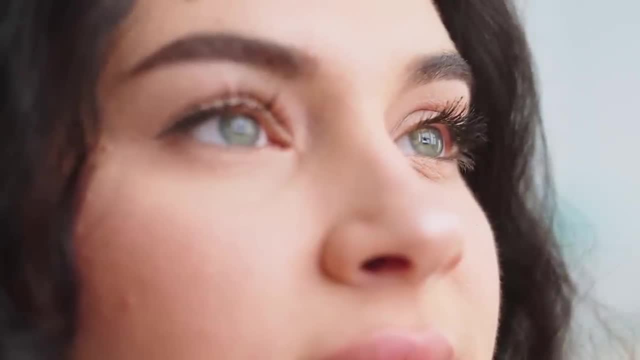 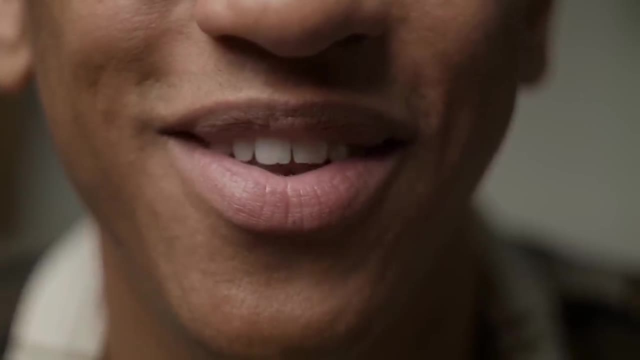 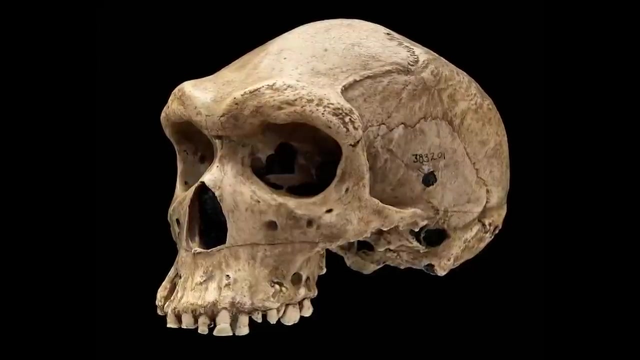 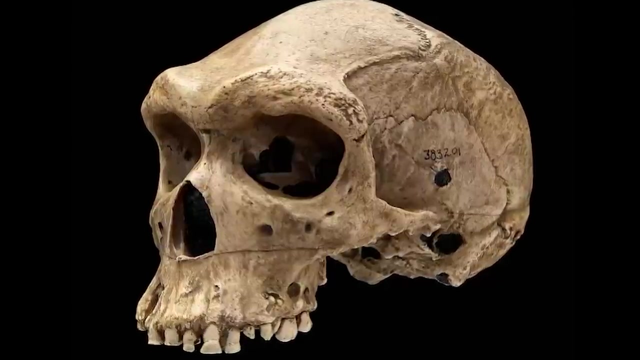 the attachment points for a nose very similar to that of our own. the teeth often well preserved in the skulls are similar and oriented in a very close fashion to that of our own, and features of the temporal bone on the skull skull indicate that the brain case of this species was rapidly growing. not only did these humans look 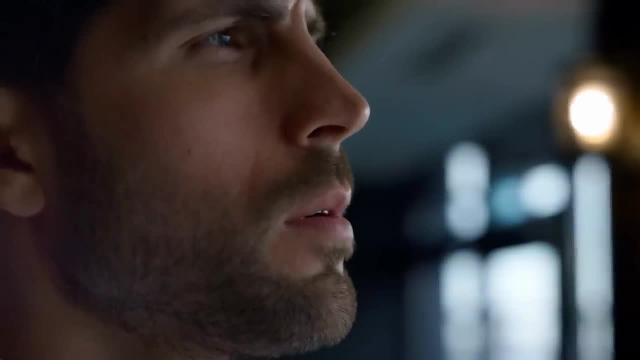 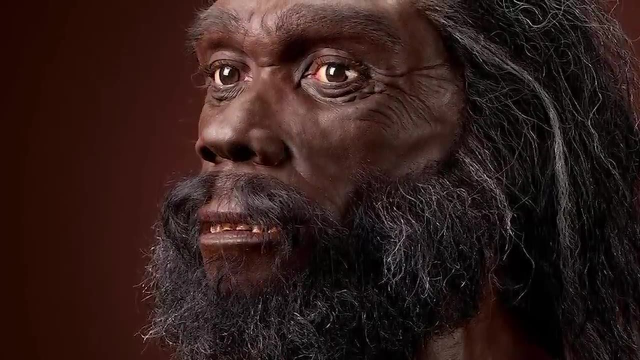 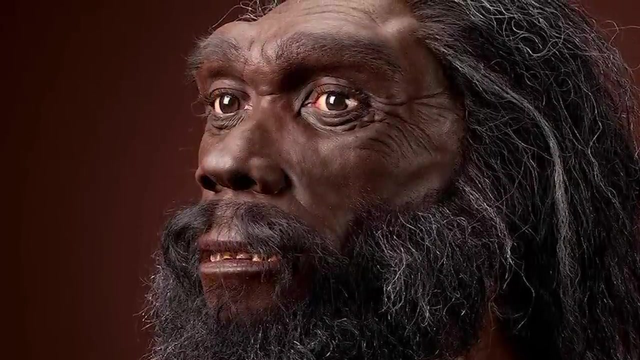 like us, they were beginning to think like us too. paleo artists and scientists have even been able to piece together lifelike busts of homo heidelbergensis head and face based on fossil evidence. some of these can be seen at the london natural history museums exhibit on human evolution. 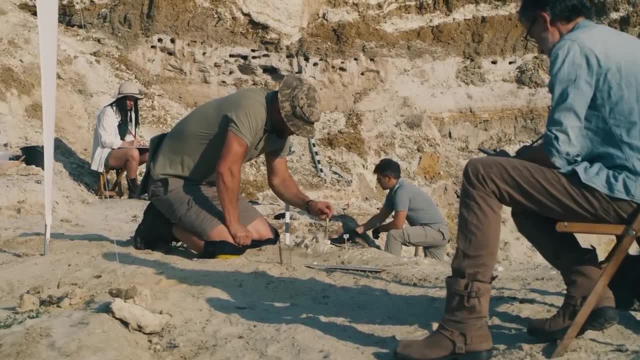 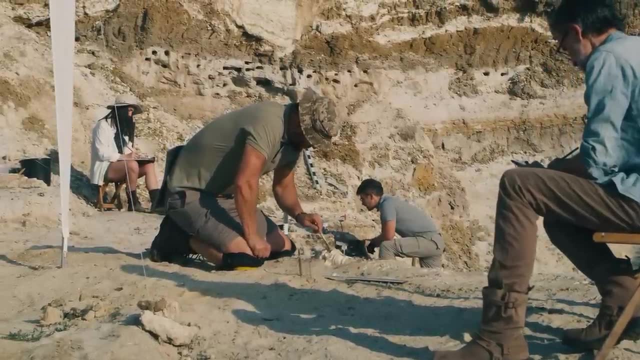 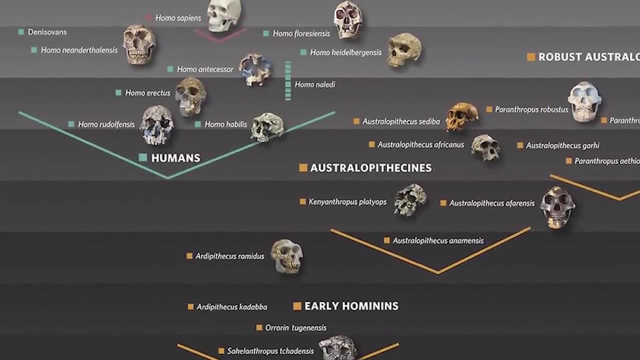 although scientists have not yet uncovered many bones from the torso and limbs of homo heidelbergensis, they have been able to infer what this species may have looked like in full based on its position in the family tree, using older and later species to determine a body plan. 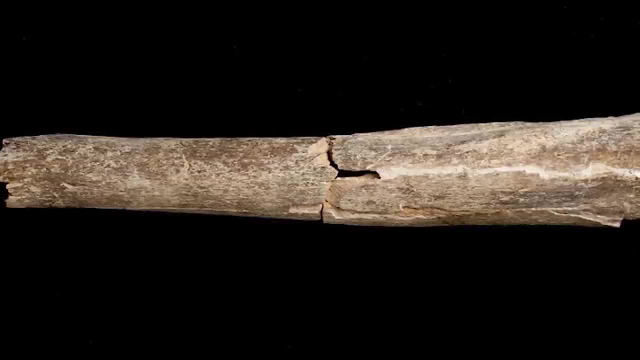 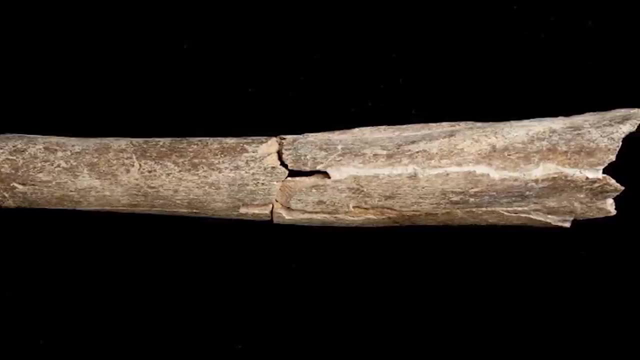 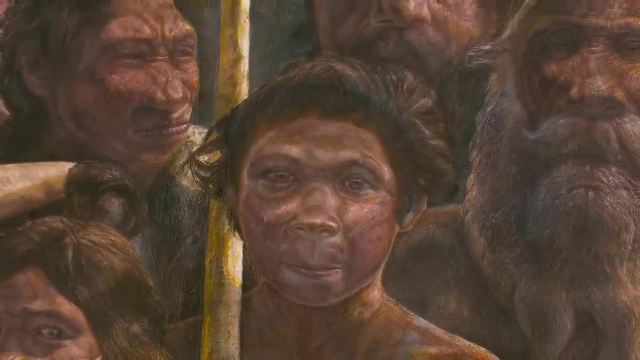 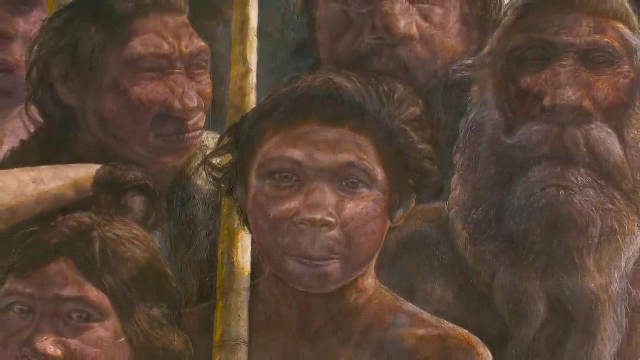 using this method, alongside the factoring in of several long bones, such as tibias and femurs, from african and european specimens, scientists have suggested that, on average, a male homo heidelbergensis individual was between 5 foot 7 and 5 foot 10 in height, whereas females were between 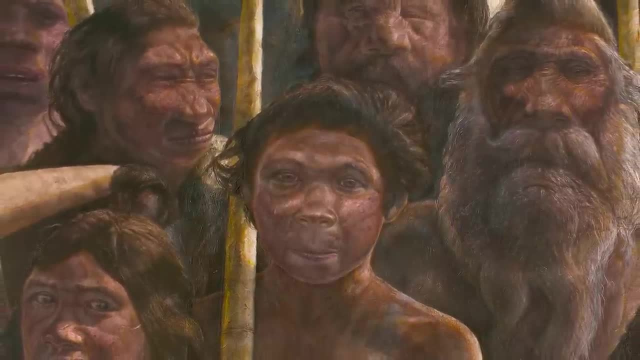 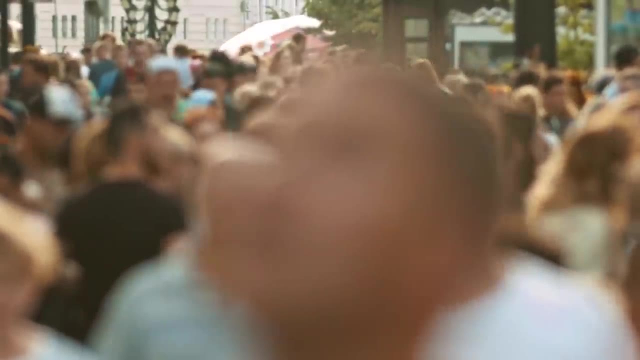 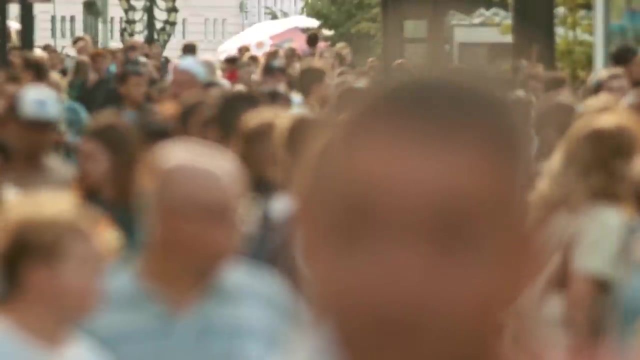 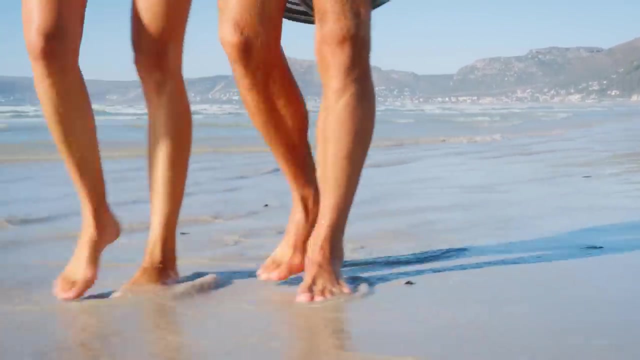 5 foot 2 and 5 foot 7 on average. although slightly shorter than modern humans, this was a significant increase from the australopithecines and early members of the homo genus from the early to middle pleistocene. these later species were evolving longer legs to help them cover greater distances. 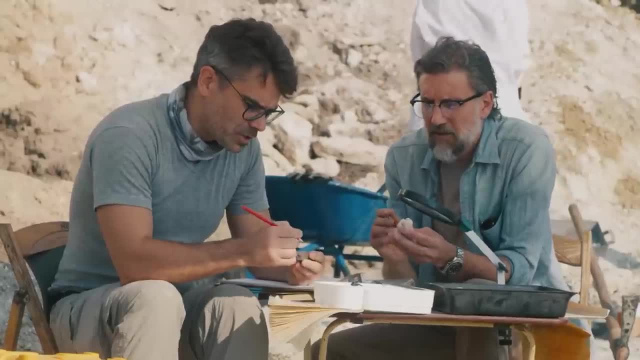 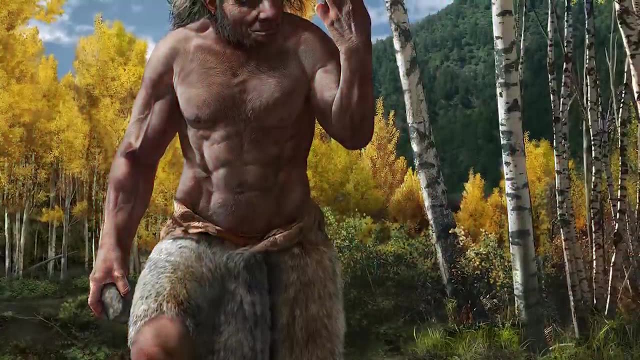 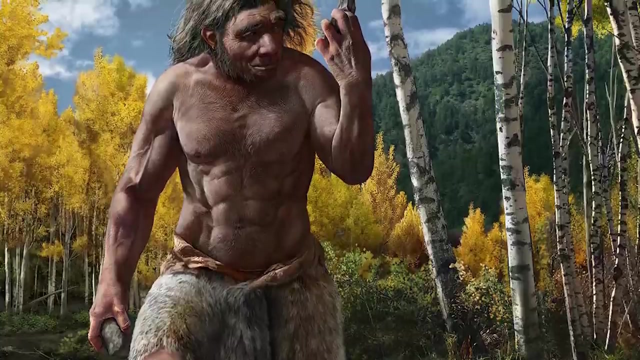 which can be seen firsthand inbuilt in the massive range of similar fossils across africa and eurasia. later species of humans to exist throughout the pleistocene tended to branch off into two slightly varying body plans. more common was the stocky, more barrel-shaped body. 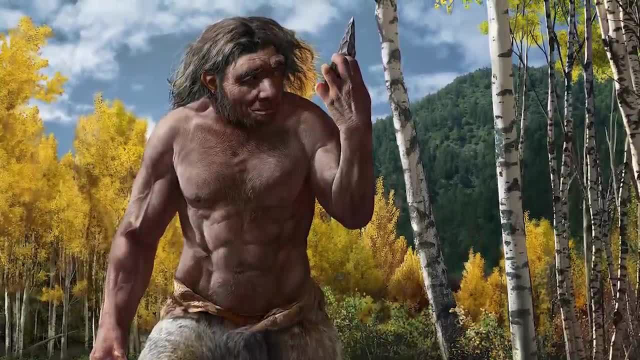 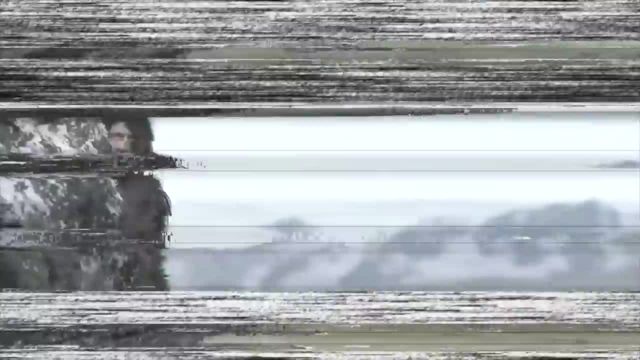 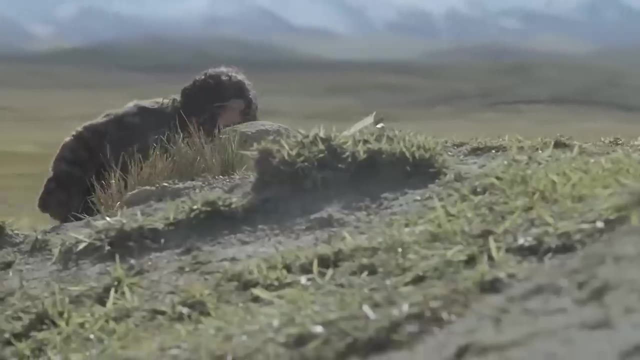 akin to that of a neanderthal or denisovan, a well-adapted body style for the harsh northern climates of eurasia. also found in archaic humans was the more homo sapiens-like form, more narrow-chested and slender than other species. 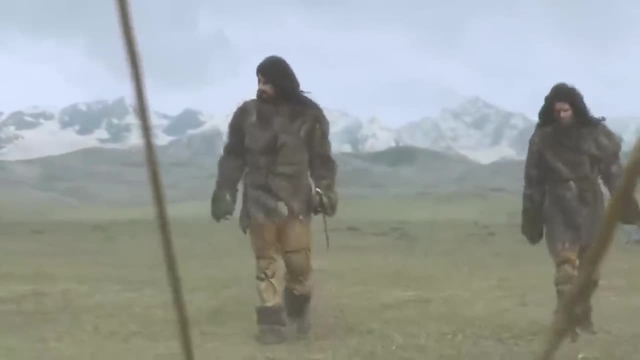 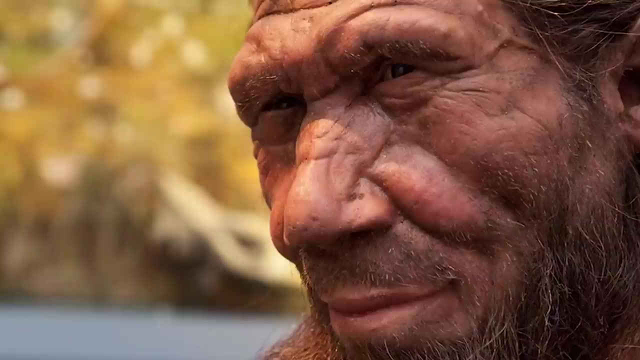 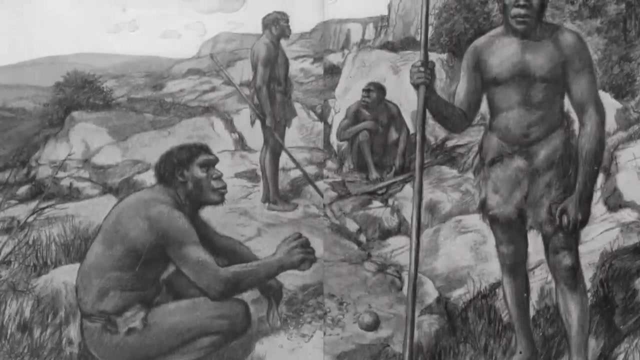 it is thought that, while these middle pleistocene humans were increasing in height, they still tended to adhere to the body plan that would later become synonymous with the neanderthals. homo heidelbergensis therefore possessed a bulky, stocky body plan with a broad pelvis and thick leg. 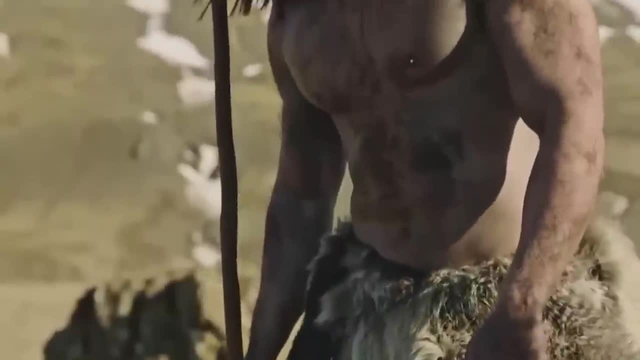 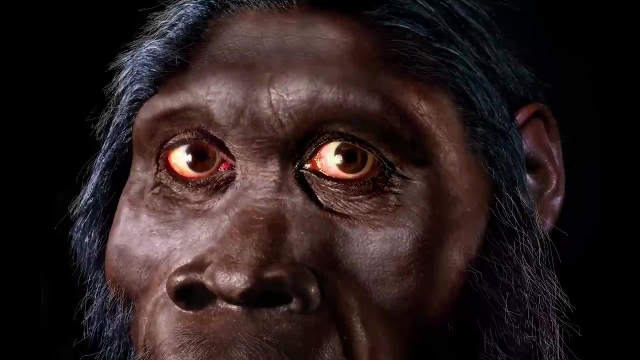 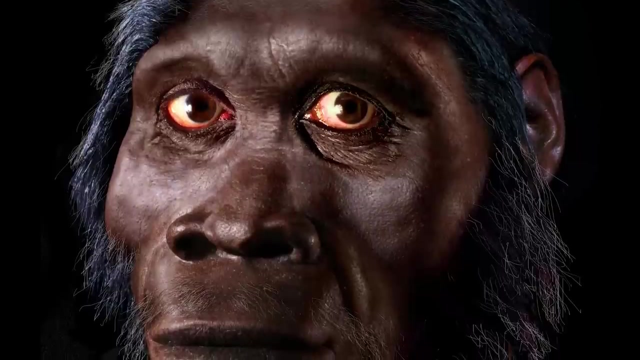 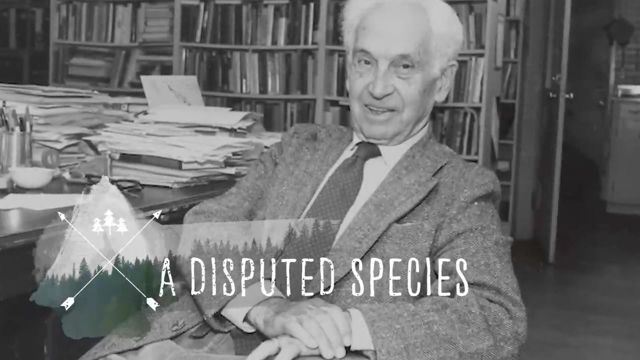 bones. this was likely an adaptation to help this species adapt to cooler climates in the north of eurasia, something that older species such as homo habilis and homo erectus, known for their affinity with warmer climates, lacked. the controversy began in the 1950s with the anthropologist ernst meyer. 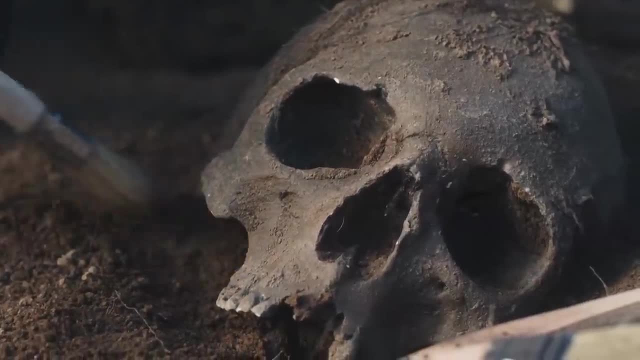 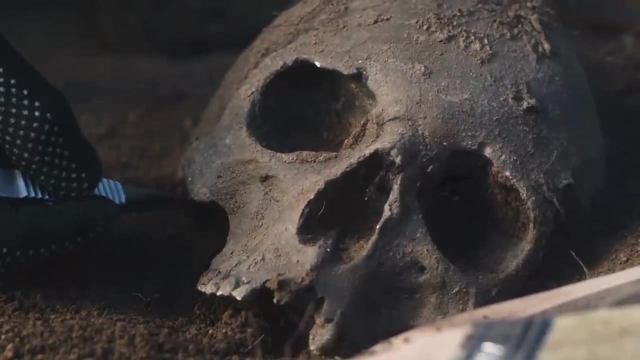 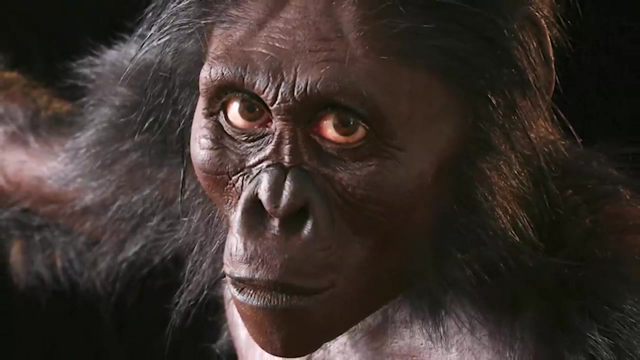 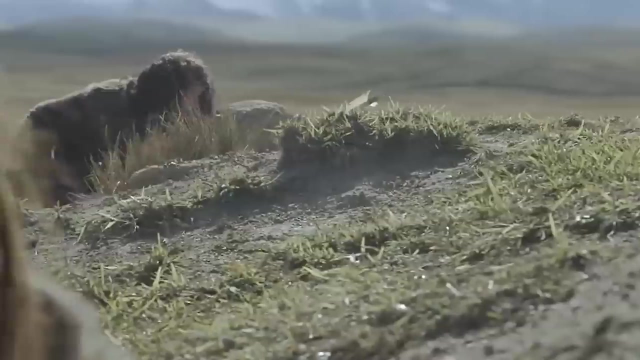 noting the extreme diversity of the number of species of archaic human popping up throughout the course of the middle pleistocene, he decided to recognize only three of them: australopithecines, defined by homo transvalensis, archaic humans defined by homo erectus, and modern humans and neanderthals, defined by homo sapiens. 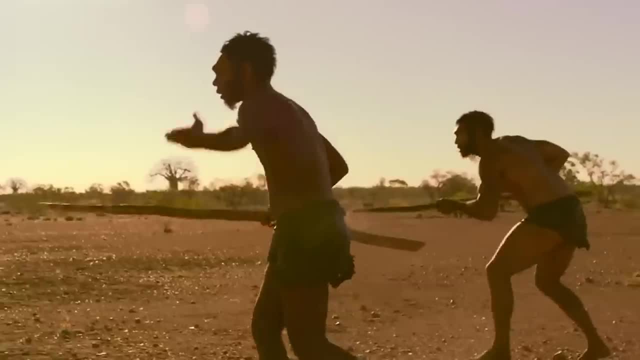 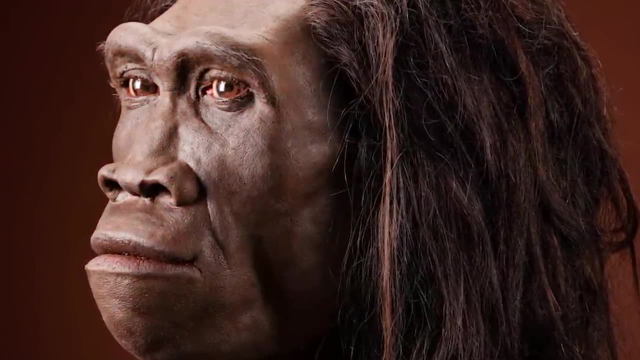 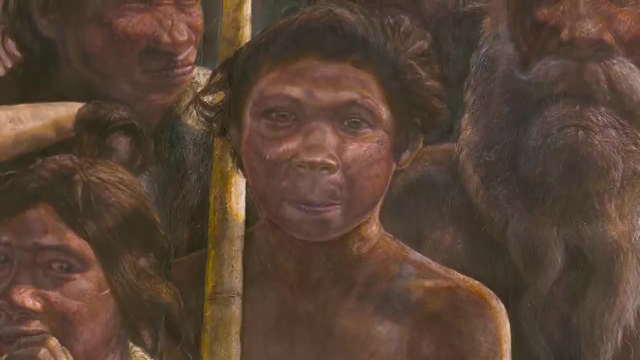 every known species of human, from the last australopithecine to the evolution of our own species, would be lumped into the homo erectus bracket, with a view to making them all obsolete. this included homo heidelbergensis, whose name would nearly fade into obscurity over the coming. 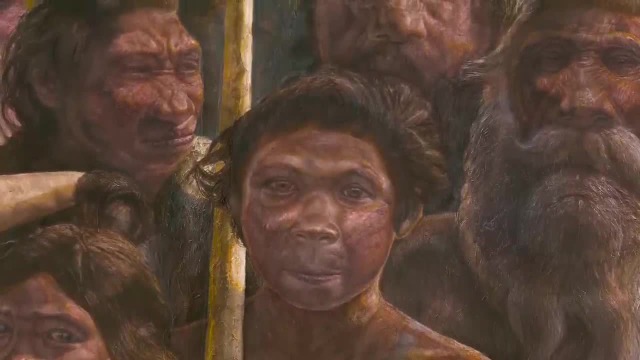 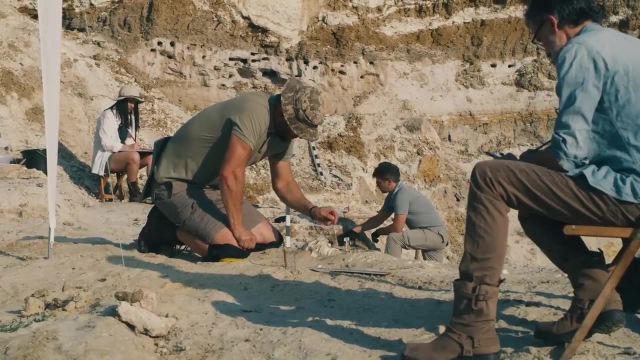 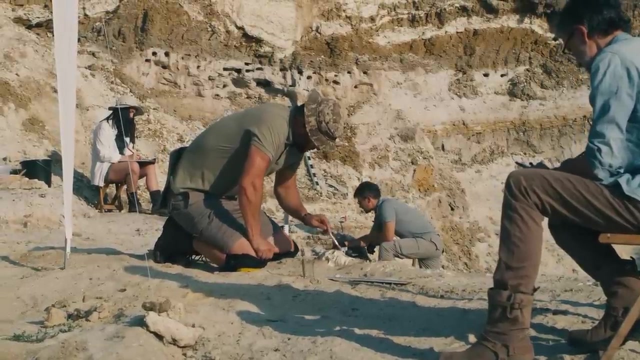 decades as meyer's take on ancient humans impacted the way we think about them today. meyer's claims are disputed. many of the species assigned to the homo erectus species by him in the 1950s have in recent years been noted for their differences and diversity, and many 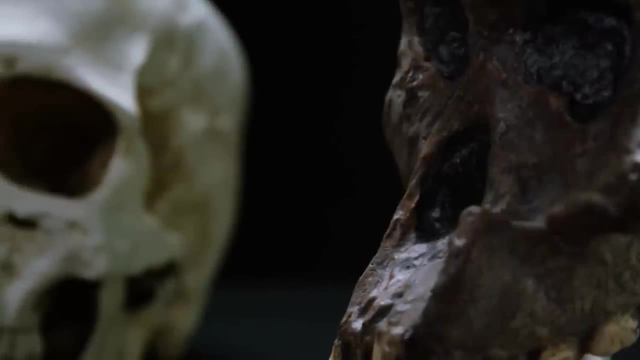 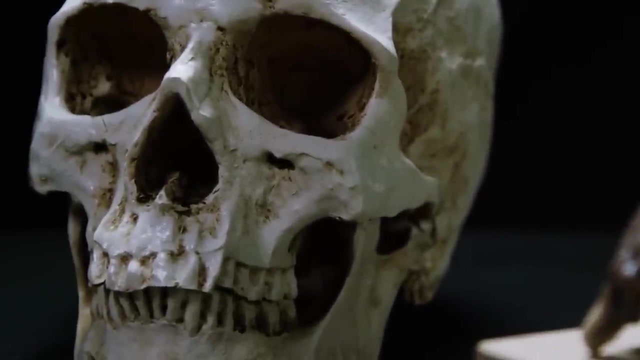 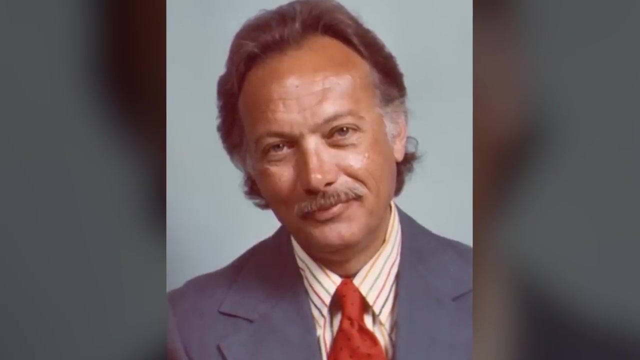 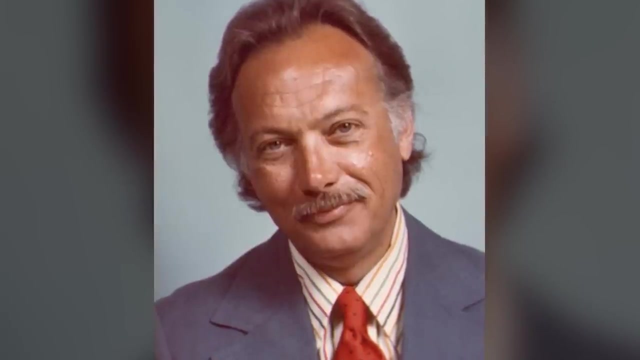 paleontologists, anthropologists and archaeologists are quick to determine them as separate valid species in their own rights. francis clark howell, an american anthropologist, was the first to lead the charge on opposing meyer's views, alongside the british chris stringer. they noted the similarities between several. 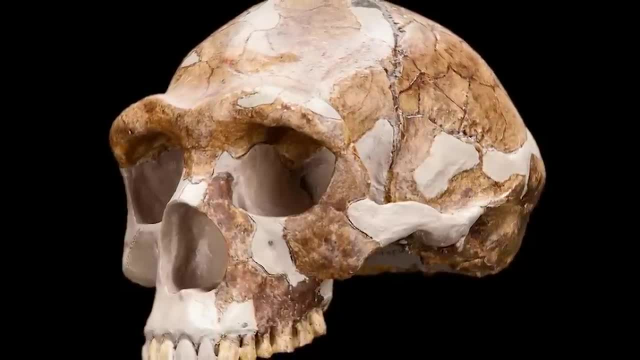 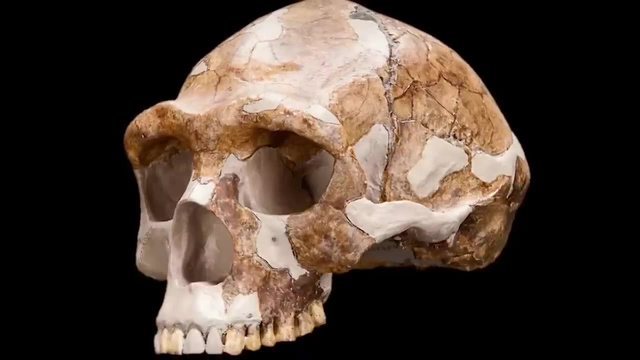 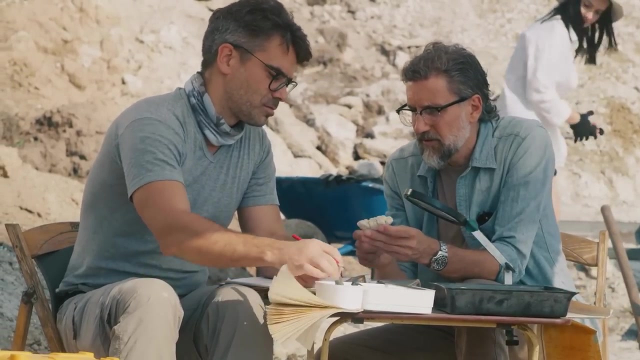 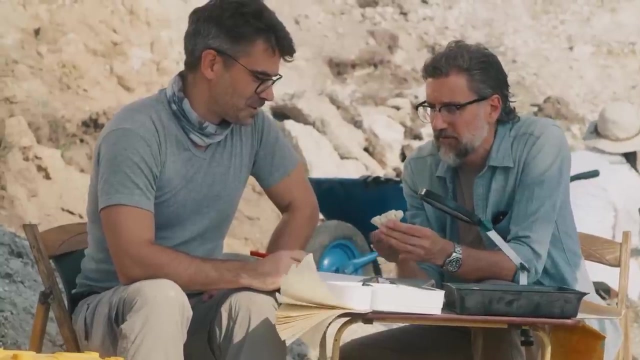 specimens of species that were previously assigned to homo erectus to those of our own species, opting to reassign them to homo sapiens. cracks started to show in meyer's original theory, and stringer suggested that homo heidelbergensis, amongst a few other species snubbed by meyer, should be reintroduced to the genus as their own distinct species. 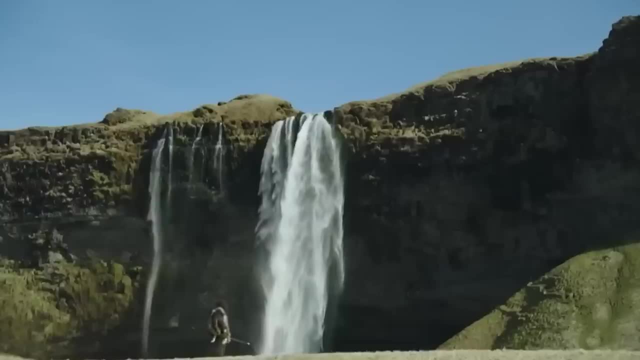 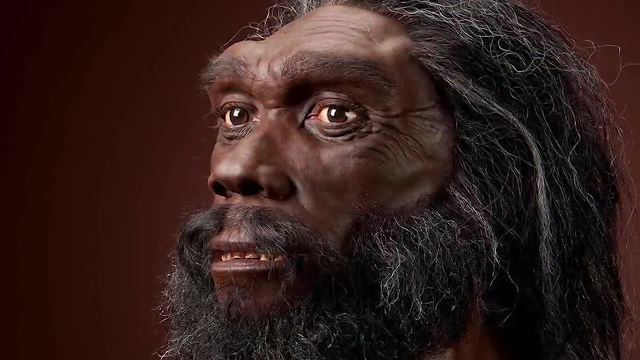 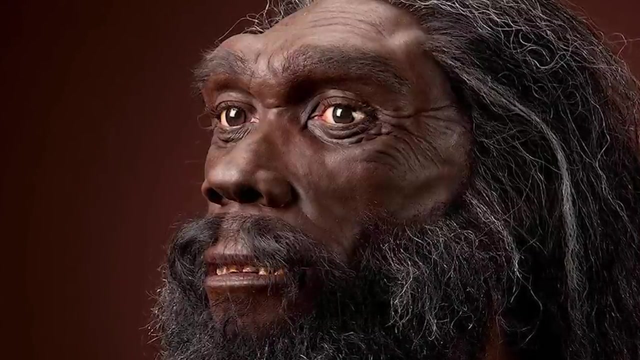 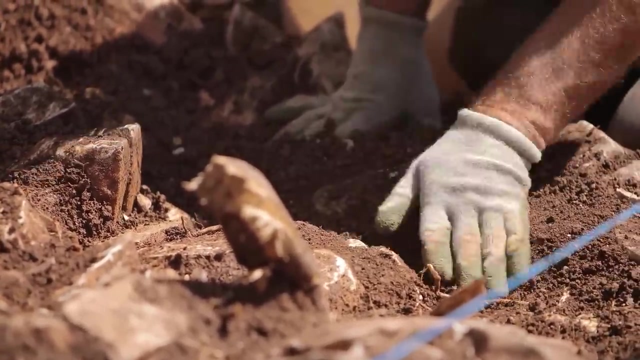 to highlight the differences between them and the specimens newly assigned to homo sapiens. stringer did a lot of work to help homo heidelbergensis become a widely used and recognized species of archaic human. once more, further studies on north african and european human fossils have led to many specimens across. 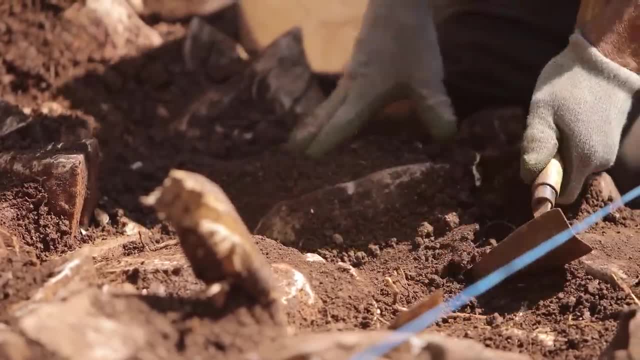 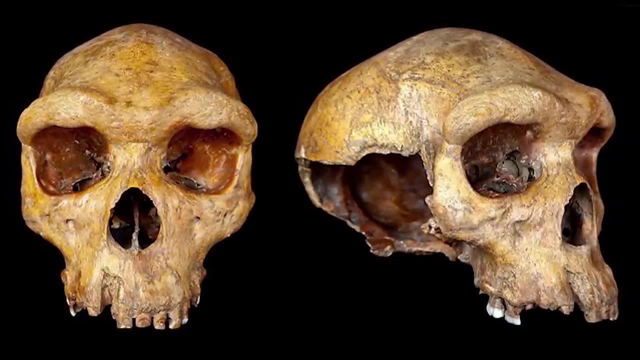 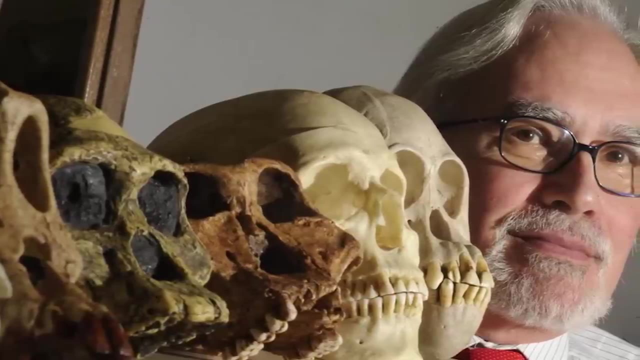 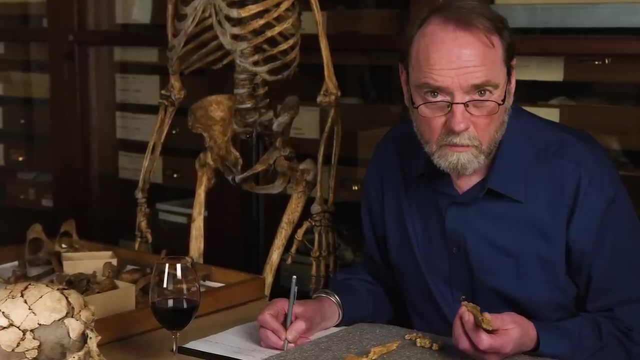 these areas being assigned to homo heidelbergensis, and most remains from these areas dating around 600 000 to 300 000 years ago are typically assigned to this species. later in 2010, american anthropologist jeffrey h schwartz, along with paleoanthropologist ian tattersall, took this a step further, suggesting that all 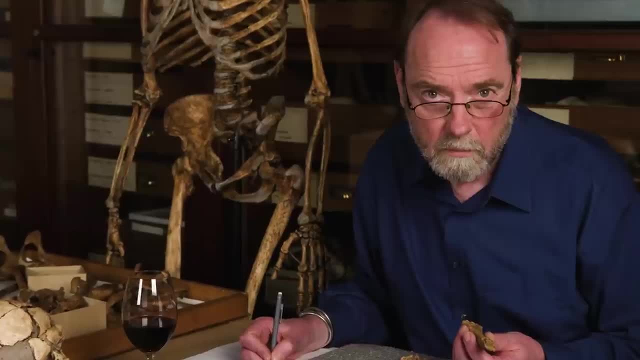 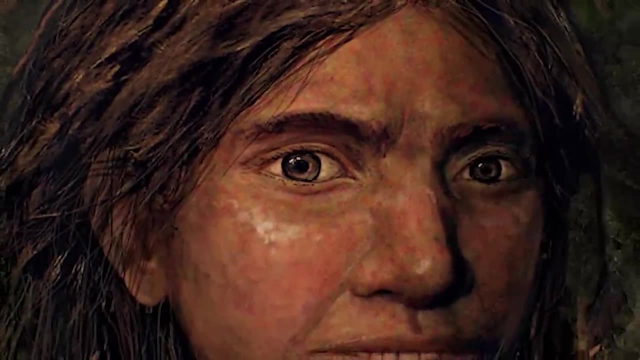 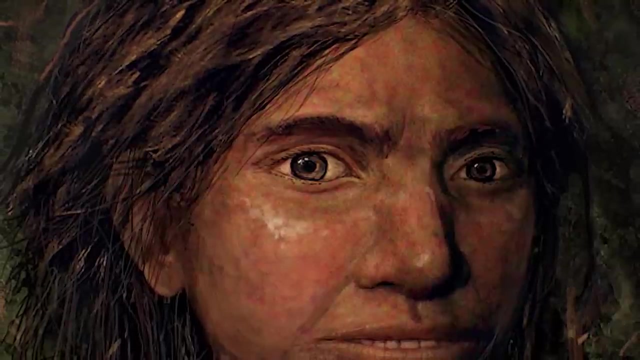 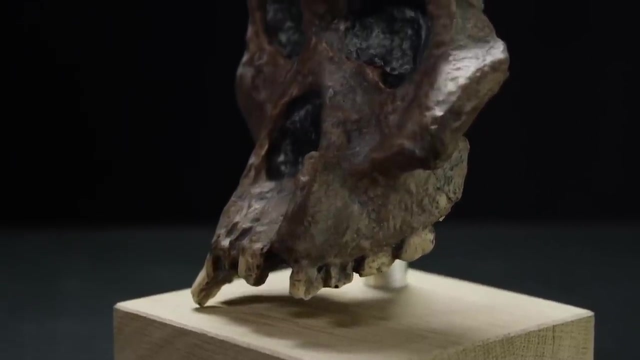 specimens from middle pleistocene europe and asia should be classified as homo heidelbergensis. upon the recognition of the denisovans, an archaic species of pleistocene human we have previously covered on this channel, this theory became less and less popular, with a lot of asian specimens being presumed to be denisovans. 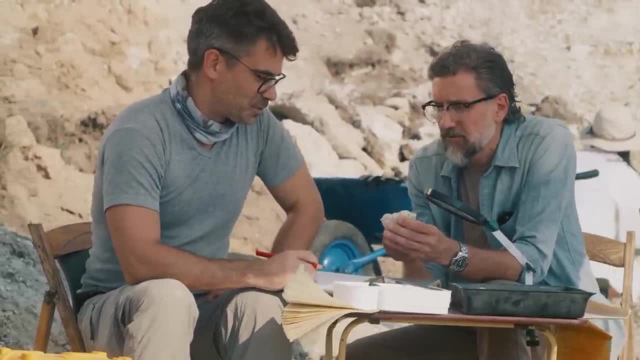 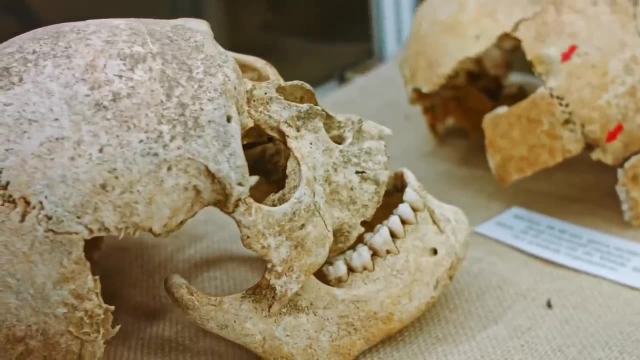 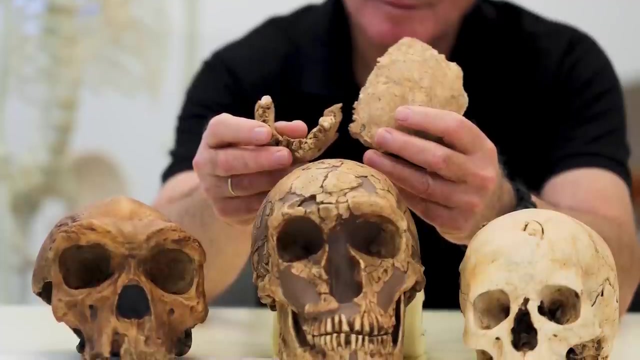 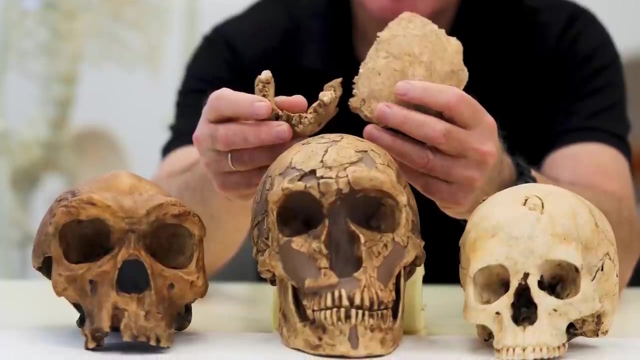 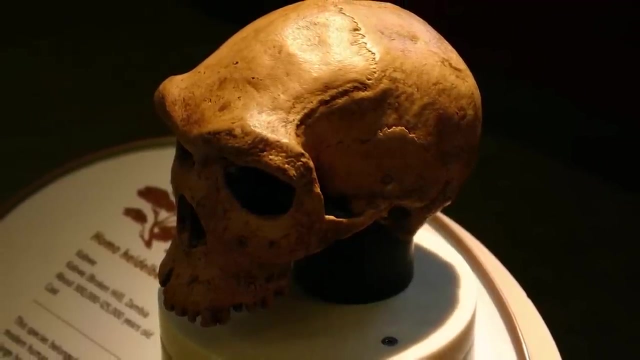 all of these factors and more when other species are brought into the mix. factor towards the middle pleistocene epochs- infamous nickname among anthropologists and archaeologists: the muddle in the middle. it is very difficult to discern at this point which species, species or specimens of known species, alongside figuring out which species evolved from and 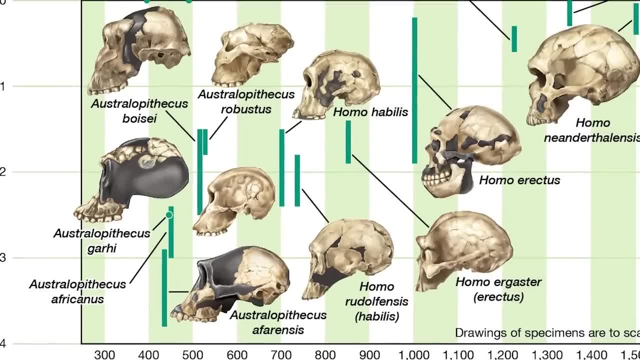 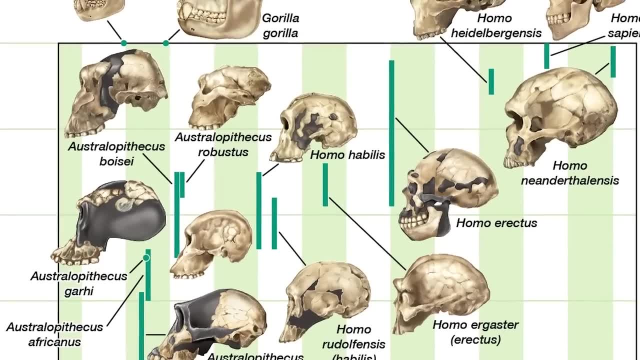 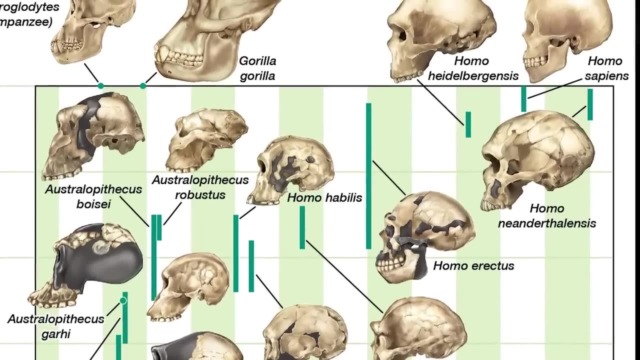 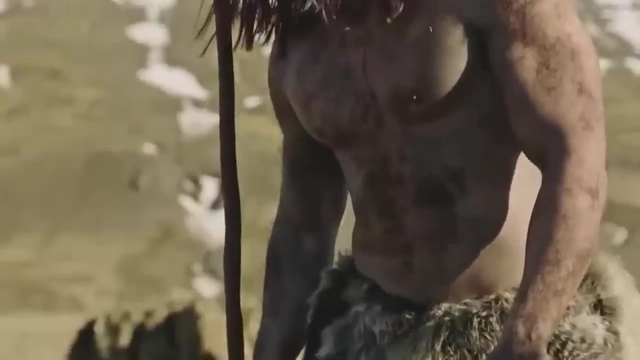 possibly into which. This is due to the large number of recognized species from this period in time, and Homo heidelbergensis has fallen victim to much debate as a result over the years since its discovery. Due to similarities and proximity in terms of time to Homo sapiens, some researchers 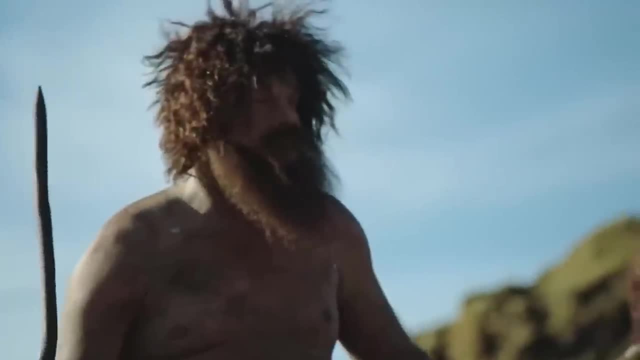 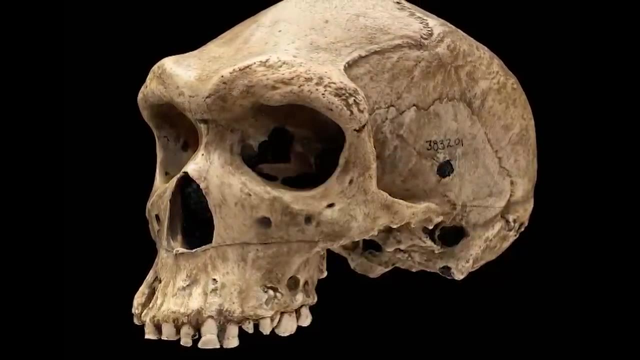 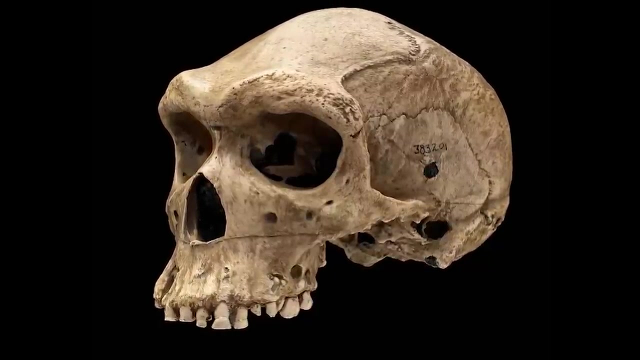 have determined that Homo heidelbergensis should be placed within our very own species and that the known fossils of Homo heidelbergensis represent a subspecies of Homo sapiens living in the earlier stages of the Pleistocene. William Strauss, an anthropologist who studied the original mandible, 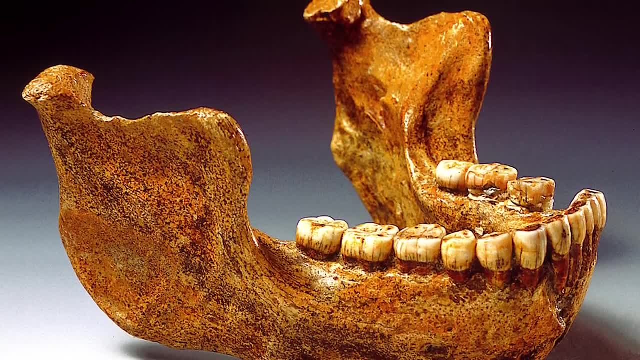 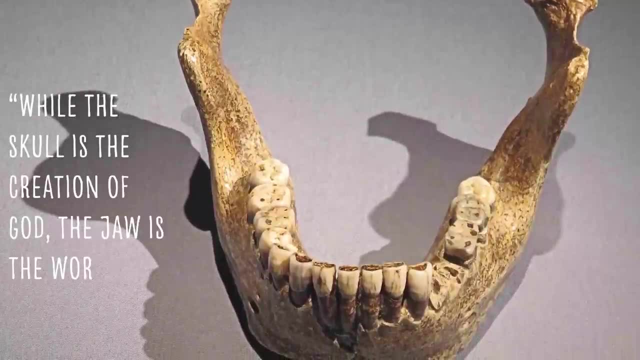 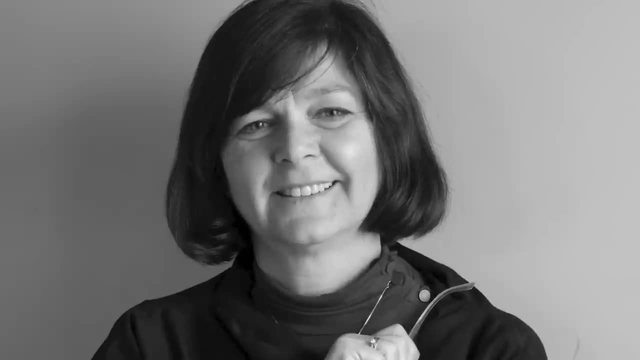 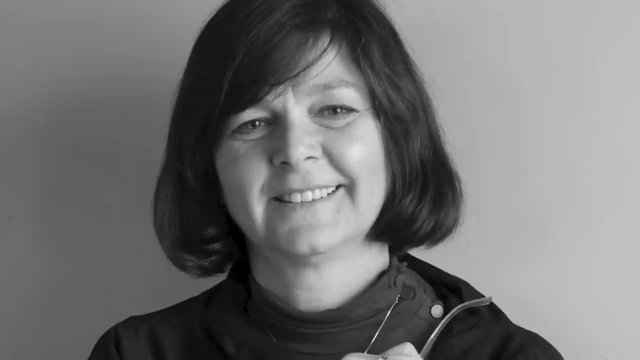 discovered in 1907 in Mawa. Germany has previously said about the find: While the skull is the creation of God, the jaw is the work of the devil. in reference to the confusion it caused, Marianna Raksanich, a Canadian anthropologist, is the most recent researcher to weigh in on Homo heidelbergensis. 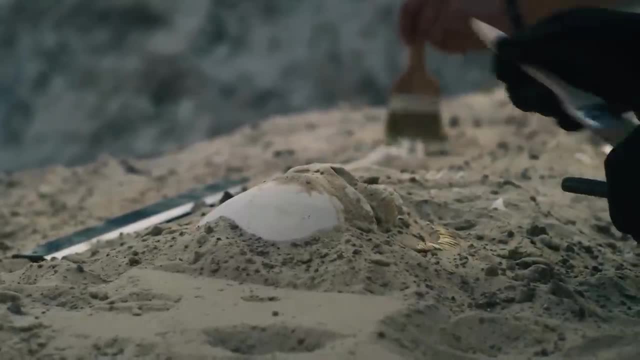 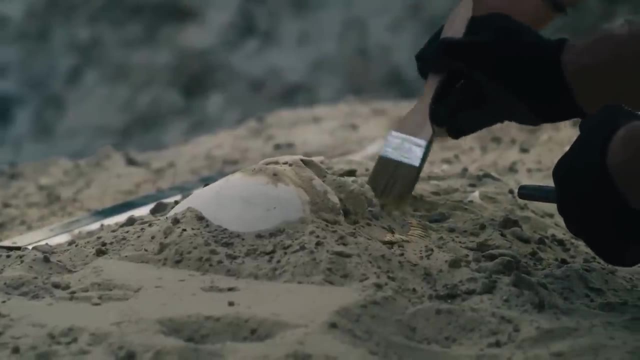 Marianna and colleagues have prepared a list of the most recent discoveries of Homo heidelbergensis. Marianna Raksanich, a Canadian anthropologist, is the most recent researcher to weigh in on Homo heidelbergensis. Marianna Raksanich, a Canadian anthropologist, is the most recent researcher to weigh in on Homo heidelbergensis. 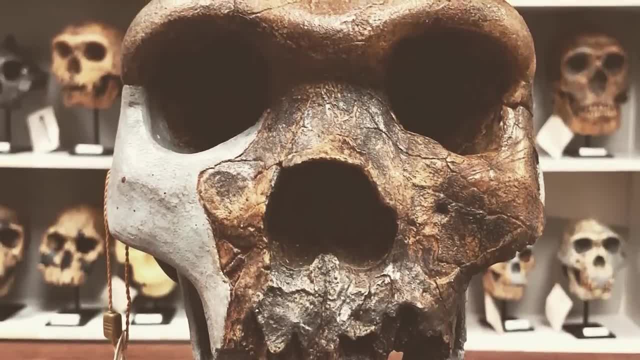 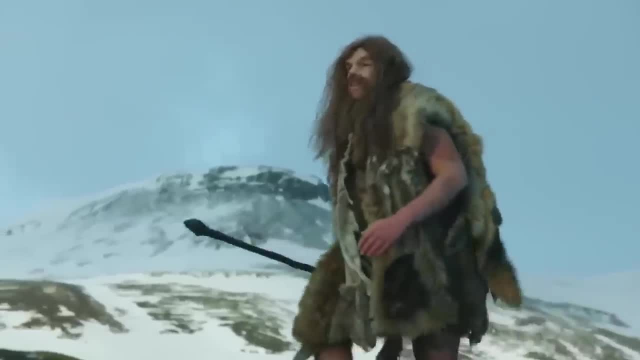 My own Dalai Lama'sacă team was very closes to the fact that the entire period of the evolution of age debering to the creation of spores was just an illustration of medical pr Dude Moriba's episode about the occurrences of disease in the Maori territory. 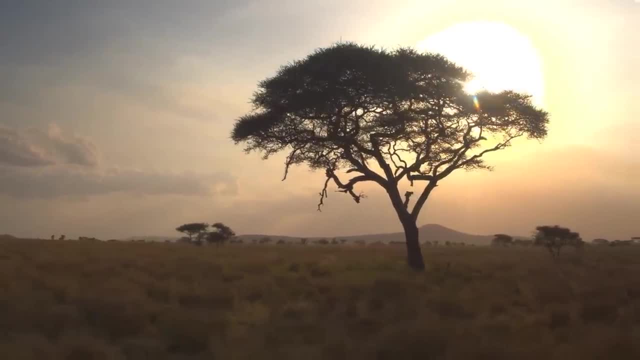 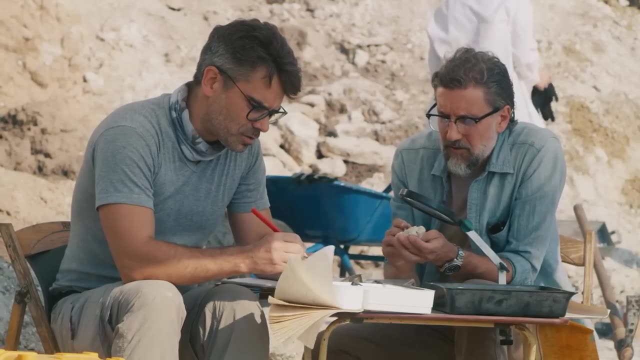 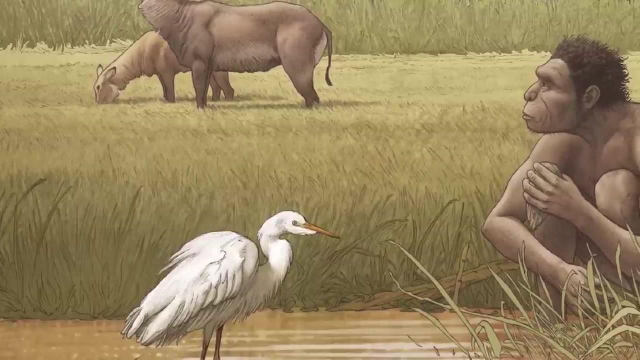 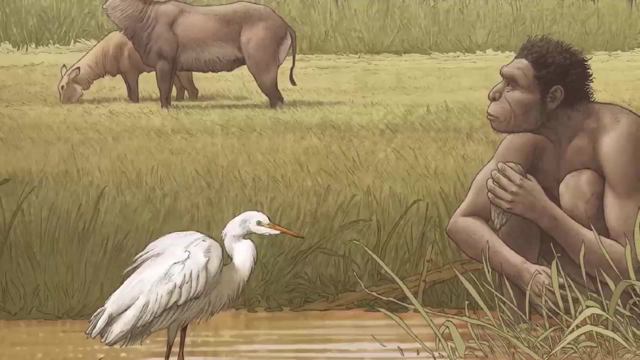 Therefore Bre exclusively, is the only victim catch-all term for African specimens, Homo bodoensis. The team also came up with an explanation for all the confusion. Potentially Homo bodoensis and what was once considered to be Homo heidelbergensis periodically migrated across Africa and Eurasia between glacial cycles. 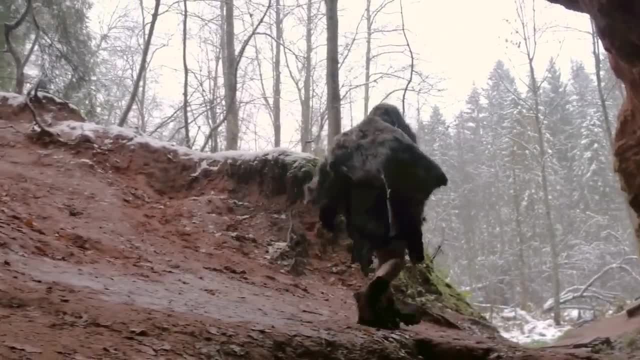 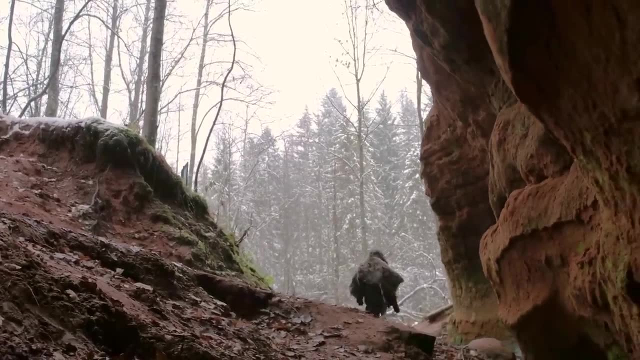 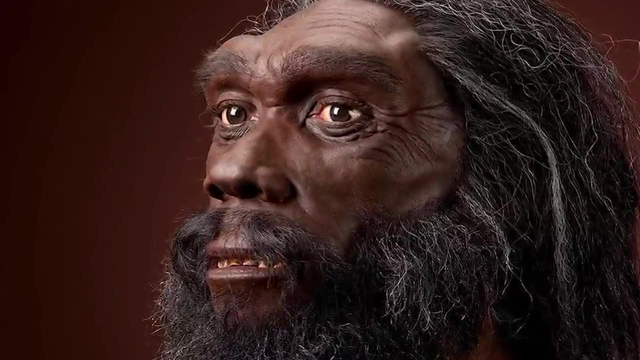 On the way they would have come into contact with indigenous populations of archaic humans, where they would likely interbreed. So where does Homo heidelbergensis stand today? Chris Stringer, who has worked extensively on Homo heidelbergensis along with other researchers, 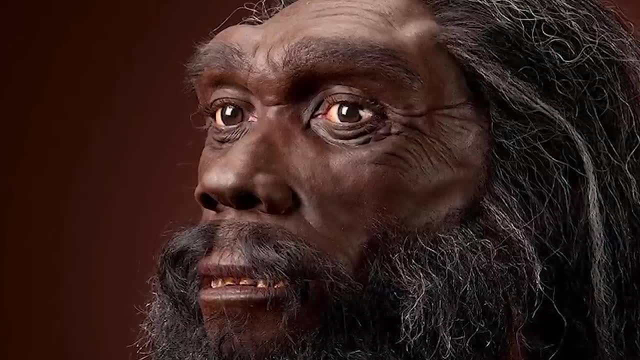 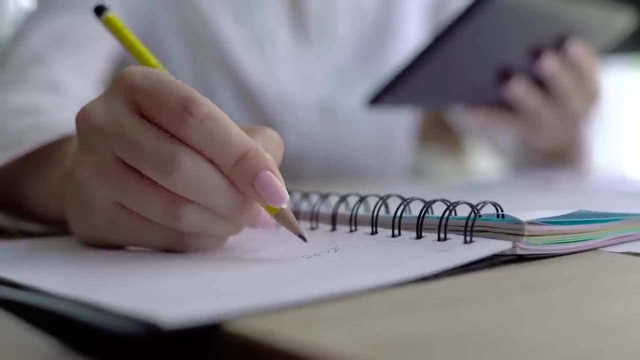 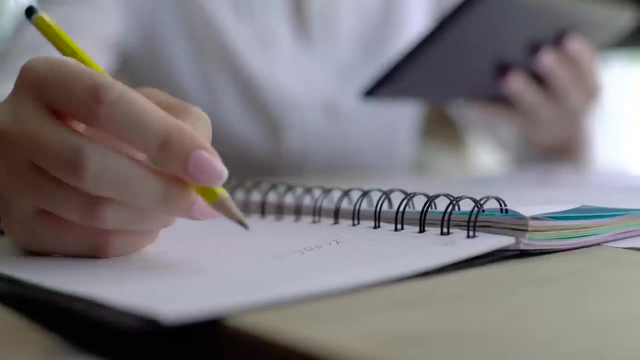 unsurprisingly reject the claims made by Roksanich and the team, as they felt the research did little to help us resolve the story of Homo heidelbergensis. Through changing the names of species at will, they also broke the rules of scientific binomial. 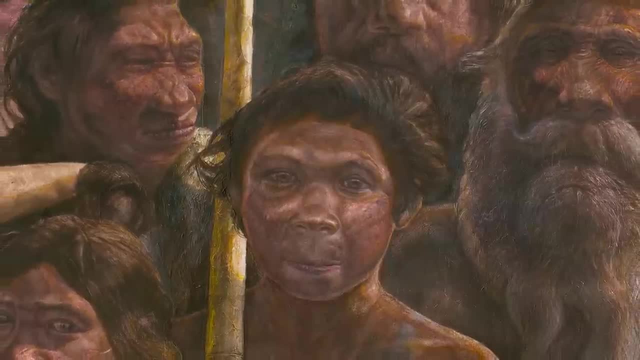 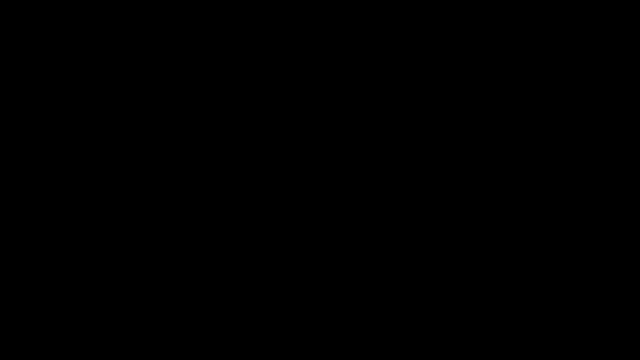 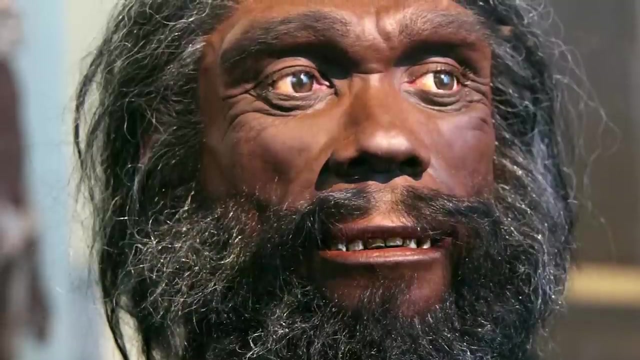 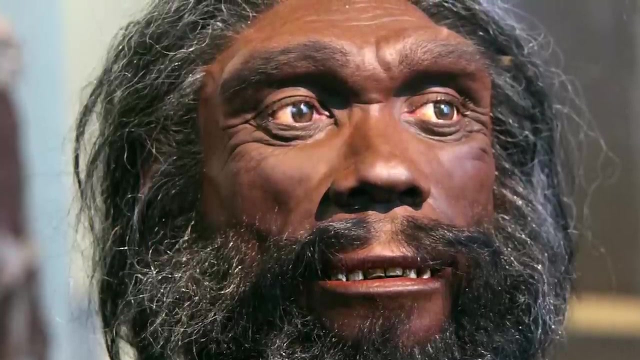 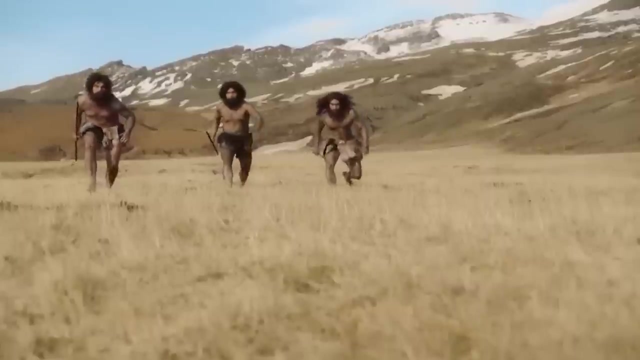 naming As it stands, Homo heidelbergensis, is valid, but for how long? Homo heidelbergensis, it has been determined, was one of the first humans to be more strictly carnivorous than other species that preceded it. These were omnivorous humans, but ones that had become highly skilled at filling the apex predator. 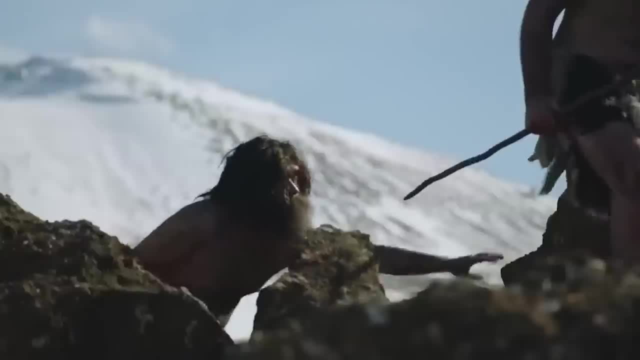 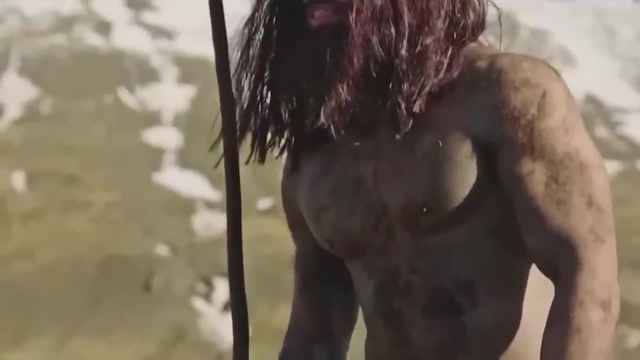 spot on the food chain. A better understanding of weaponry and hunting techniques allowed these early people to hunt big game, Actively stalking and pursuing it across the steppes. they were able to hunt big game. They were able to hunt big game. They were able to hunt. 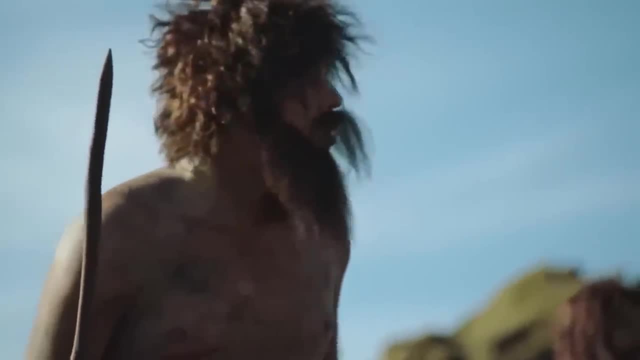 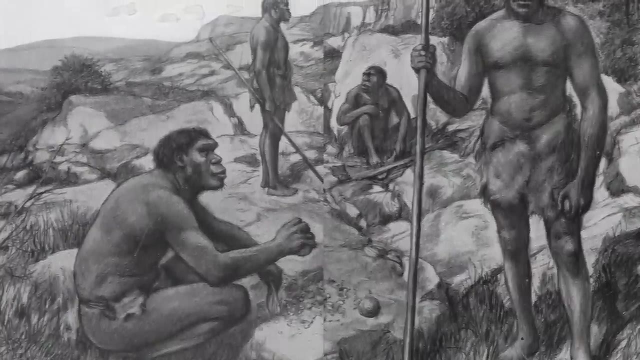 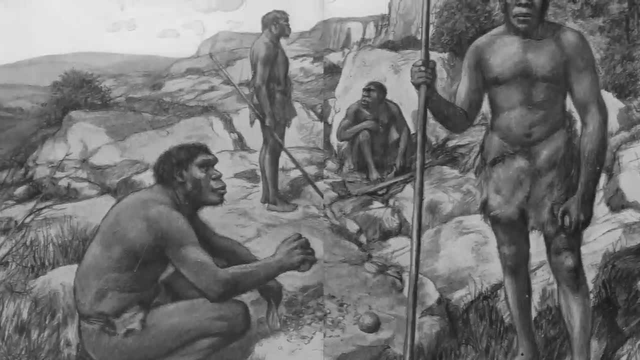 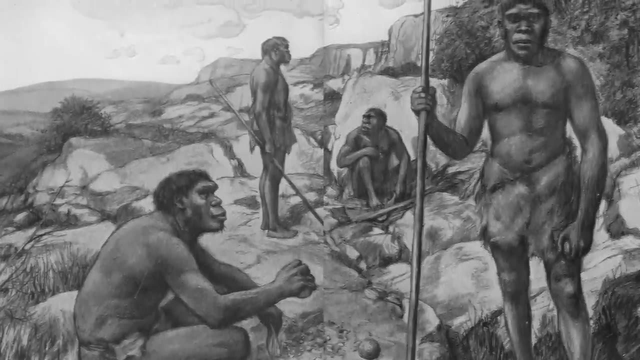 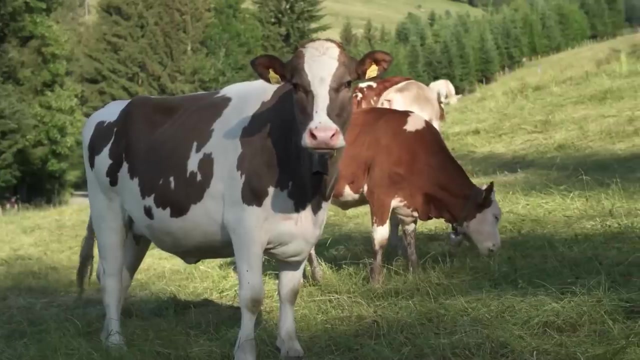 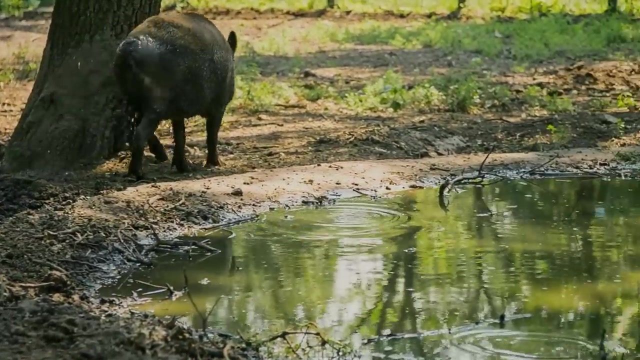 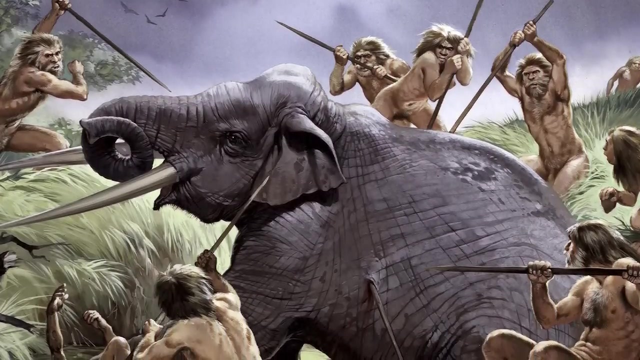 and they are determined to hunt, even if only for the sake of itsası Some. not far from this. some pieces could have existed of great size- horses and boars- But on occasion, possibly, when food was more scarce or when the opportunity presented itself, these people would take prey as large as elephants. 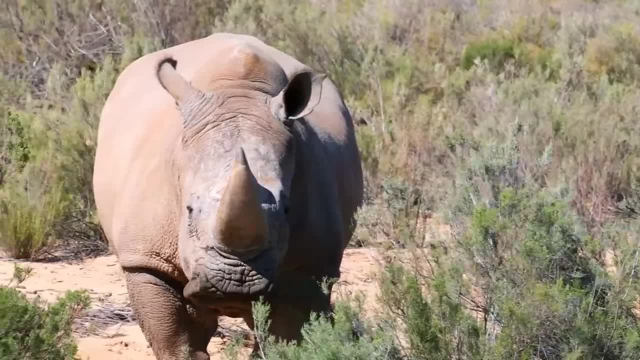 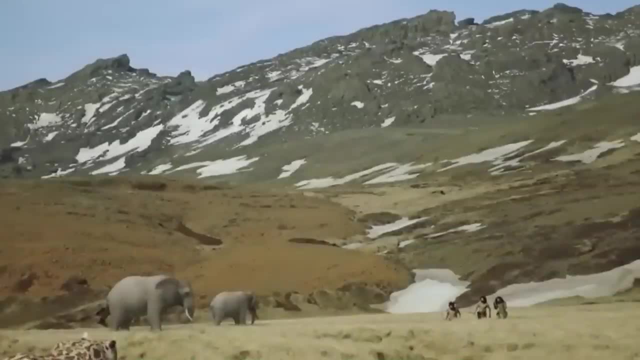 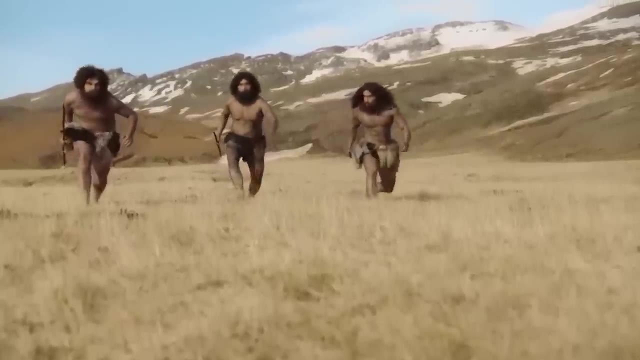 Archaic species of elephant, as well as rhinoceroses, would have been challenging yet possible kills for Homo heidelbergensis, whose communities would have efficiently worked together on elaborate plans to bring down these animals As archaic humans. hunted meat: natural selection. 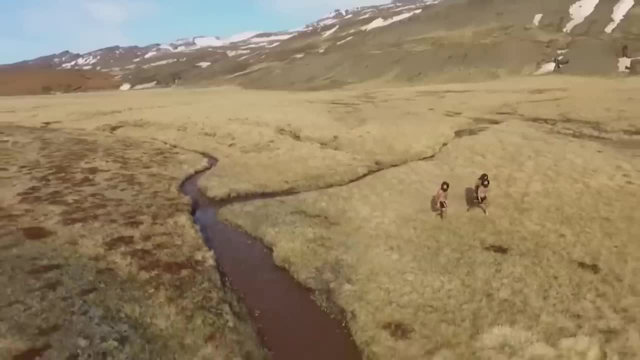 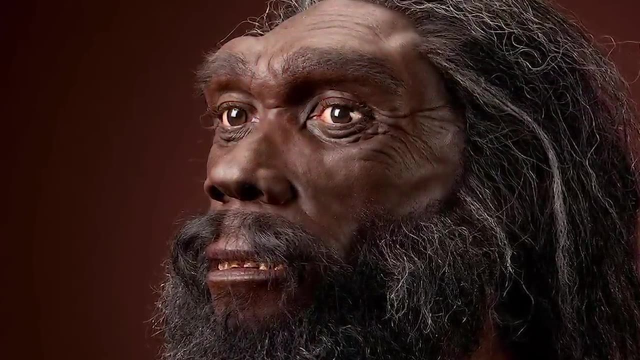 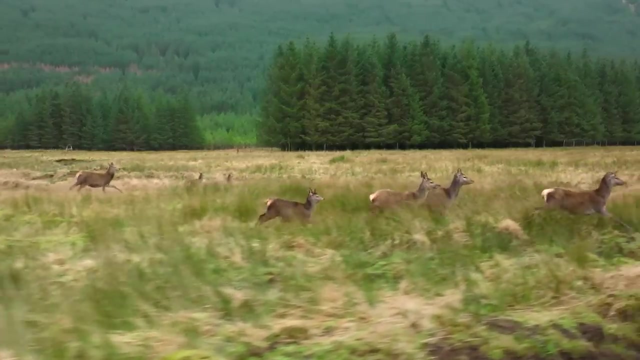 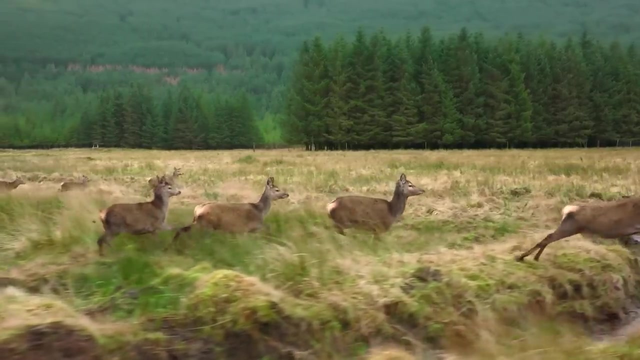 set to work in improving these people's abilities to hunt. Larger brains led to better hunting strategies, which led to the ability to hunt larger and more complicated prey. It is thought that when hunting Homo heidelbergensis, teams worked together to herd animal into environmental features that were difficult to escape Larger animals. 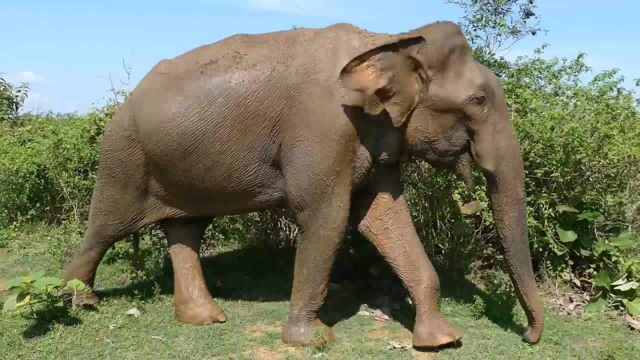 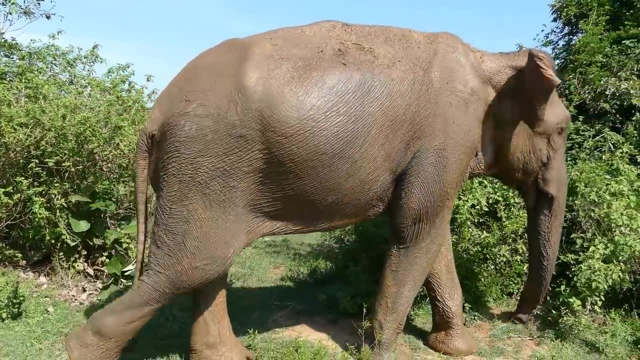 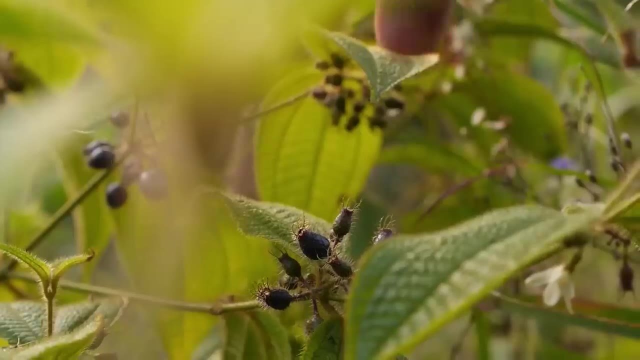 such as elephants, may have been chased into swamps or marshes before being circled and killed with sharp spears and points. Meat was not the only food source on the menu for Homo heidelbergensis, however, and communities of these humans are known to have. taken a wide range of berries and fruits from the Homo heidelbergensis family. The Homo heidelbergensis family is known to have been a great source of food for the Homo heidelbergensis family- and possibly even tree bark To counteract the threats of protein poisoning inflicted by a. 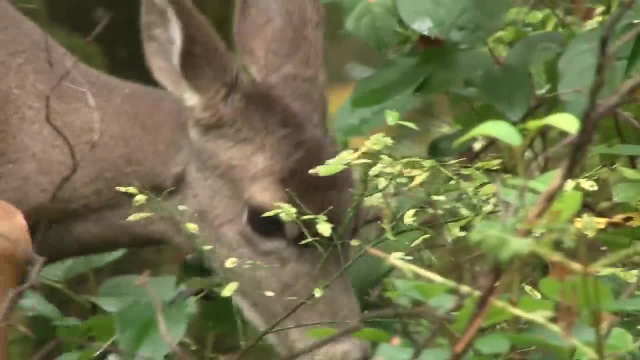 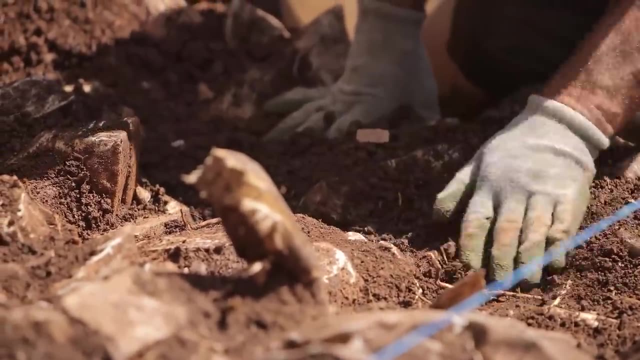 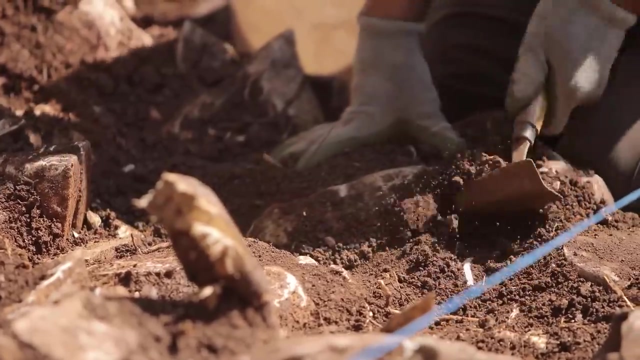 consumer of a diet with a very high meat content, a large deal of carbohydrates would need to be consumed. Plant matter does not fossilize as well as animal bones, and for the time being we cannot determine too much about the plant-based food intake of Homo heidelbergensis. 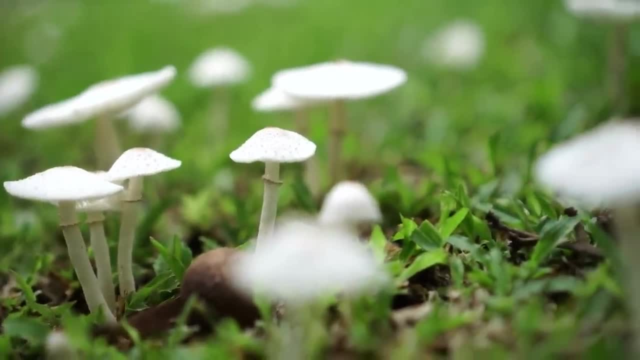 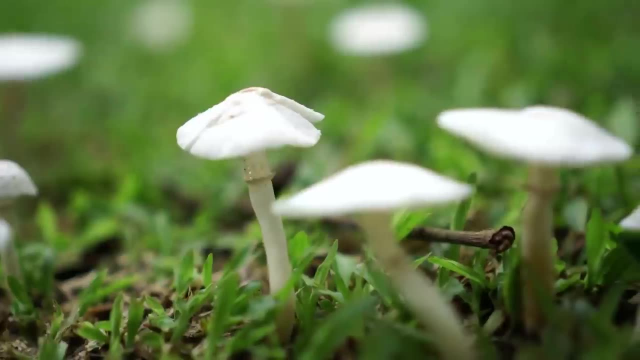 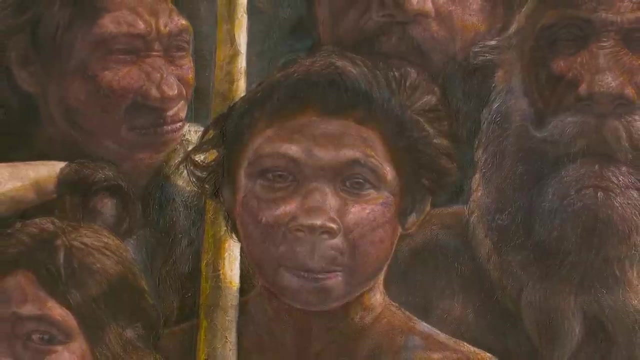 But it is known that the Schöningen site in Germany, associated with high-quality hominid vines, is home to over 200 plants that can be safely eaten uncooked or otherwise. Given that these plants were likely present at the same time, Homo heidelbergensis was present on the 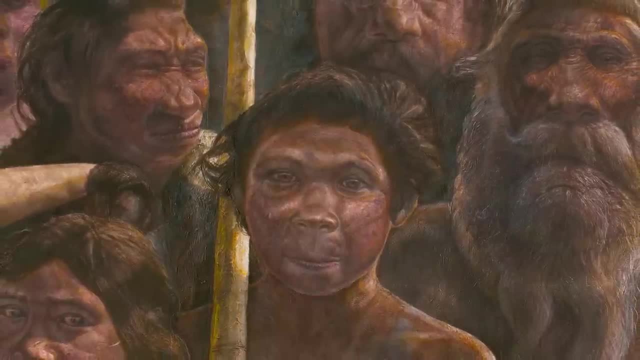 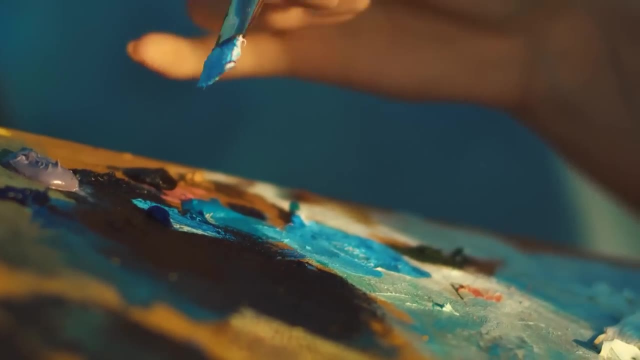 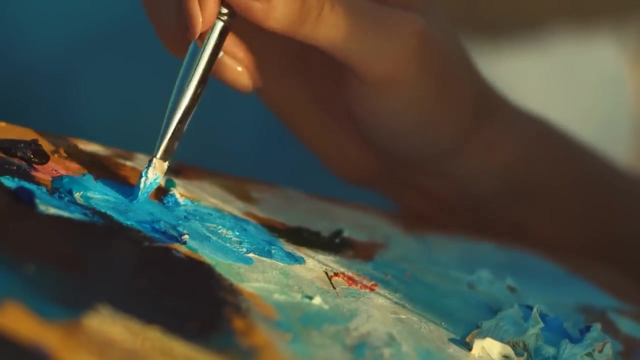 scene, it is safe to assume that many of them would have found their way into the diets of this species. It is in Homo heidelbergensis that we see some of the earliest evidence for what could be considered to be art. Engravings and carvings have been uncovered across the areas where Homo heidelbergensis 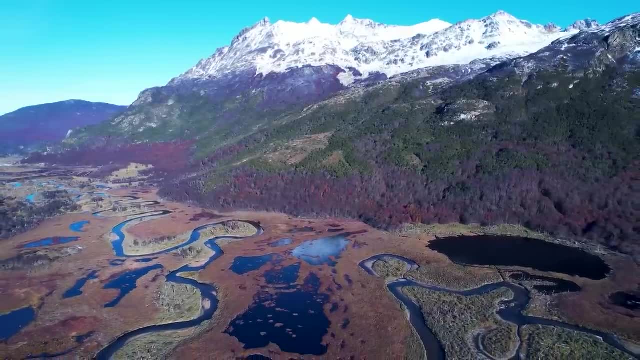 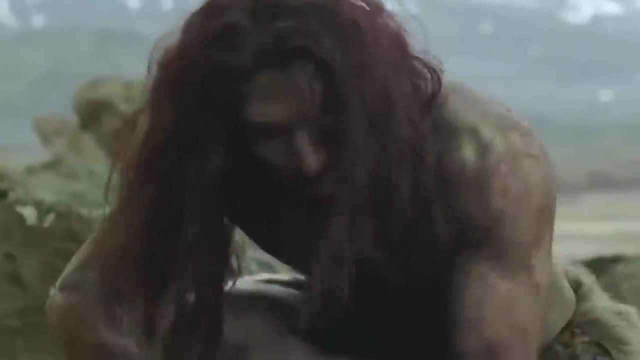 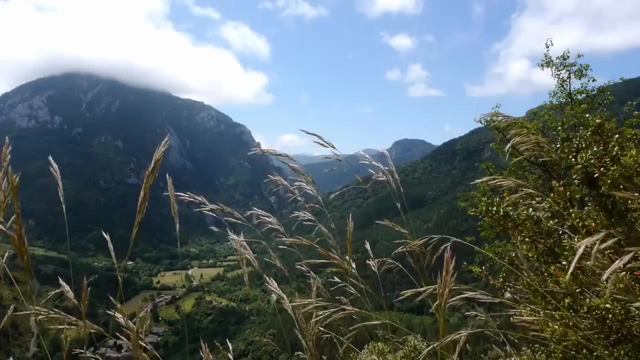 would have been living that bear no logical explanation other than a symbolic one, indicating that these people may have been carving simple patterns or lines into rocks for fun, Or to make a note of something. Such structures have been found across France and Germany. 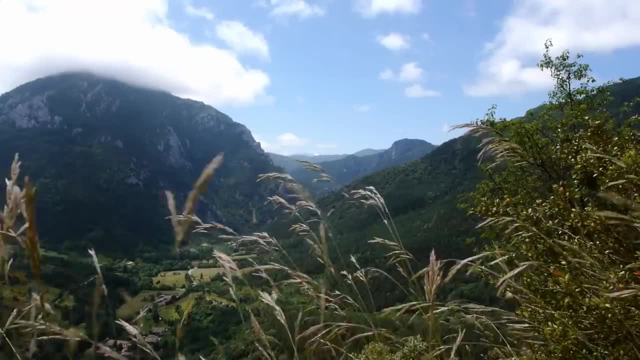 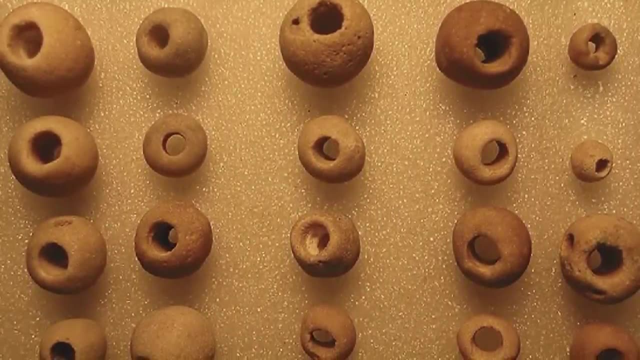 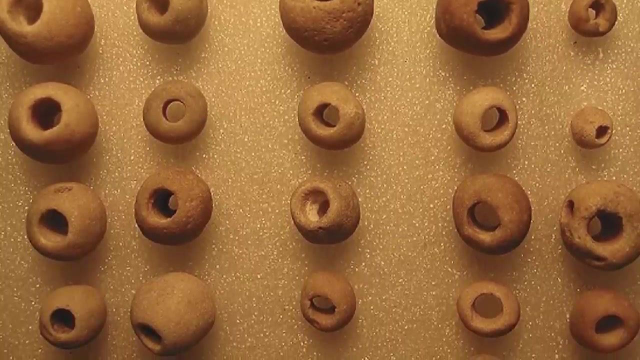 Potential jewelry has even been discovered from Europe in the form of perforated sponge fossils which may have been threaded together to form charms or beads on a necklace or bracelet. These structures appear to have been deliberately chosen due to their round form and shape. These structures appear to have been deliberately chosen due to their round form and shape. 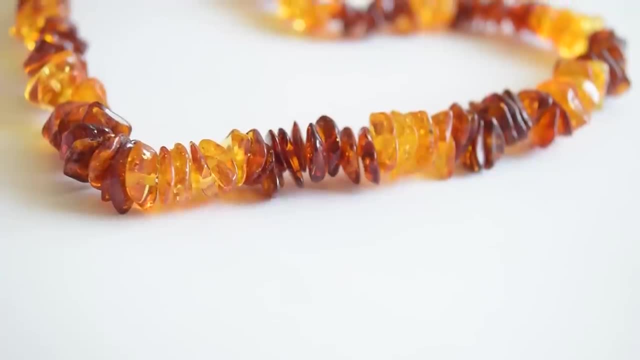 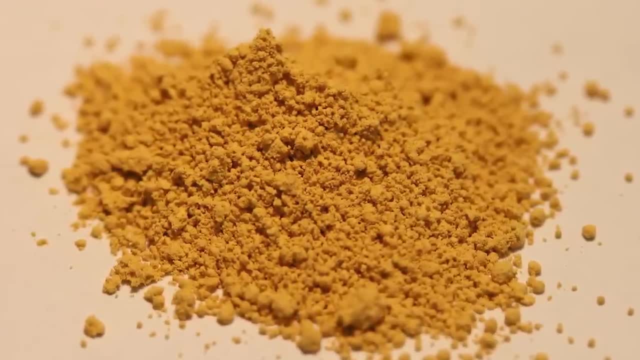 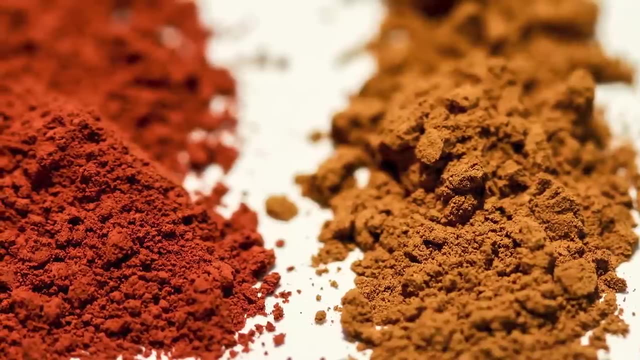 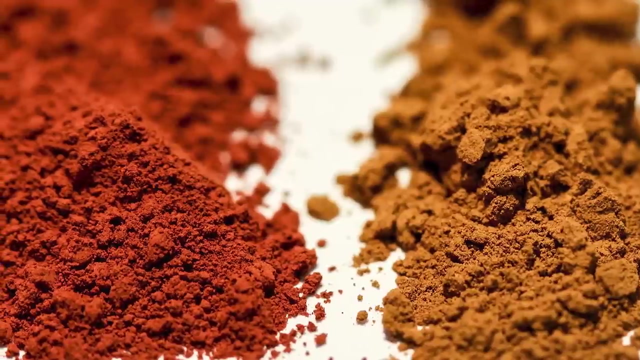 which were cut through to create a bead-like structure. We also know that many humans from this period in time were utilizing ochre to create a paint-like substance. Red ocher is particularly common, Scientists have suggested perhaps due to the fact that it cauvers with a similar colour to that of blood. 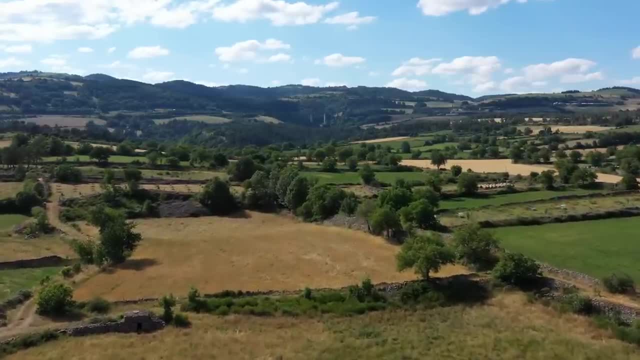 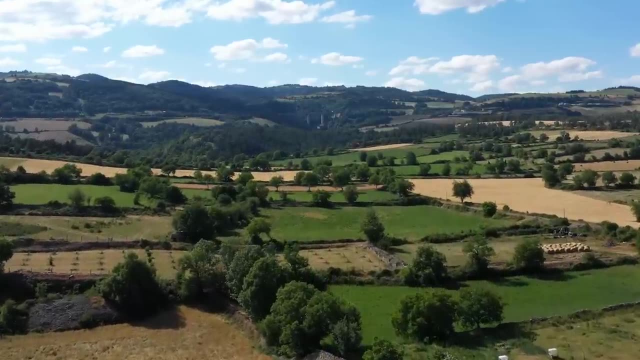 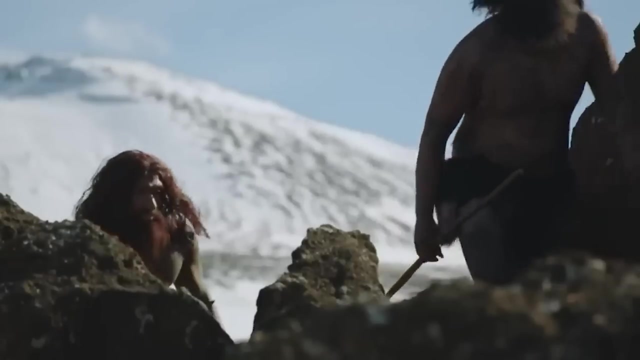 più Terra Armada site near France, over 70 pieces of ochre have been found that are thought to have been mixed to achieve different shades of reds, yellows, browns and oranges. This indicates that these people had a preference for the color they used to decorate their 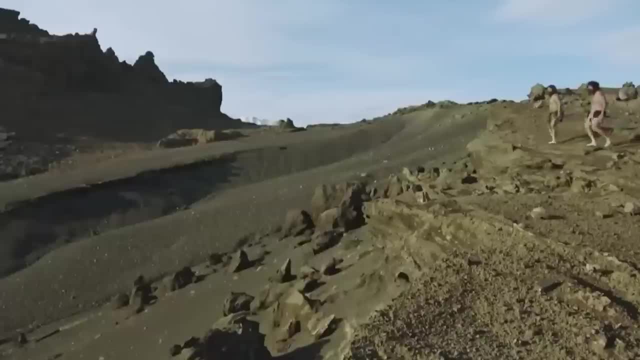 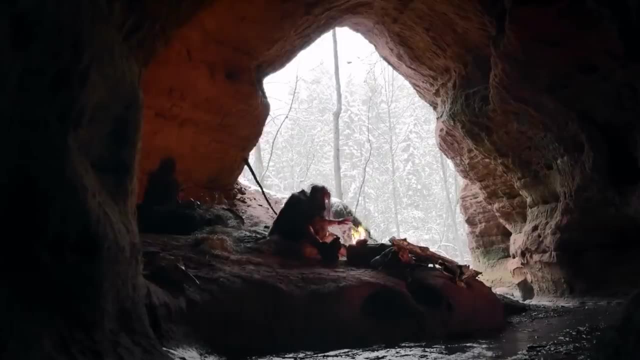 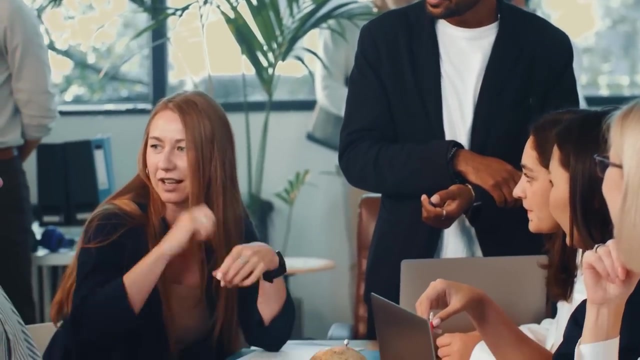 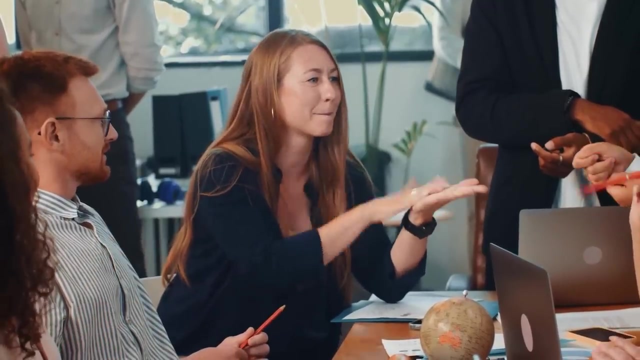 structures and potential artwork, meaning they had a basic understanding of creativity and design. One of the most intriguing questions surrounding ancient species of humans concerns their ability to speak and formulate a language. Could they do it, Or did they communicate more in a series of incoherent grunts and whoops? 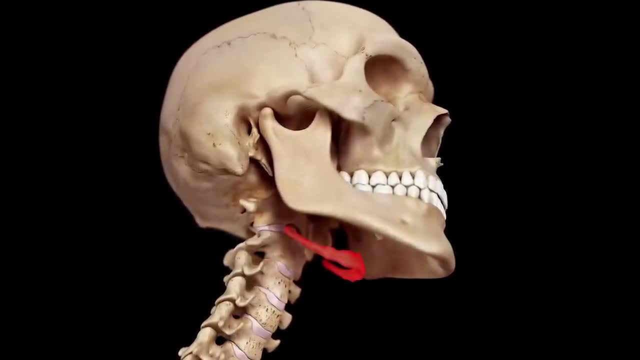 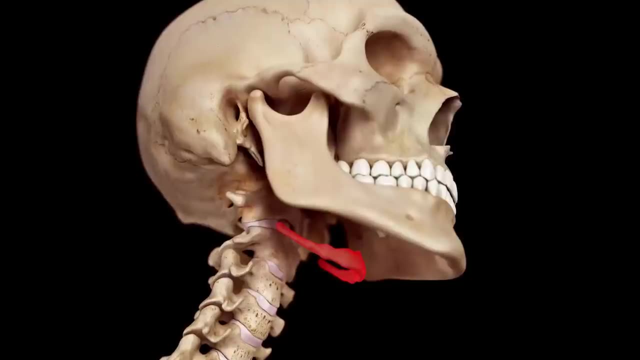 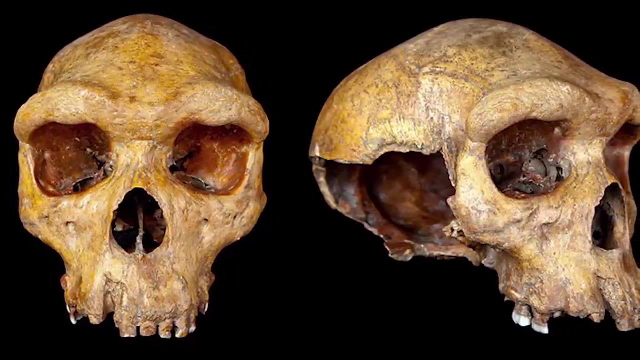 Bones thought to belong to Homo heidelbergensis from Spain indicate that the hyoid bone in Homo heidelbergensis was well developed, Similar in fact to those of our own. The bone was set far enough in the skull to support the tongue and the middle ear bones. 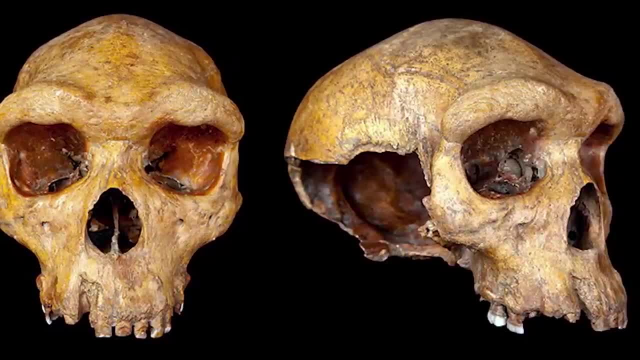 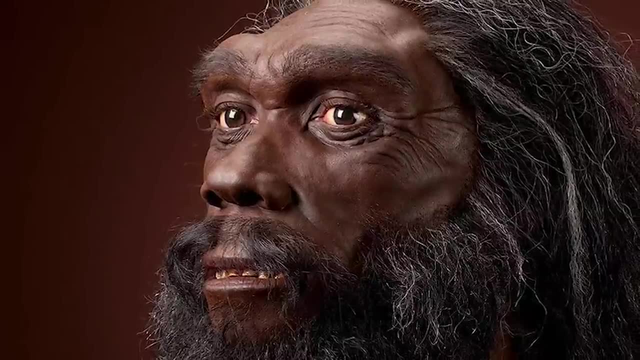 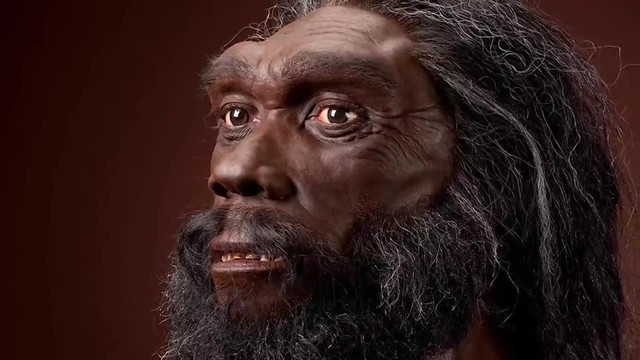 were developed well enough to allow these people to distinguish the frequencies associated with human speech. Even more remarkably, it is thought that these people were predominantly right-handed due to the articulation of marks and striations in the teeth. This is not surprising. 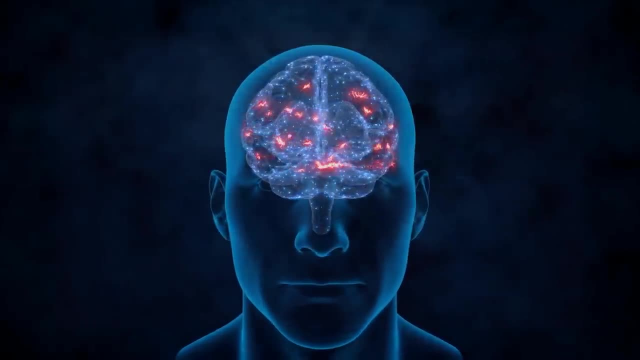 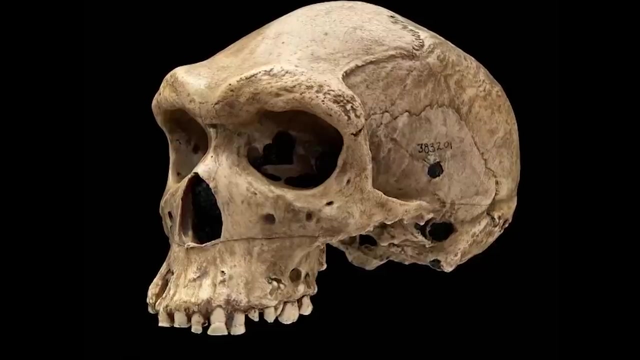 The bone in the skull is the same as the bone in the brain, which is associated with the same section of the brain, which is also associated with language production and speech. Therefore, it is thought that if these specimens do represent Homo heidelbergensis, then the 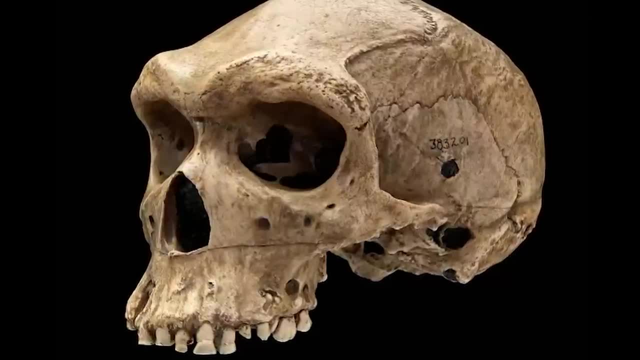 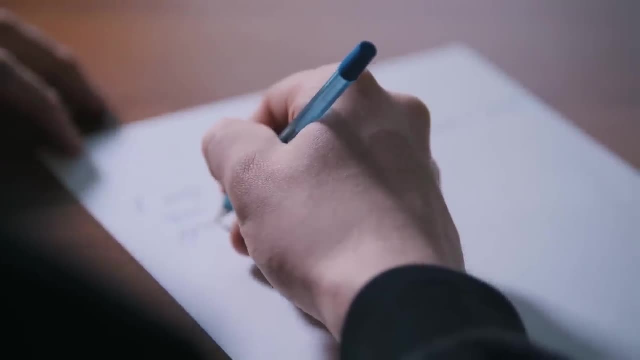 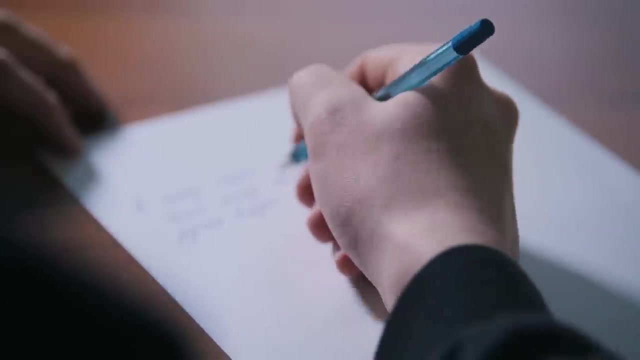 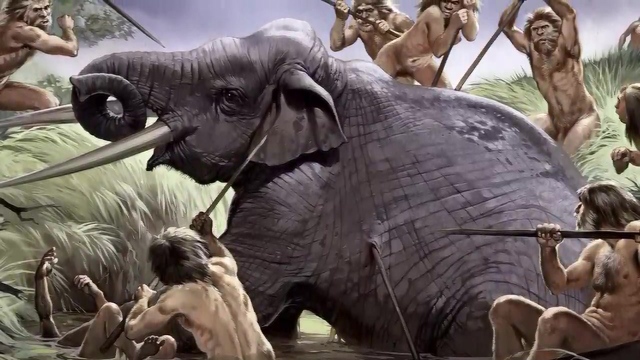 species was capable of speaking in an early form of language, Although, due to the fact that these people were a long way from developing any form of writing, We have no way of determining what exactly it sounded like. Homo heidelbergensis were therefore a highly social species which would have lived and. 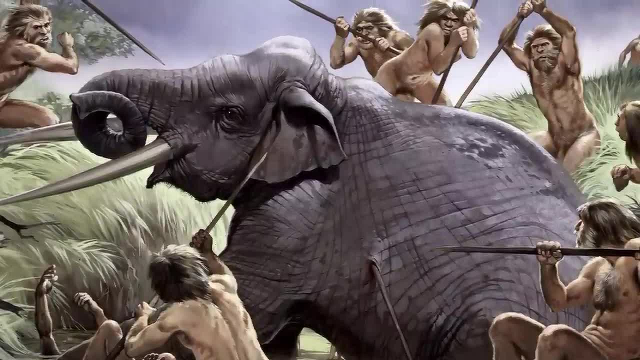 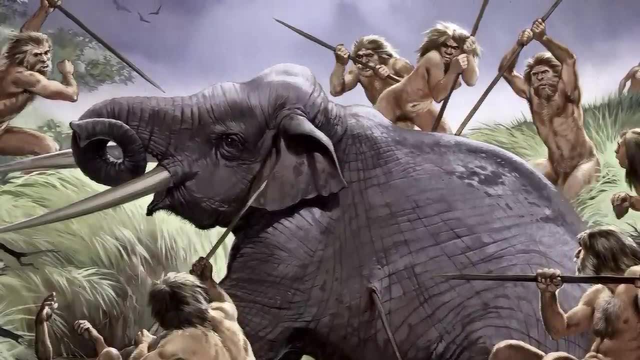 hunted in groups of families and friends, communicating with and learning from one another as they survived the wilds of Pleistocene Eurasia. Little is known about the specific social structure of these humans, But it is thought that they lived in the wilds of Pleistocene Eurasia. 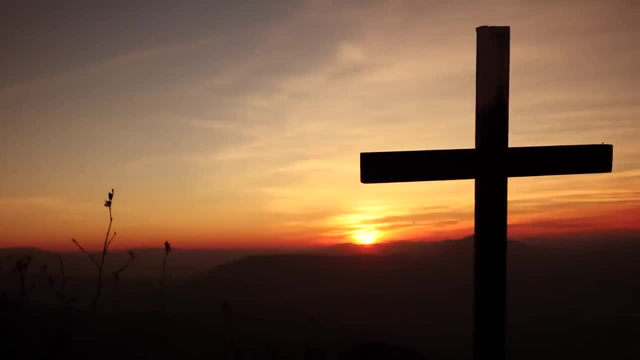 But it is thought that they lived in the wilds of Pleistocene Eurasia, But it is not that they buried their dead, based on the remains of 28 individuals from Spain. This points to one of two things: a broad awareness of the risk presented by decomposing. 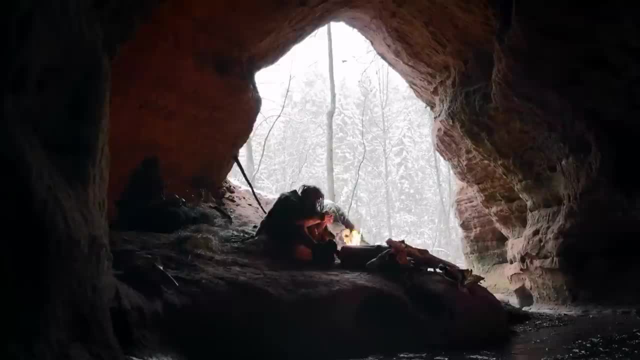 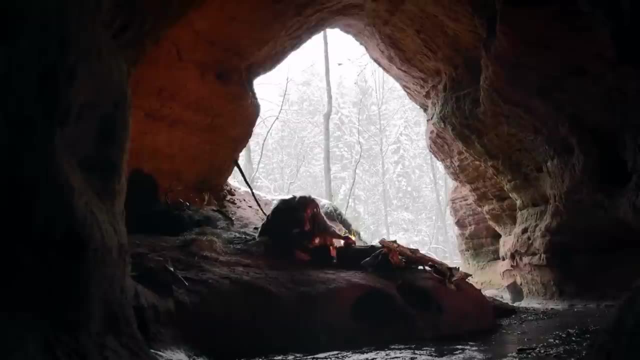 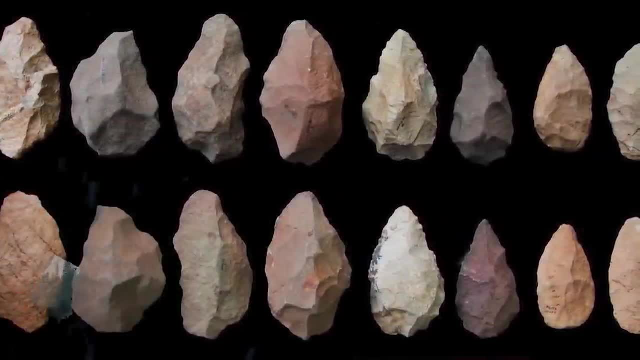 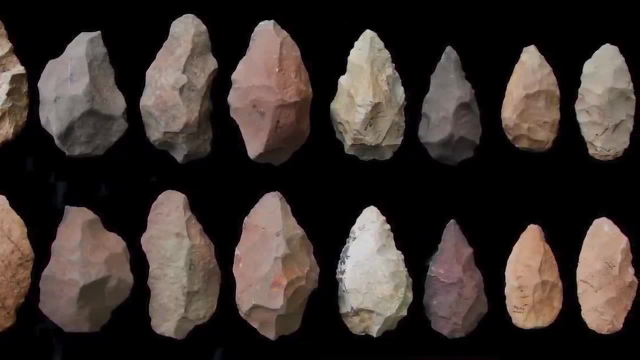 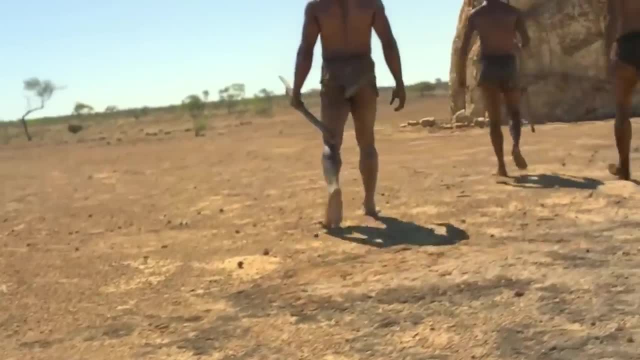 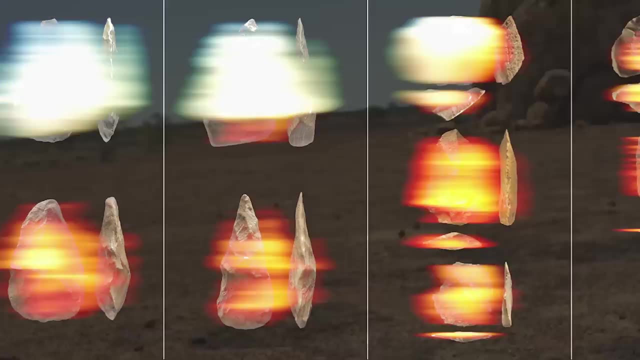 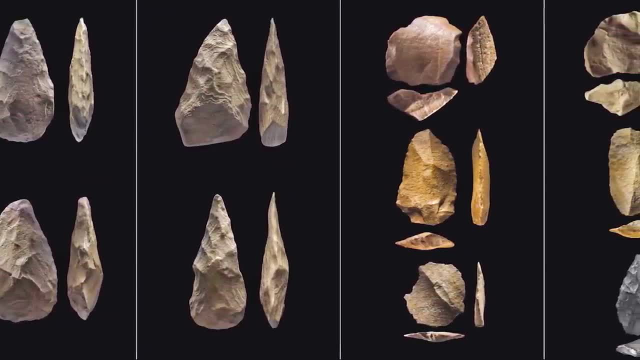 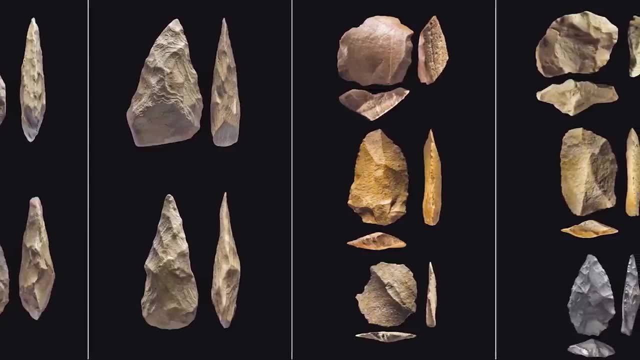 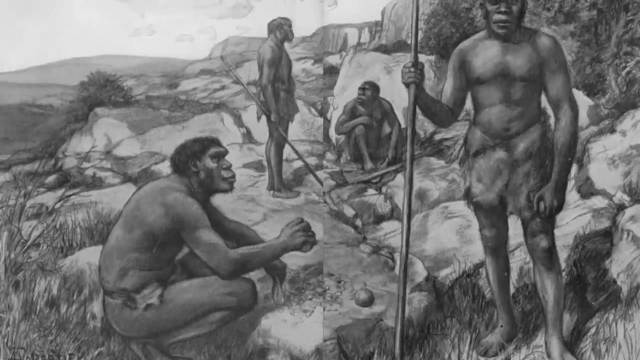 Thanks to the Acheulean stone tools produced by Homo heidelbergensis, we can see simple yet symmetrical hand axes which were specifically crafted to be more lightweight than their predecessors. To become lighter and easier to wield, Homo heidelbergensis designed these tools to be. 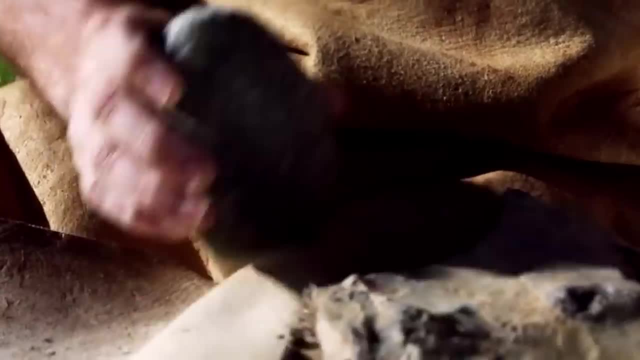 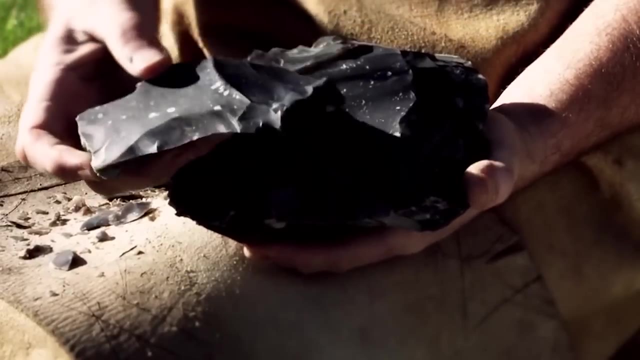 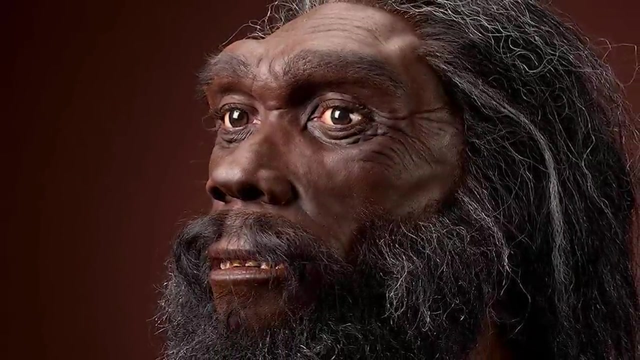 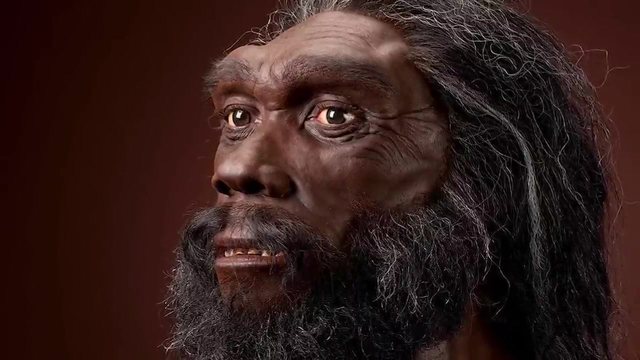 smaller and thinner, a technique achieved by striking the axe from either side, with a hammer-like structure likely composed from a second stone. It is also thought that Homo heidelbergensis had access to specifically prepared platforms or basic table-like slabs, which were reserved for tool preparation. 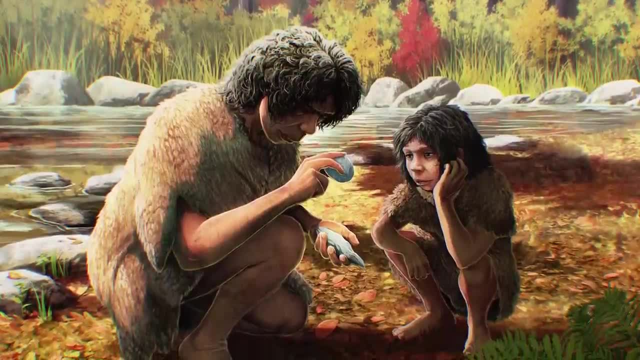 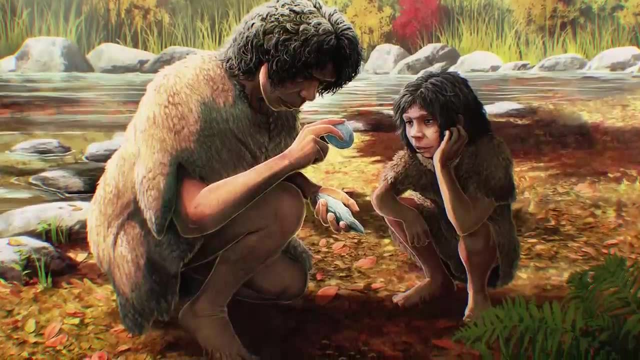 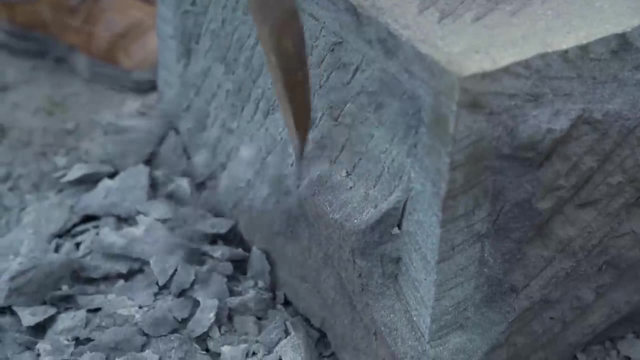 Carved from large pieces of rock. materials required to make specific tools would have been brought to the platform In order to maximize activity Accuracy when constructing a tool. The process of making these hand axes would have resulted in large chips and flakes of rock being sheared off. 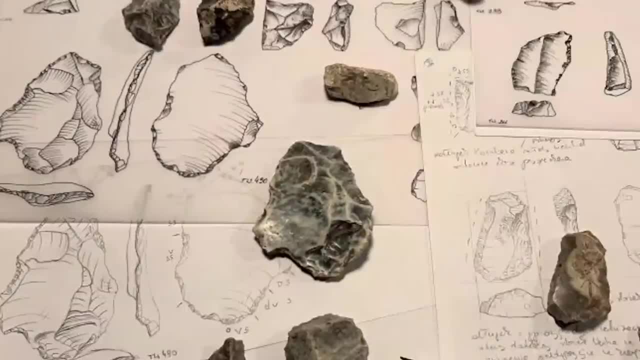 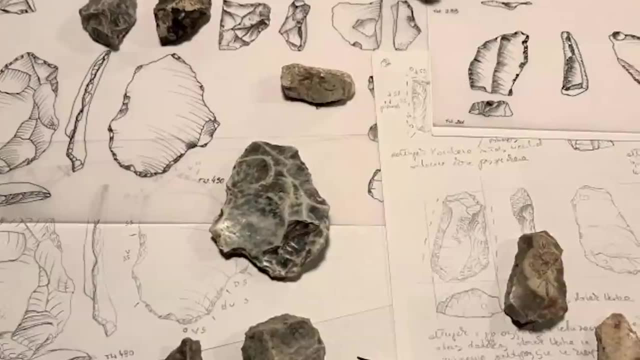 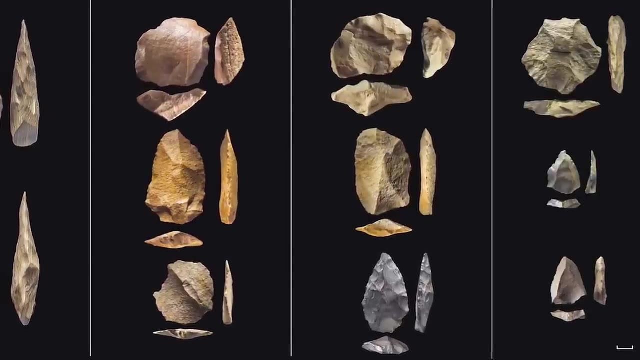 But these were still useful. It is thought that Homo heidelbergensis, alongside other middle Pleistocene hominids, may have recycled excess materials created when constructing tools, Shaping them into smaller tools That would have been able to suit more specific, intricate jobs. 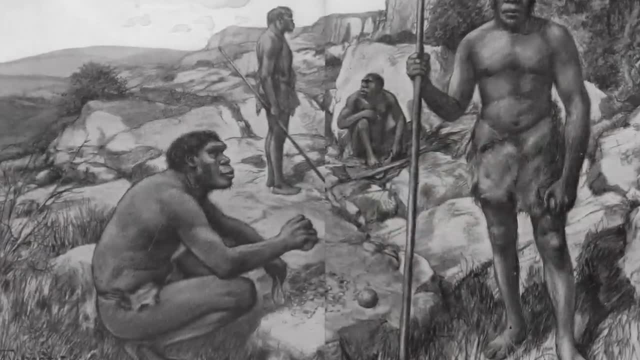 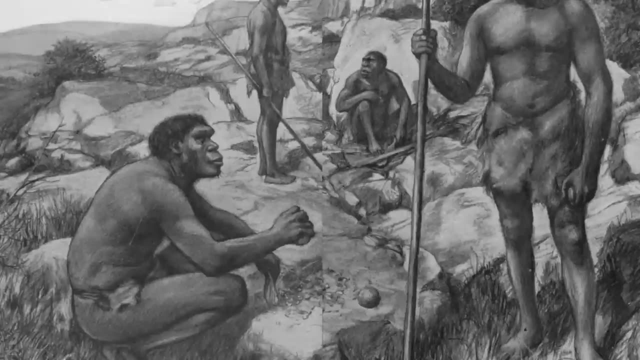 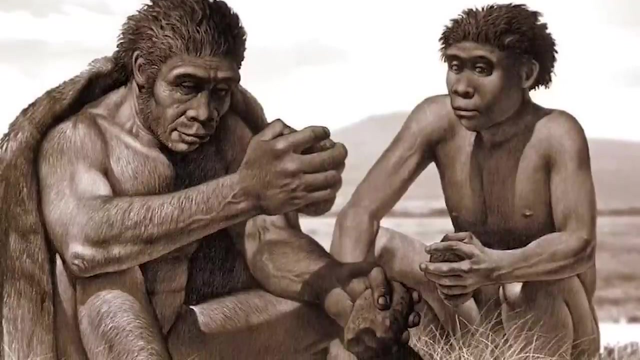 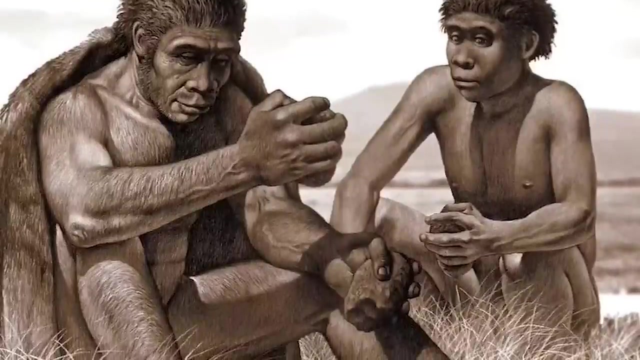 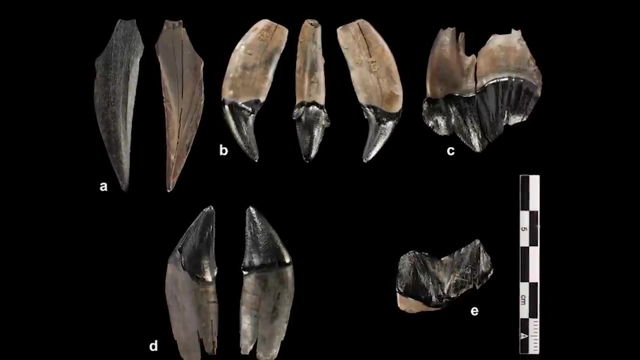 The existence of stone platforms used for designing tools indicates that these people had an understanding of prerequisite technologies, otherwise known as hierarchical organization, Which was a huge step forward for human species going on to create more complex structures later on down the line, Some groups of humans around this time also began to make their tools from bone and deer. 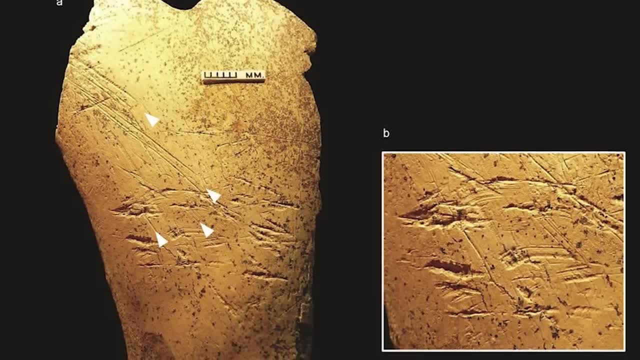 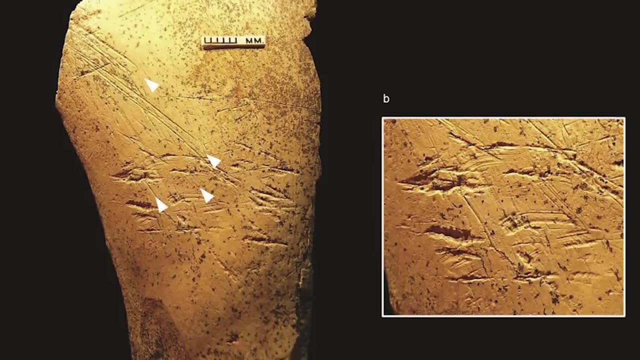 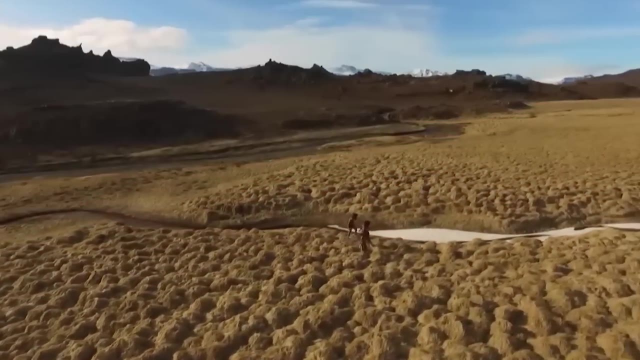 antler, Each of which would have required different techniques and levels of force to construct, Pointing towards the fact that these humans had an understanding of planning, design and material choice. It is possible that Homo heidelbergensis may have been the first human species to have 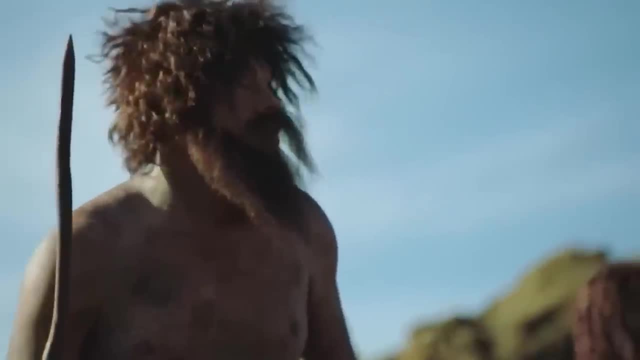 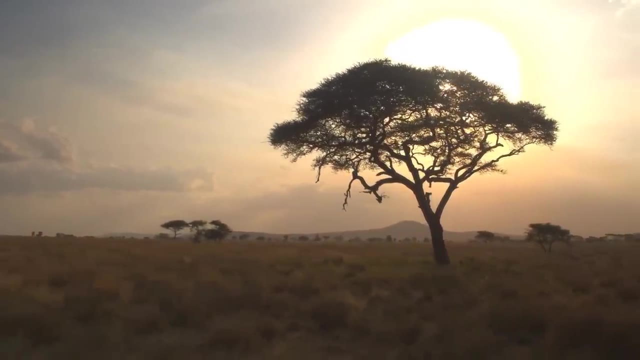 been able to make tools from bone and deer antler. It is possible that Homo heidelbergensis may have been the first human species to have built'em from stone. In rocks belonging to the capthorne formation in what is now modern Kenya, bladelike structures. 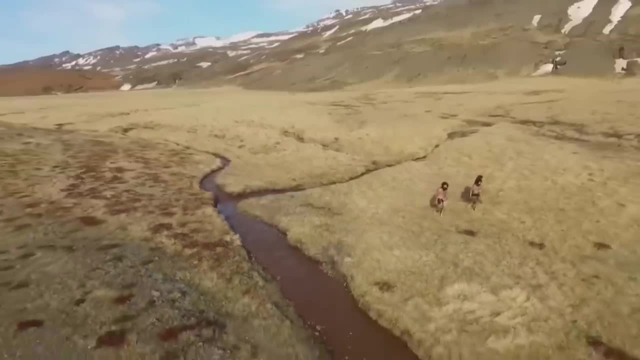 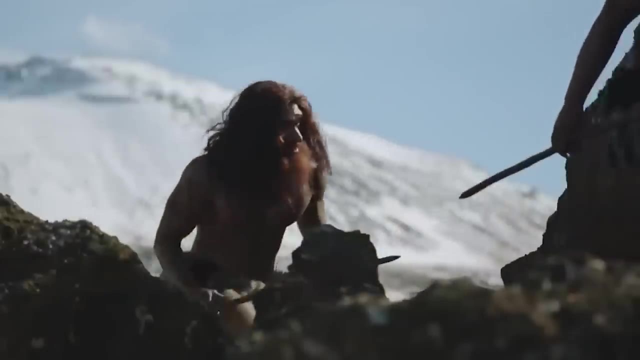 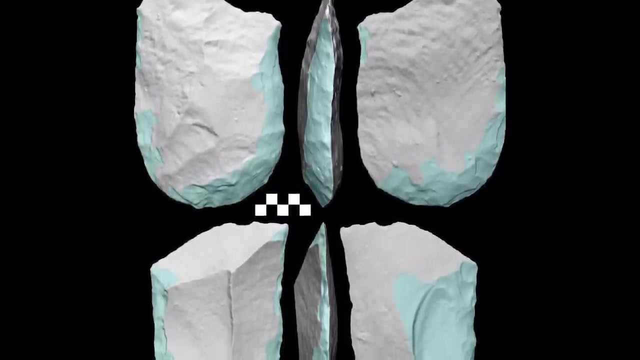 have been found, thought to have been intentionally carved by a species of human who may or may not have been Homo heidelbergensis. These blades and bladelets have been determined to date to around five hundred and forty thousand years ago. 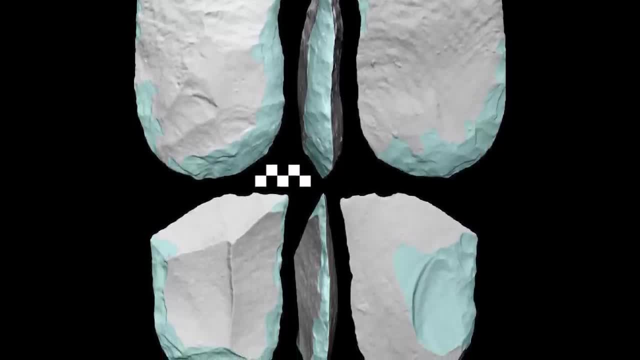 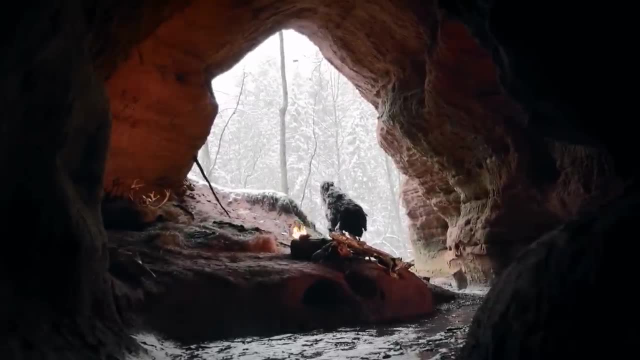 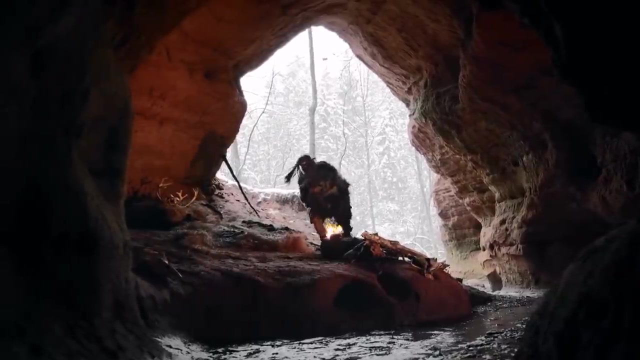 and may have been used as a form of defense or offense against wild animals. It cannot be determined if this technology was passed down from previous generations or if blademaking was a technology that had been lost and rediscovered multiple times across the human evolutionary story. 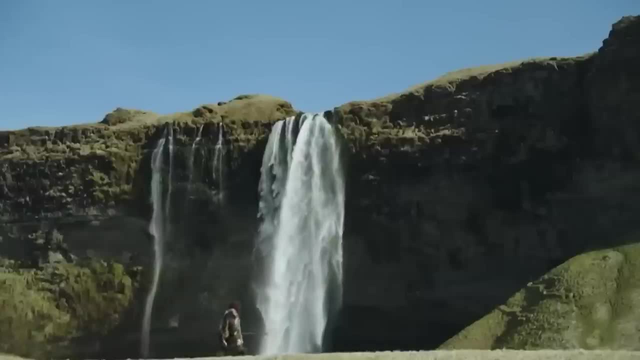 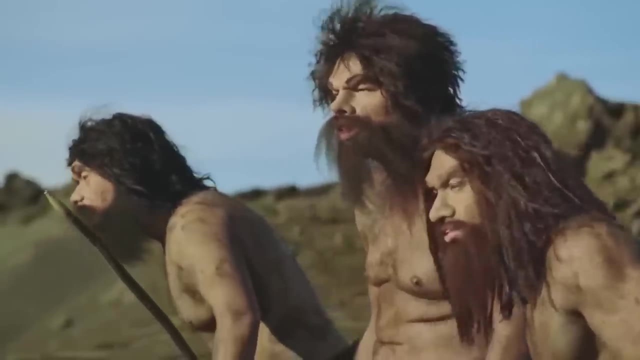 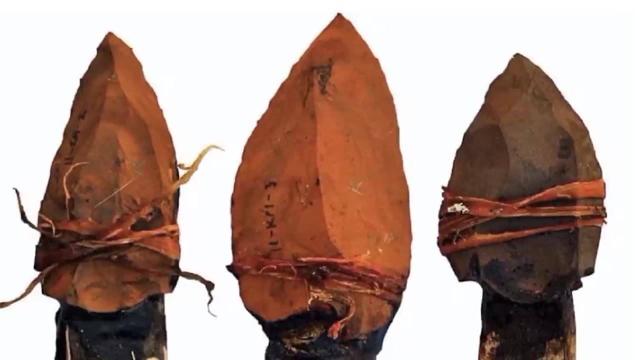 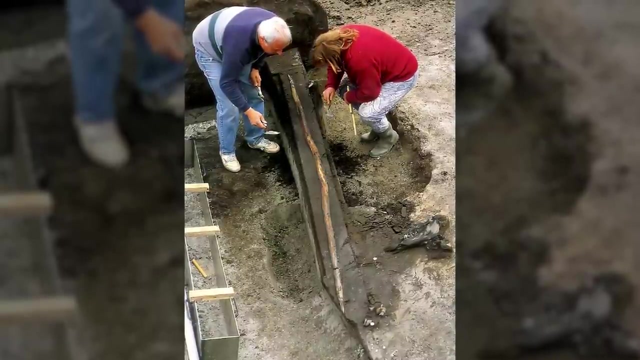 On top of this, Homo heidelbergensis is thought to have been the first human species able to harness the technology of hafting. This involves the attaching of stone points to sticks in order to make basic spears. At the Schöning Inn site in Germany, a total of nine spears and spear fragments have been uncovered. 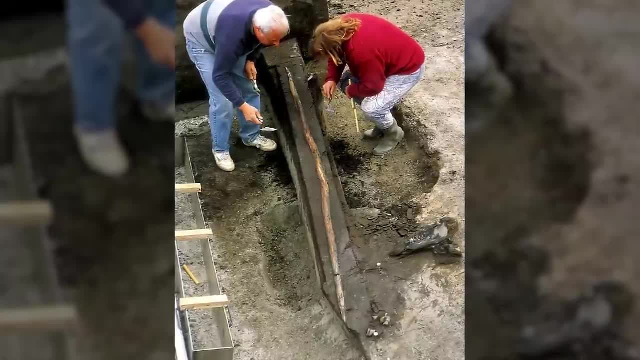 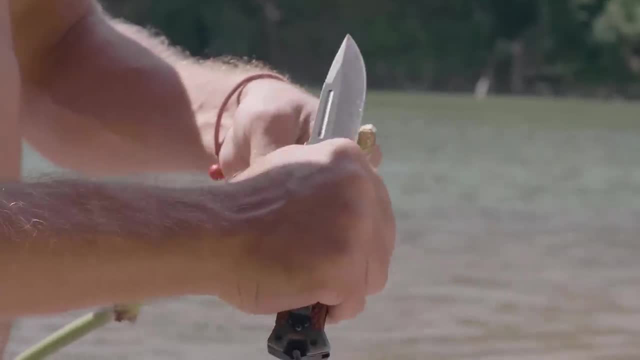 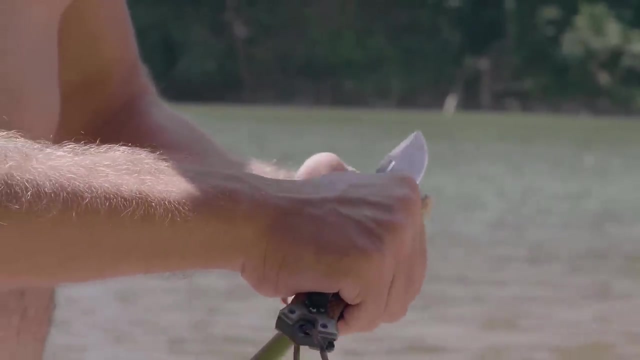 and are thought to have belonged to Homo heidelbergensis. Some of these spears are remarkably complex. One exceptionally long spear could be classed as a basic lance, and one of the spears even has an attachment point for a sharpened stone on both ends. 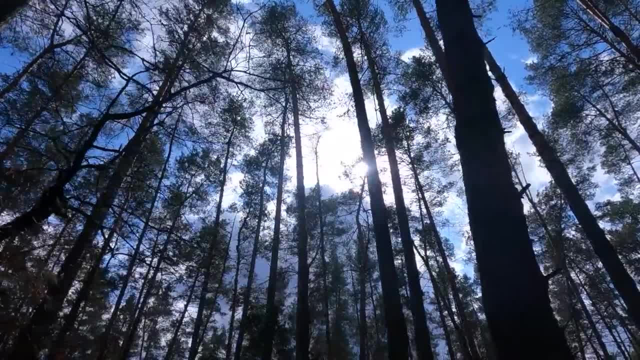 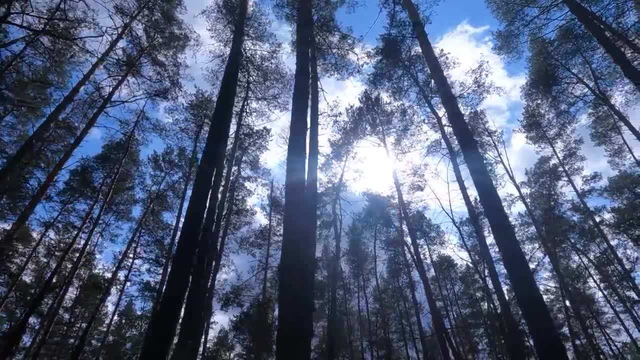 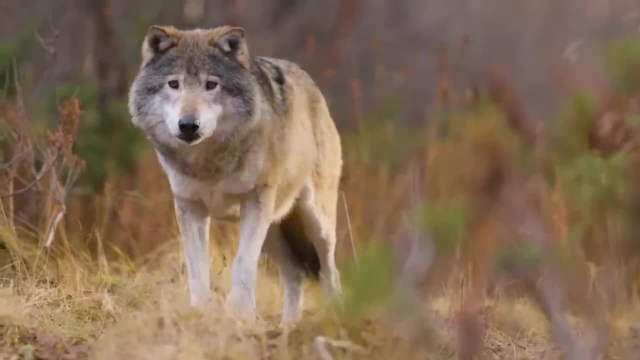 The spears were made from spruce and pinewood and, when fully assembled, could have been up to two and a half meters in length. It is likely that these spears could have been held as melee weapons at close range for keeping animals such as bears and wolves at bay. 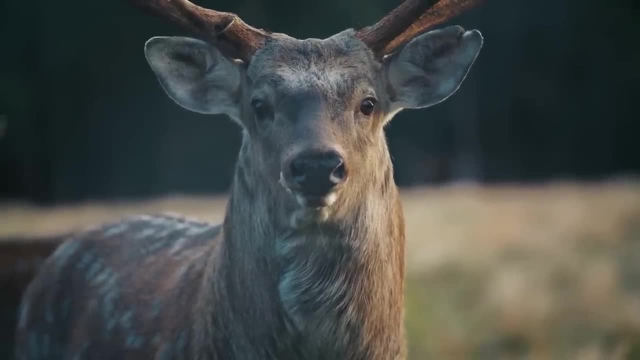 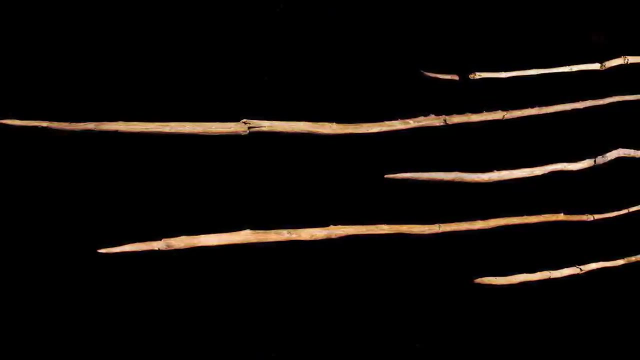 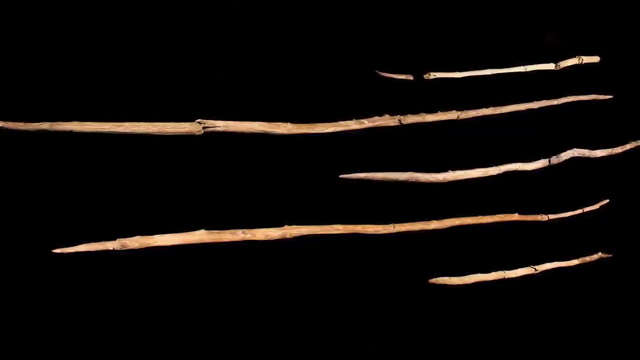 or thrown or stabbed into the flank of a prey animal in order to cause a potentially fatal wound. It is thought that these spears, given their size and the strength of the individuals throwing them, could have been launched 35 meters through the air. 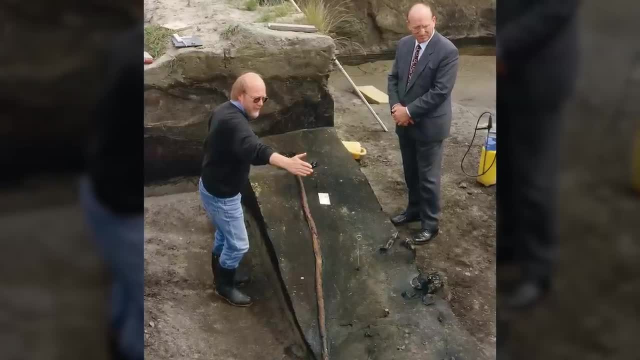 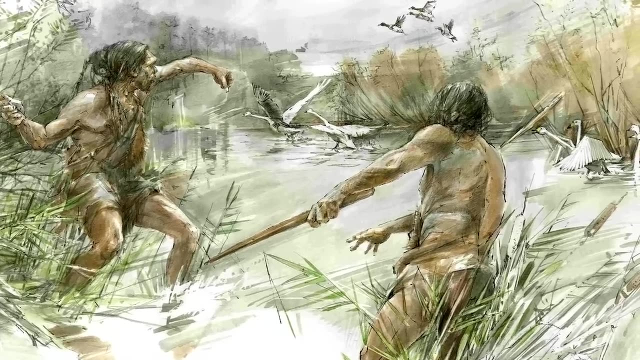 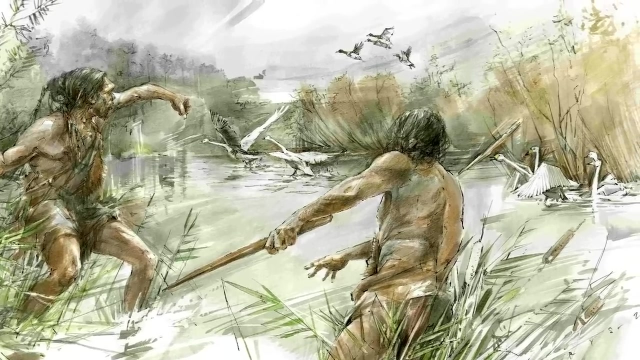 and could have been used as a weapon for the use of weapons, But would have been more effective the closer the thrower was to the target. It is from this technology that humans eventually discovered how to craft more complex and powerful weaponry, including hafted blades and axes. 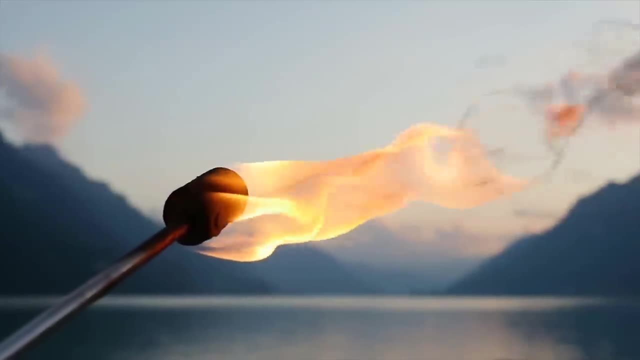 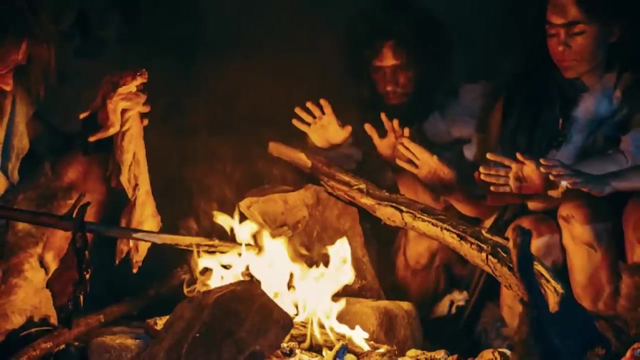 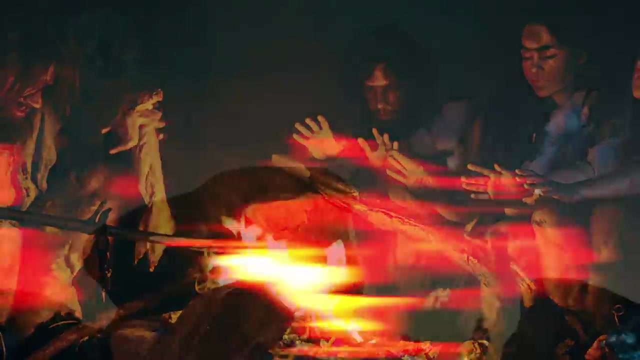 Although evidence for fire use amongst humans is uncommon in the fossil record until around 400,000 years ago, we do know that Homo heidelbergensis would have been able to harness and utilize it effectively. Homo erectus, the species that preceded Homo heidelbergensis, 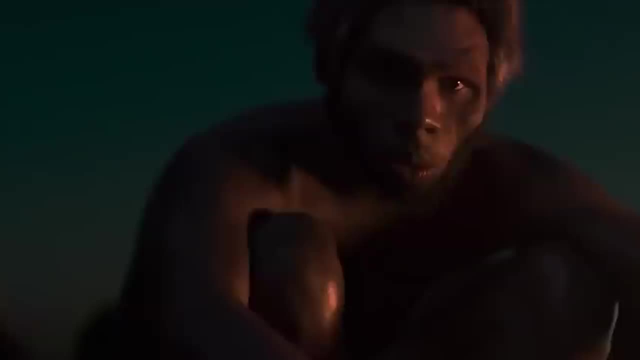 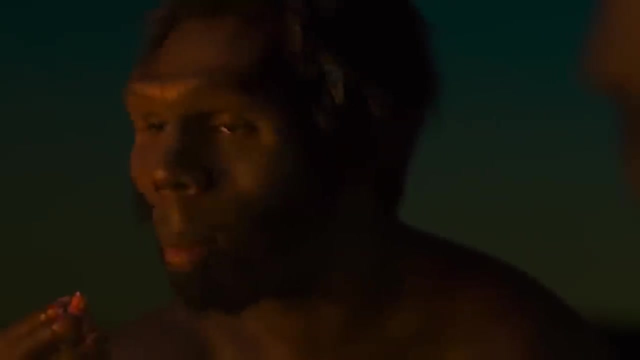 were already utilizing and harnessing fires in their hunts, which proved to be an extremely effective tool for both bringing down large animals and cooking their meat. after, It is thought that the spears were made from spruce and pinewood and that they could be used as a weapon for the use of weapons. 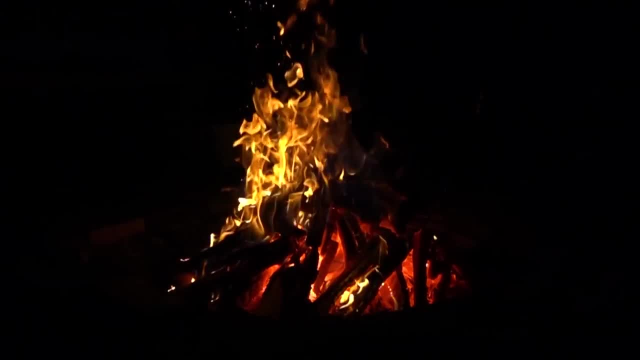 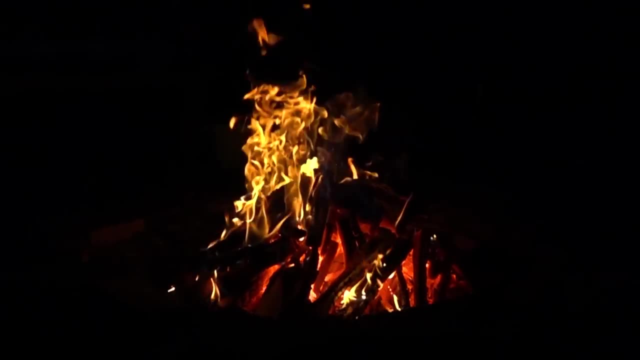 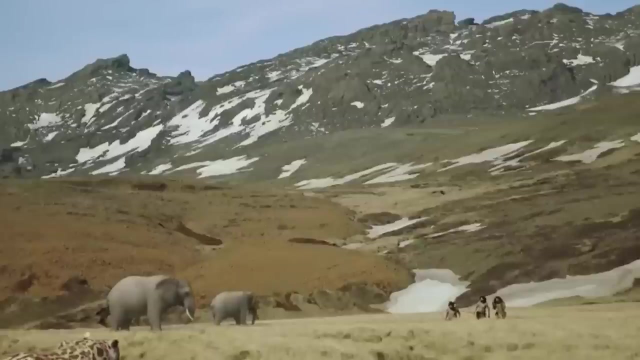 It is thought that the species that followed Homo erectus were able to take this a step further and maintain and manage their fires in a controlled setting. Homo heidelbergensis hunting parties would likely have brought fire along with them to attack large animals such as elephants and rhinoceroses. 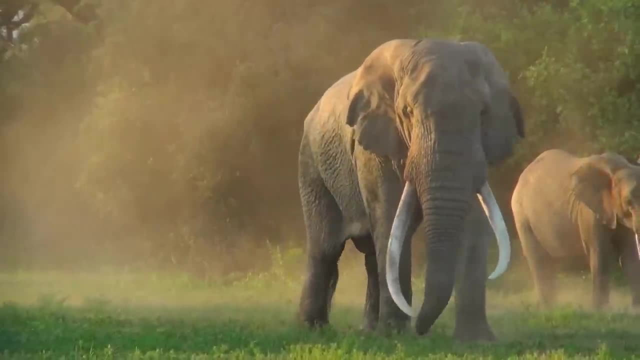 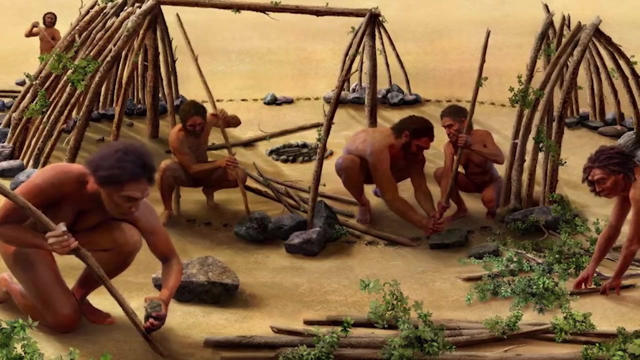 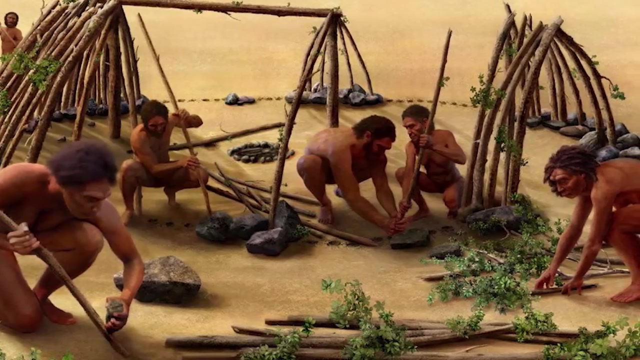 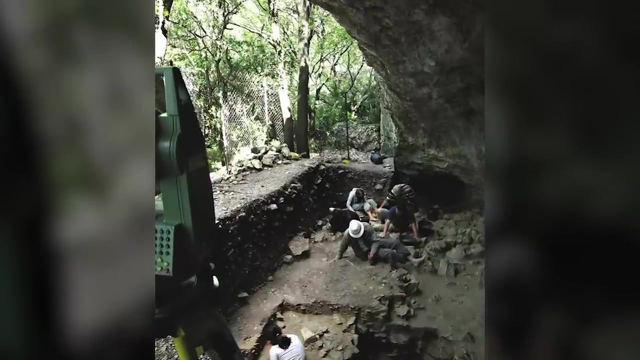 which would have been extremely effective against these animals' tough defensive hides. Finally, Homo heidelbergensis is thought to have constructed basic shelters to defend themselves against the elements when cave space was scarce or occupied by other species. These structures were very simple. 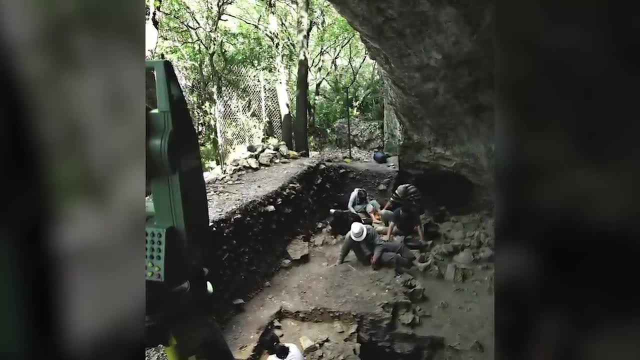 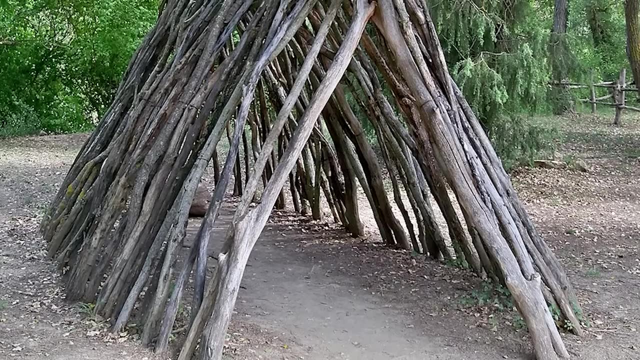 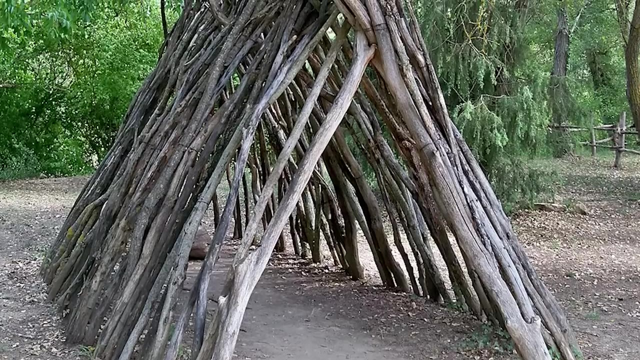 and have been found across Europe in areas sheltered from the weather, such as against the faces of rocks or cliffs. Basic Foundations of Homo heidelbergensis. The foundations of rocks and earth hold thick pole-like branches in place to support a basic roof made of thinner branches. 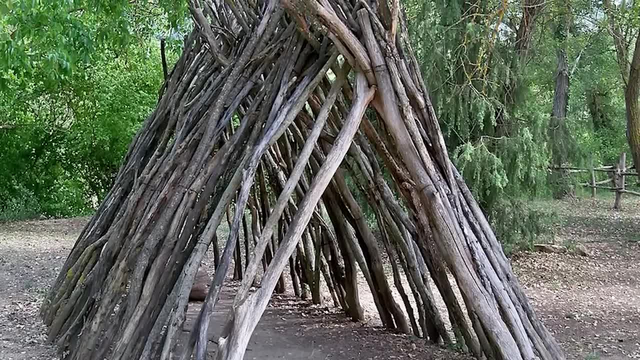 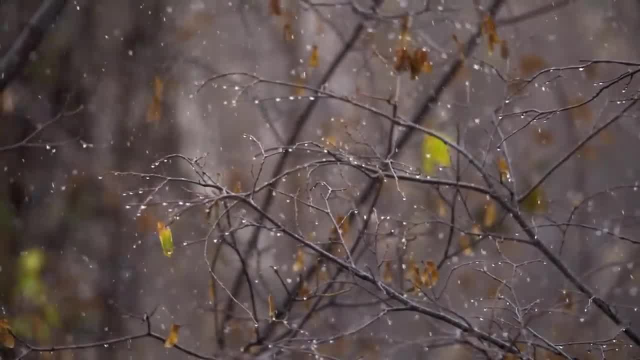 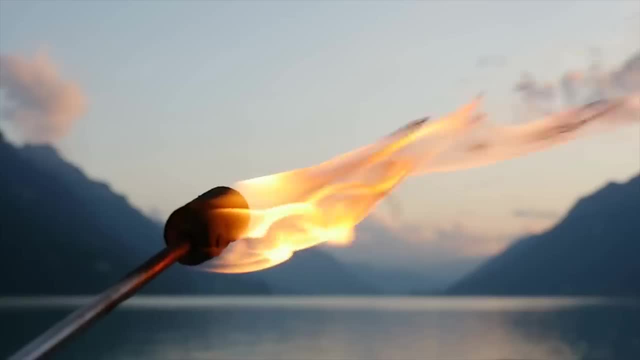 These structures typically measure 3 meters by 3.5 meters and it is thought that they were built in early winter, occupied throughout the harshest season and were only used for sleeping in at the time. All evidence of fire use in early hominins. 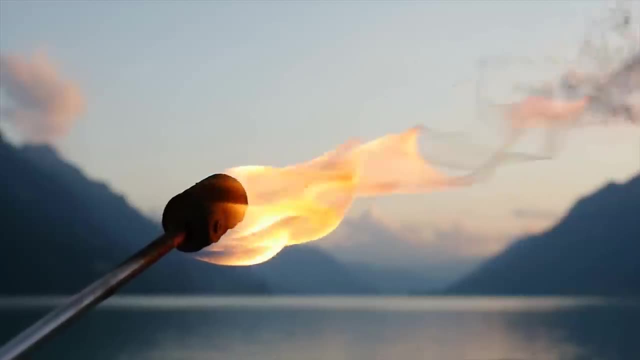 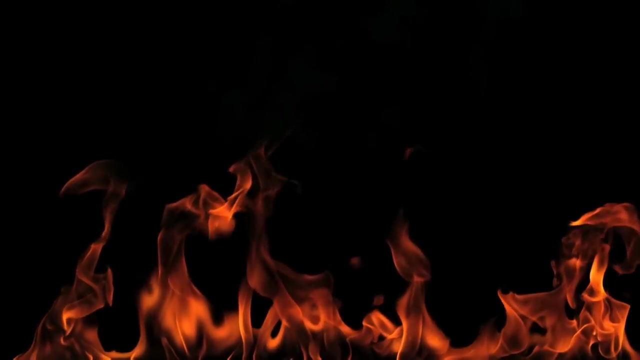 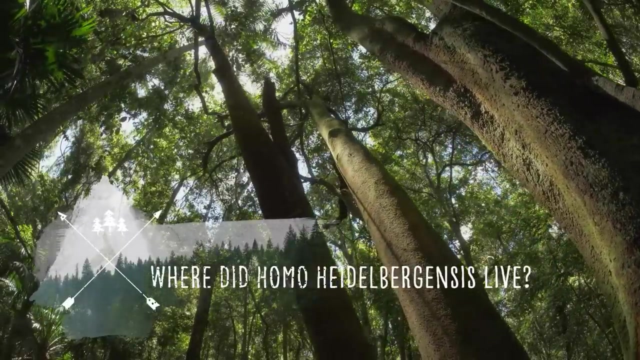 appear to have taken place in the entrances of caves or outside, altogether, likely to prevent the dangers of smoke or a spreading dangerous fire from affecting the group Homo heidelbergensis. Much of the environment traversed by Homo heidelbergensis would have consisted of steppes and forests. 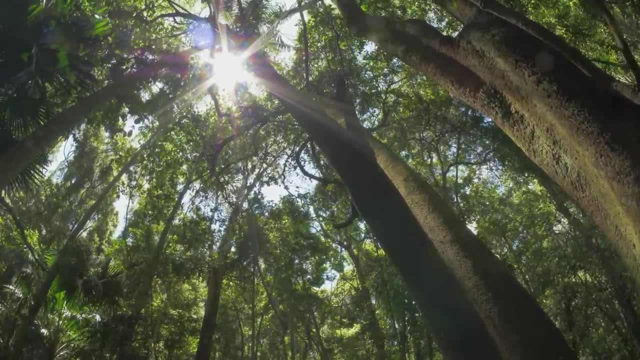 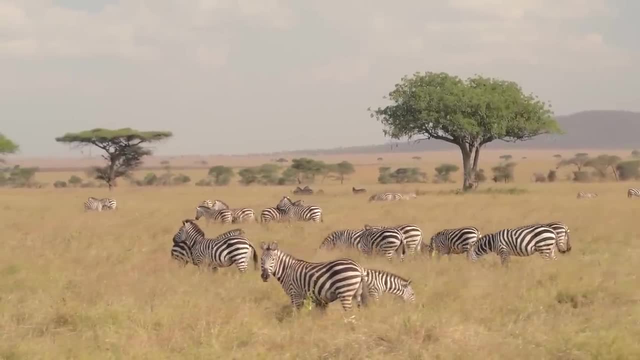 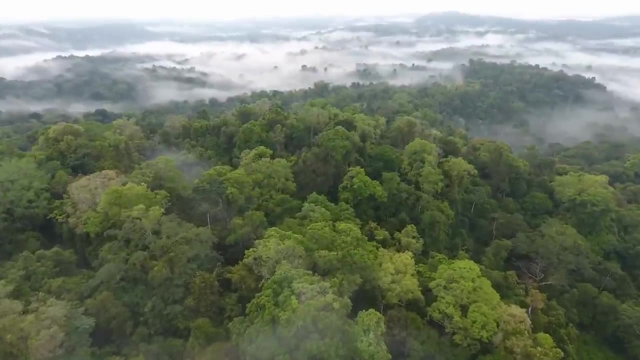 cool and cold in temperature. to the north, to the south, in the lower reaches of Europe and the vast swaths of Africa, Grasslands and plains would have dominated the landscape, offset by patches of forest and the occasional mountain. Homo heidelbergensis was an adaptable and hardy species. 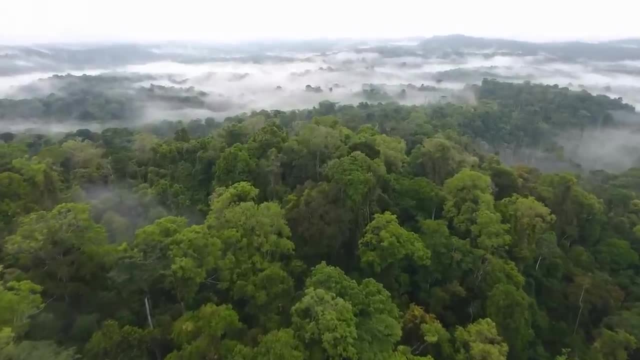 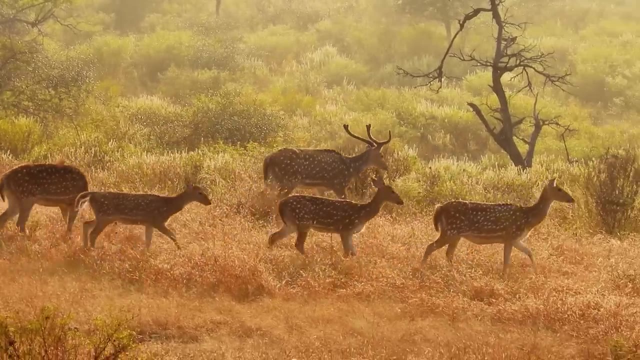 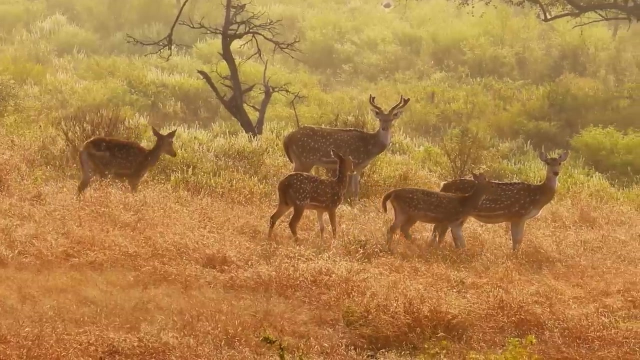 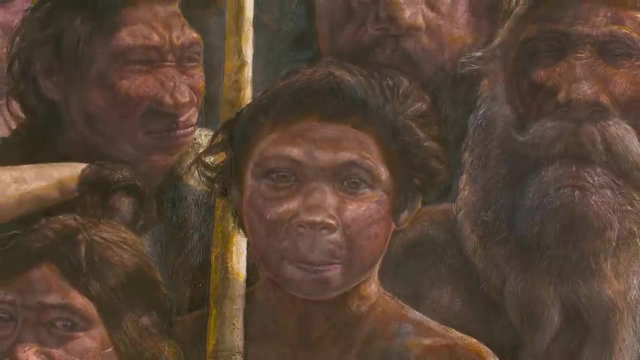 that could therefore inhabit a wide variety of ranges and environments and could have exploited a plethora of food sources in these environments. Alongside the food sources associated with the species, many dangers would have been present across the ranges they inhabited. Rival groups of Homo heidelbergensis could have posed a significant threat. 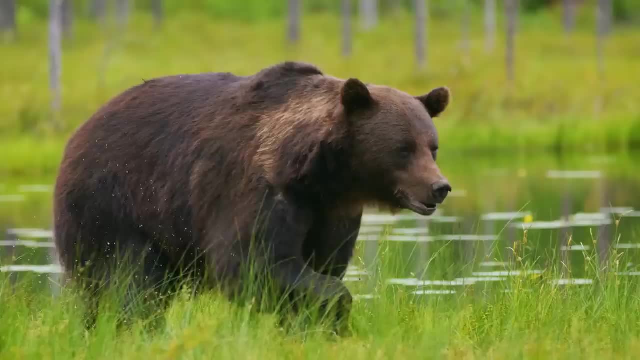 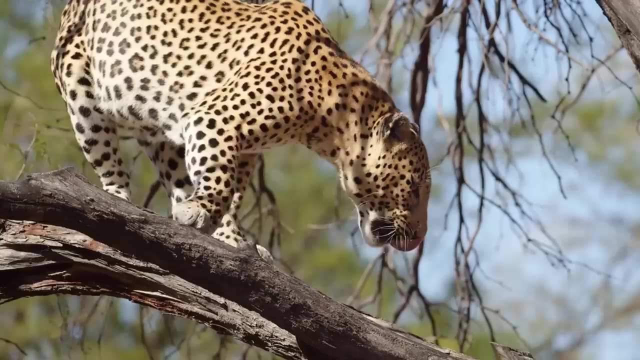 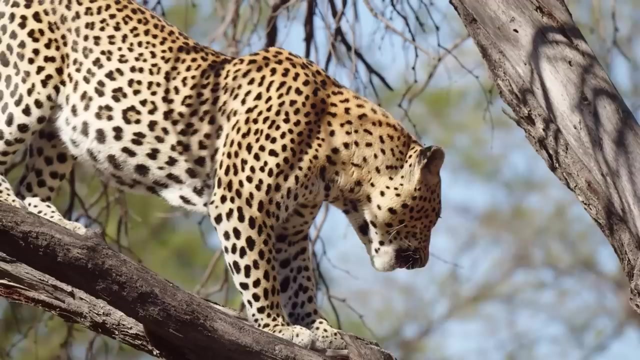 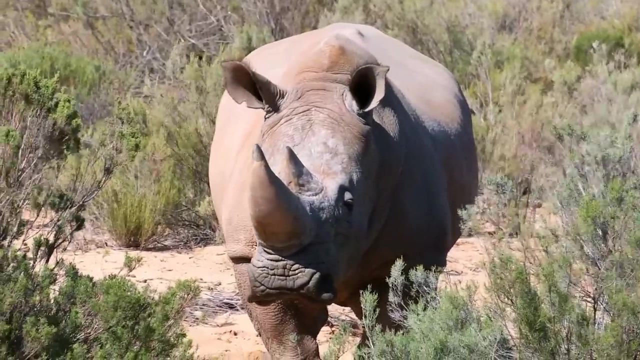 especially if times were tough. Dangerous mammals such as bears and wolves are known across the Eurasian ranges, and large, powerful species could be found throughout Africa. across the time, Homo heidelbergensis was present on the scene. Add to that the presence of dangerous herbivores. 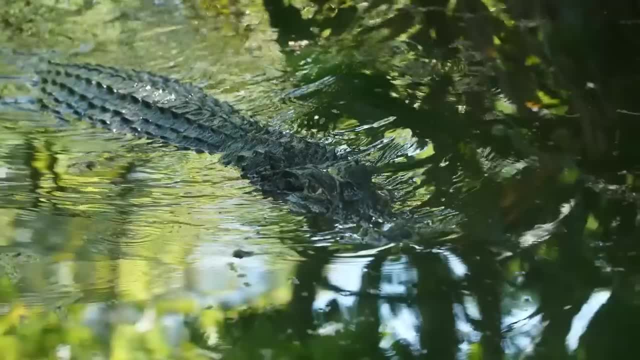 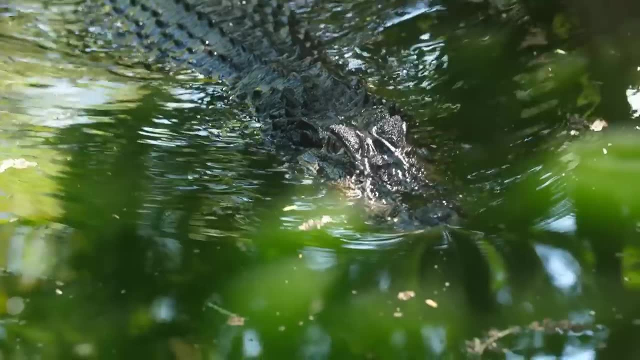 such as hippopotamuses and rhinoceroses, and carnivorous reptiles such as snakes and crocodilians, and you have a dangerous range of environments that could have quickly proved lethal for a young, sick, inexperienced and ill-mannered animal. 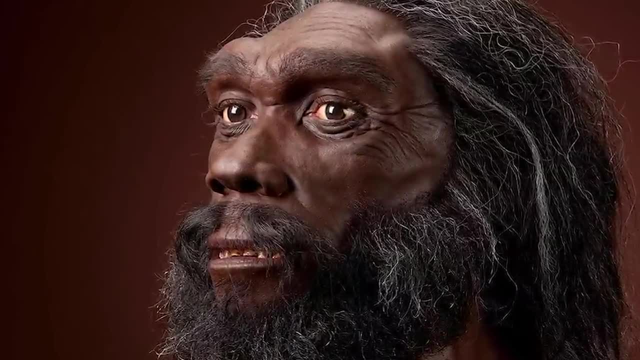 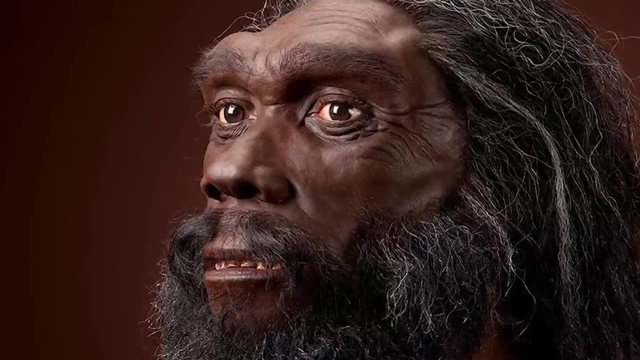 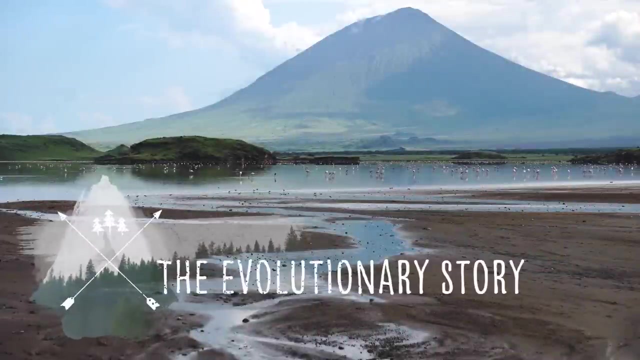 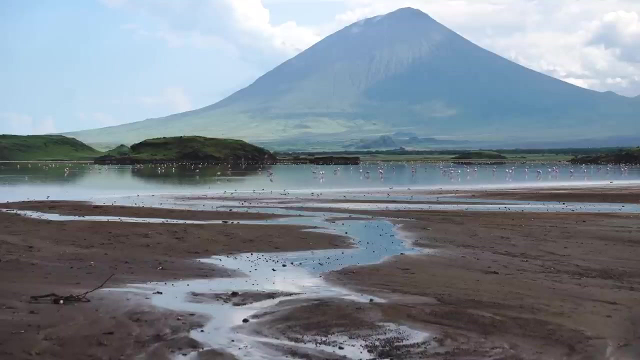 These early humans needed to be hardy and defensive if they were to survive in these harsh landscapes. So how did Homo heidelbergensis initially come to be? The species is, in fact, thought to have evolved directly from populations of Homo erythritus. 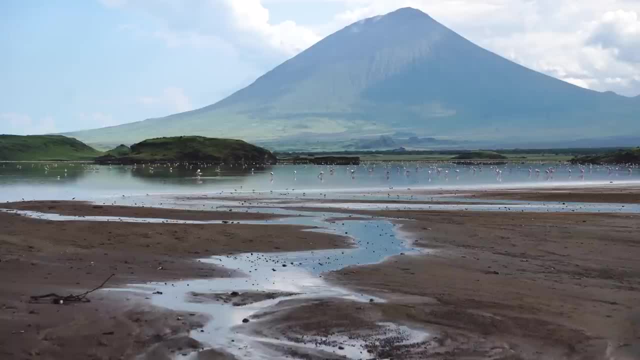 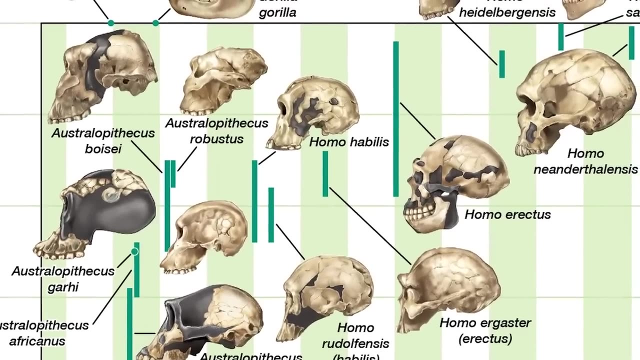 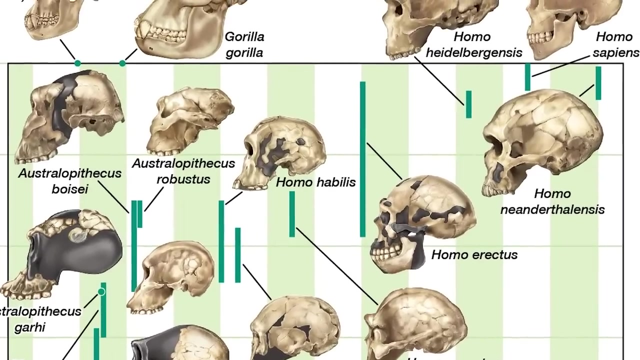 in Africa around 700,000 years ago. This is a process that is thought to have begun around 2 million years ago during the migration of hominins out of Africa and into the wider ranges of Eurasia. Returning briefly to the debate, 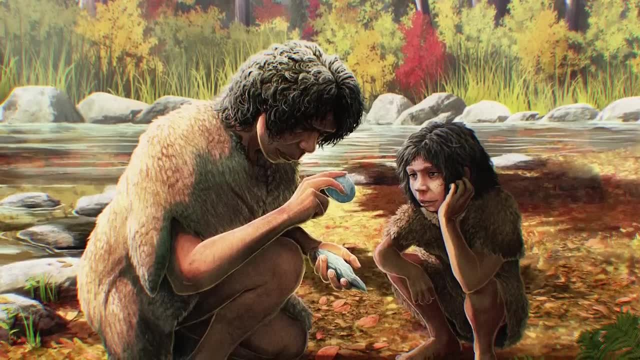 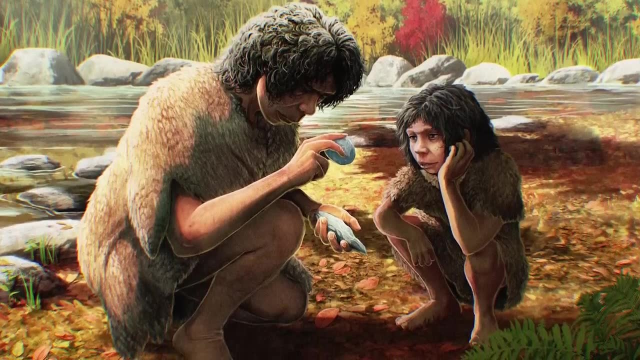 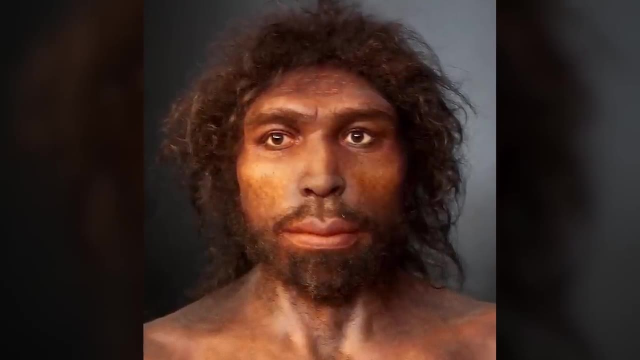 on how Homo heidelbergensis should be classified. some scientists believe that Homo erectus split into two groups, the Homo heidelbergensis in the north and Homo rhodesiensis in the south, while other scientists believe that Homo heidelbergensis occupied both regions. 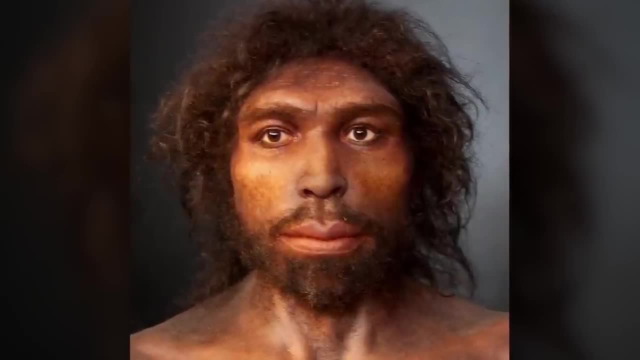 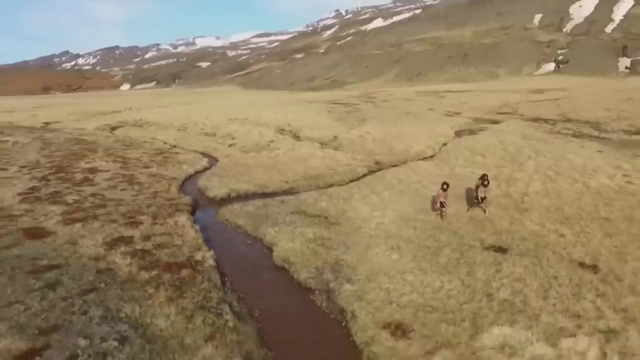 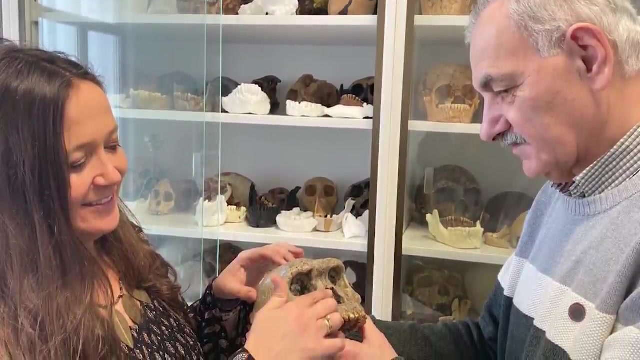 as the same species. It is commonly thought that Homo heidelbergensis is the ancestor of modern humans, Neanderthals and Denisovans, But Spanish archaeologist Jose Maria Bermuda de Castro came up with a differing theory in 1997.. 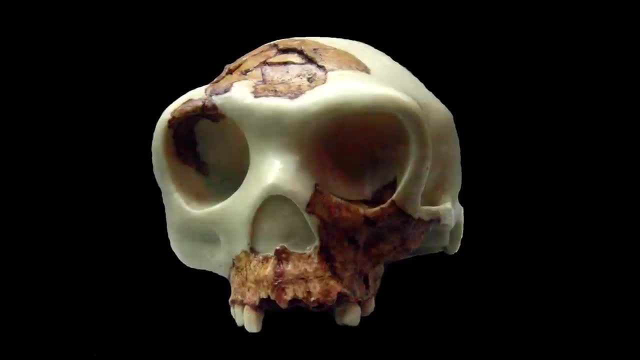 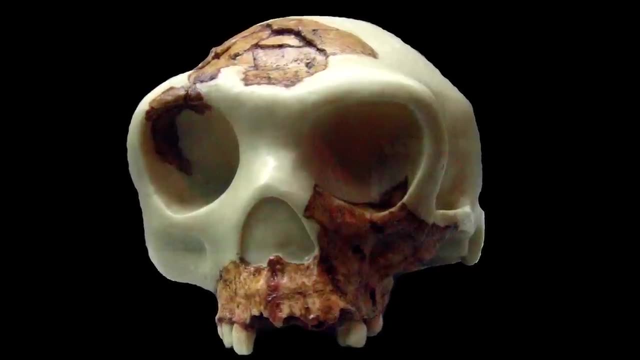 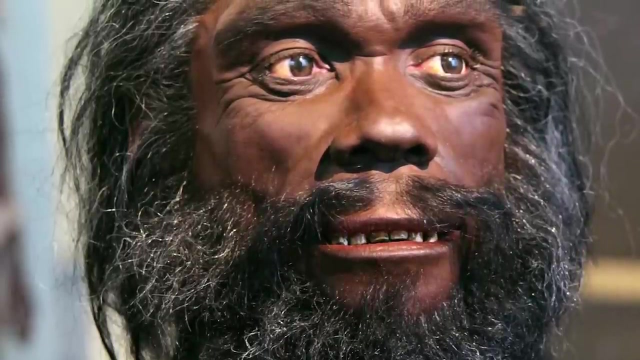 He suggested that at the time, the newly discovered Homo antecessor, known from Spain, represented the ancestor of just Homo sapiens and that Homo heidelbergensis represented a different line descending from Homo antecessor into Neanderthals and Denisovans separately. 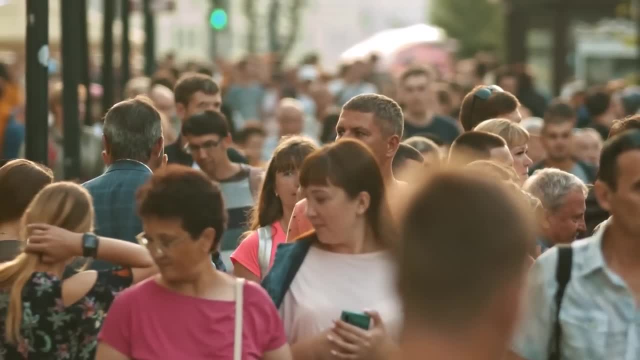 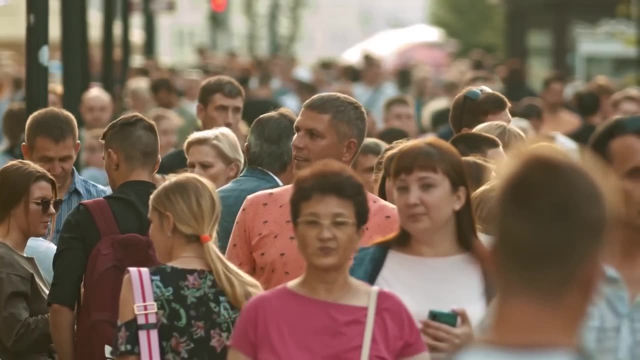 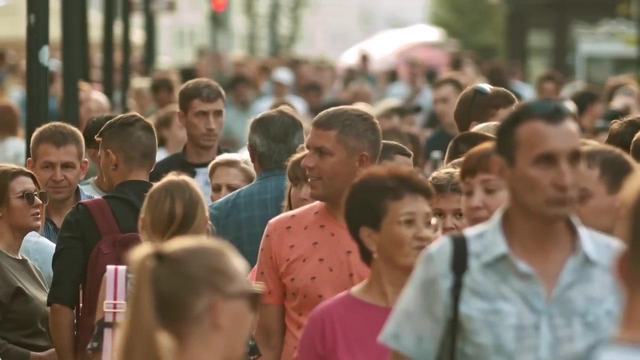 If his theory were true, that would mean that we are not directly descended from Homo heidelbergensis and that the last common ancestor we share with the Neanderthals and the Denisovans would be Homo antecessor. Interestingly, Jose later backtracked on this opinion. 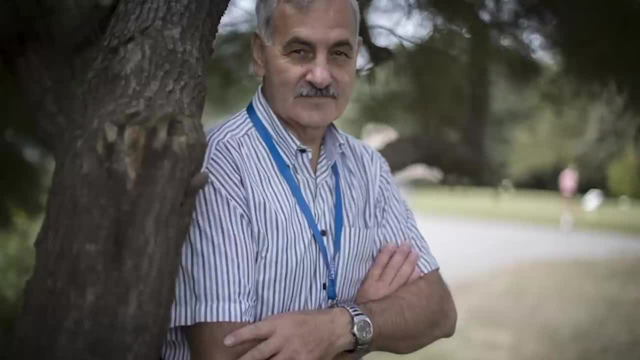 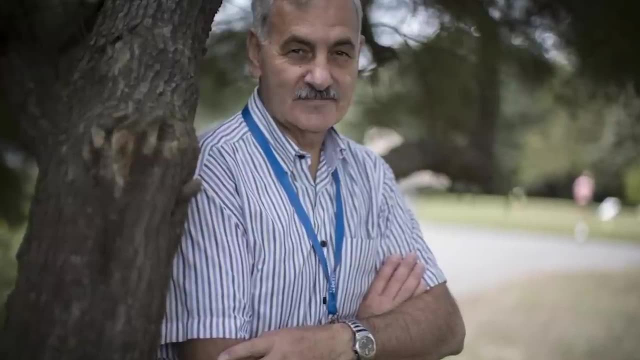 and returned to the original belief that Homo heidelbergensis was the last common ancestor of Homo sapiens and Homo neanderthalensis and that Homo heidelbergensis was the last common ancestor of Homo sapiens and Homo neanderthalensis and that Homo heidelbergensis was the last common ancestor of Homo heidelbergensis. 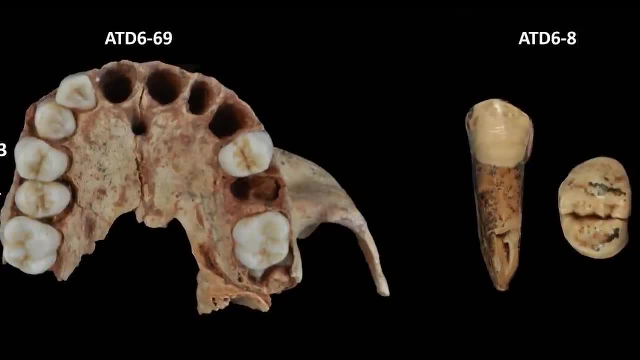 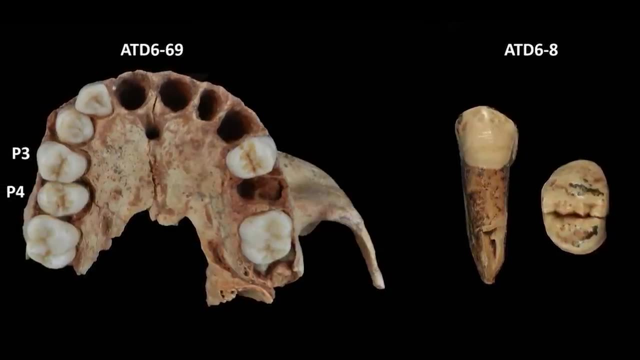 and that Homo heidelbergensis was the last common ancestor of Homo heidelbergensis. It was later discovered, based on evidence collected from Homo antecessor teeth by paleoanthropologist Fredo Welker in 2020, that Homo antecessor was not an ancestor. 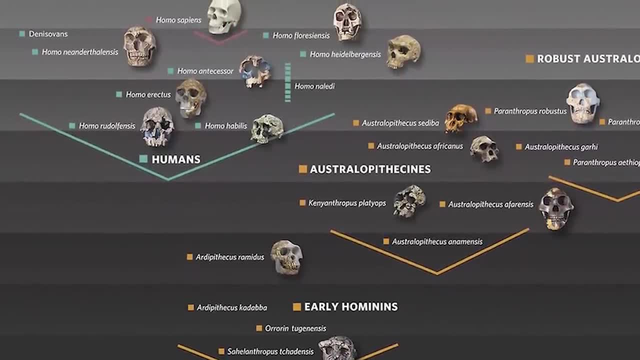 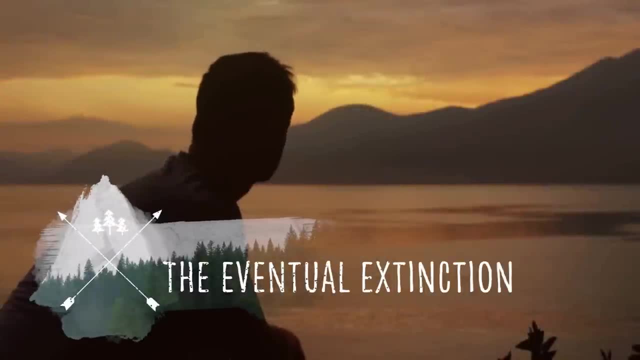 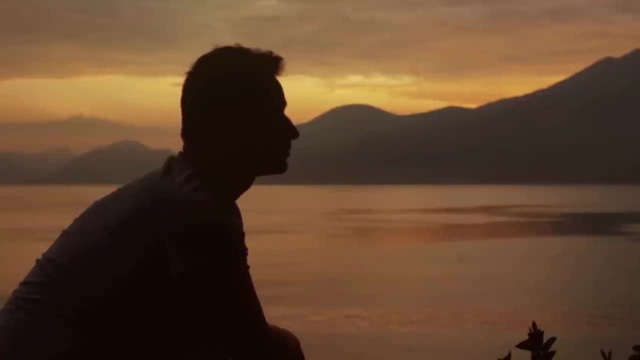 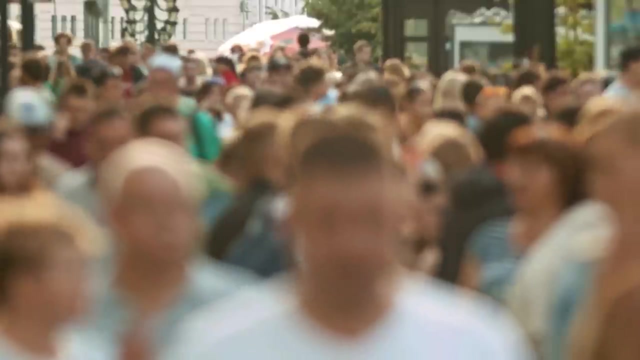 to Homo heidelbergensis, and the species were, in fact, sister lineages. This segment may, in fact, have a misleading title, as Homo heidelbergensis is thought to have evolved into our species rather than having gone extinct. That being said, only select populations of Homo 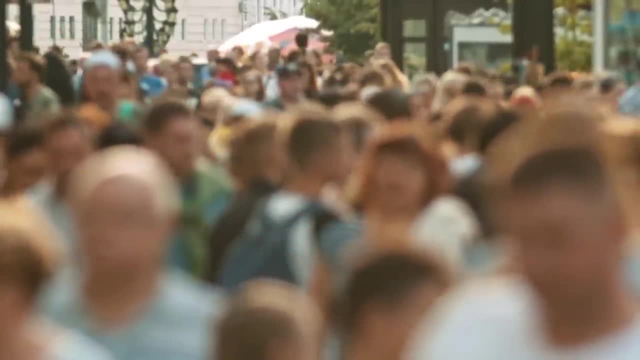 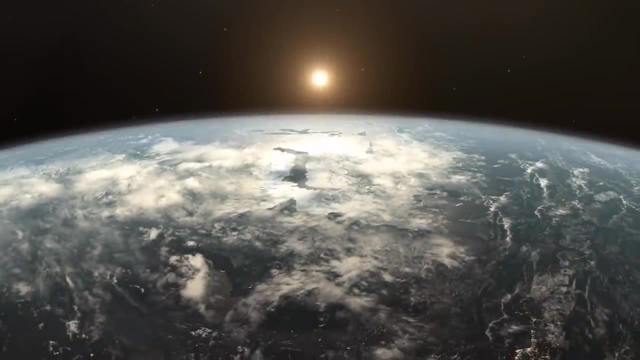 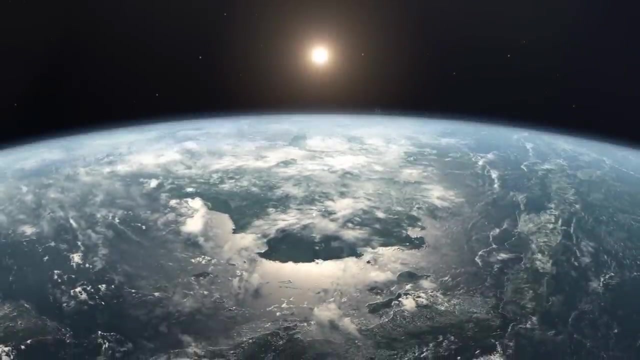 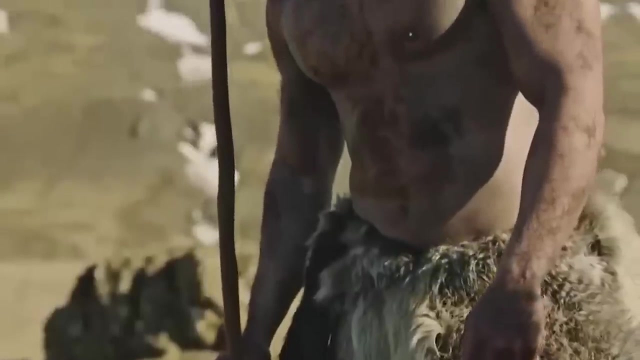 heidelbergensis would have transitioned into our own species, those who adapted to the changing world. Climate change and a potential lack of food sources in some regions may have driven the Homo heidelbergensis- individuals who failed to adapt- to their demise, with only the successful genes being passed on to the 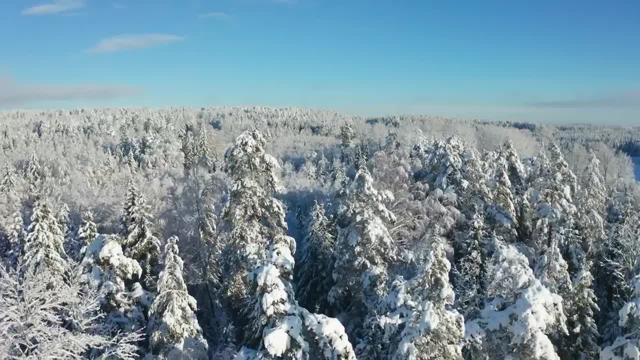 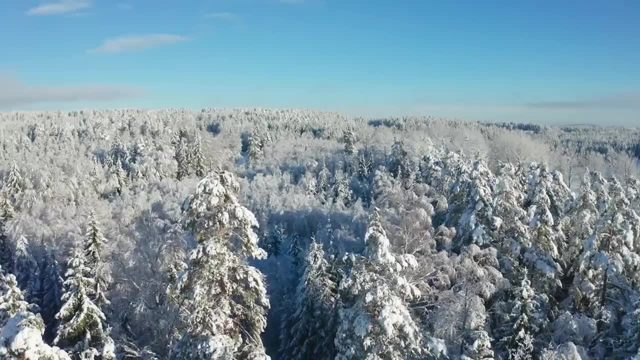 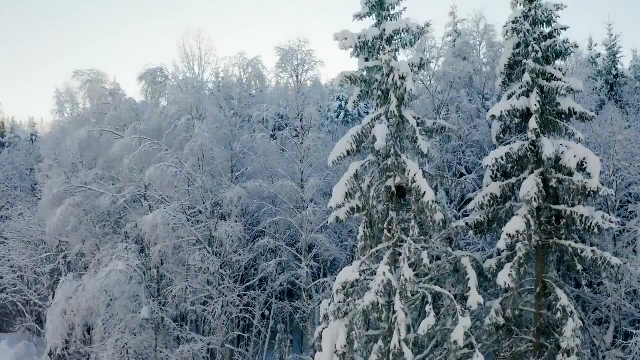 descending species. As the climate changed towards the end of the Homo heidelbergensis' appearance in the fossil record, the environment and the food within it would also have begun to alter. The disappearance of food sources that are not known to the general public and the lack of food sources that are not. 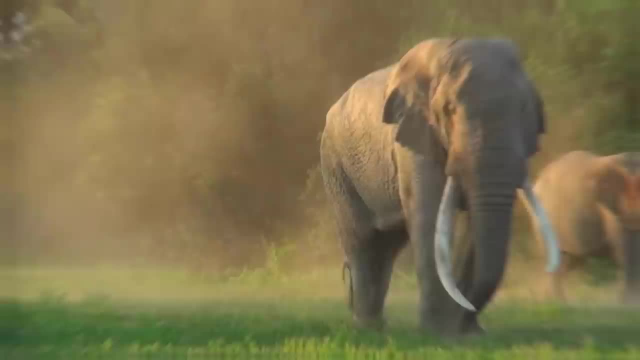 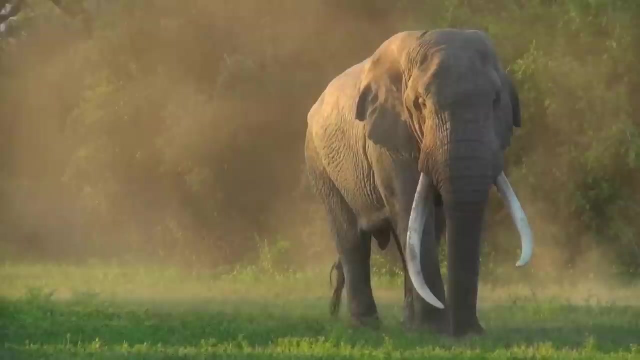 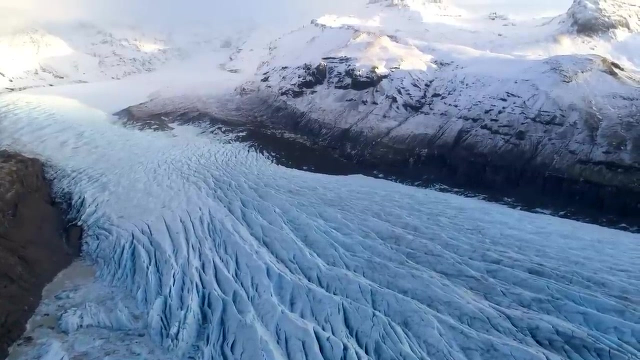 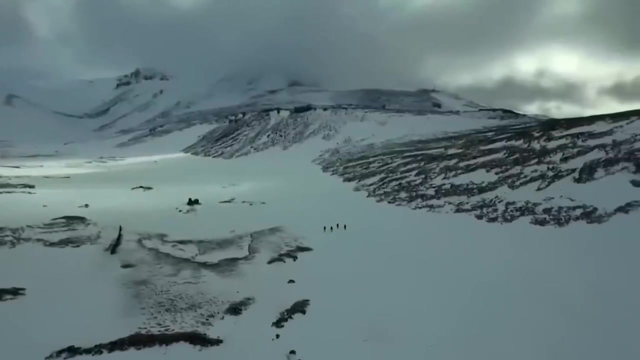 the species relied on in certain areas, such as the megafauna, mammals such as elephants and rhinoceroses would have caused a massive struggle amongst existing communities And, one by one, the groups that could not adapt faded into the depths of prehistory. The same thing would happen to their eventual ancestors. 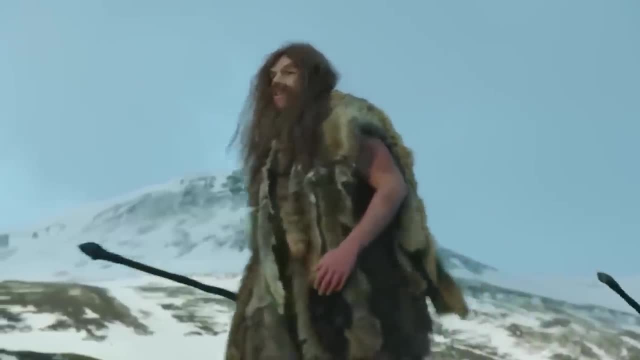 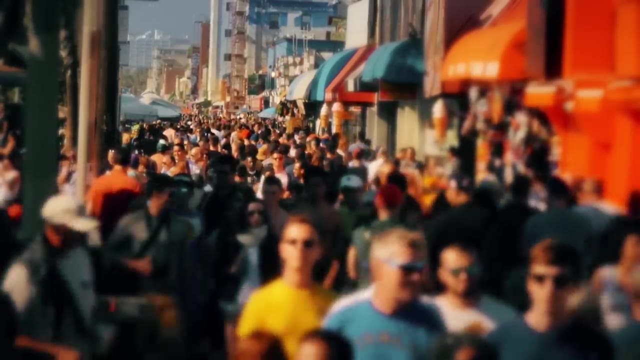 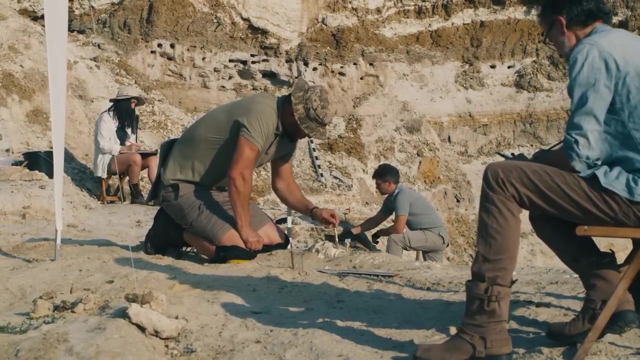 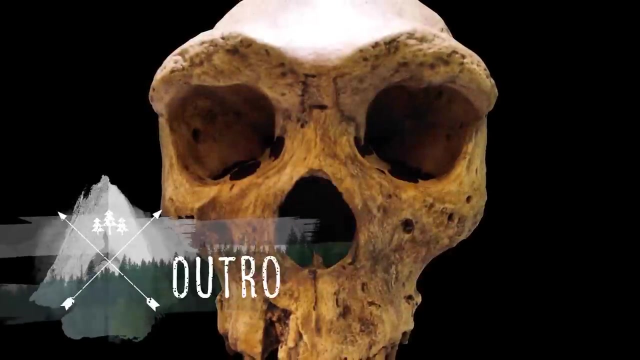 the Neanderthals, later on in the Pleistocene. Obviously, today, it is only Homo sapiens that persist, and we are left solely with important archaeological finds, such as those unearthed in Germany and Spain, to remind us of our lineage. 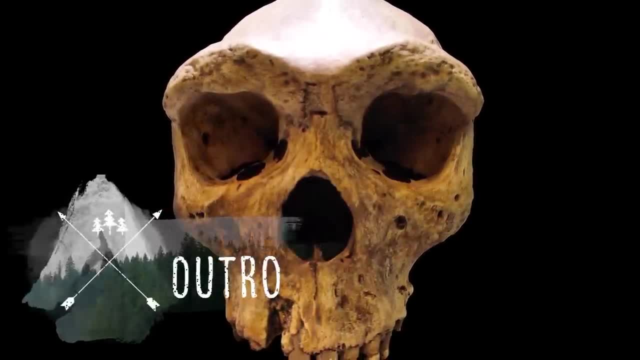 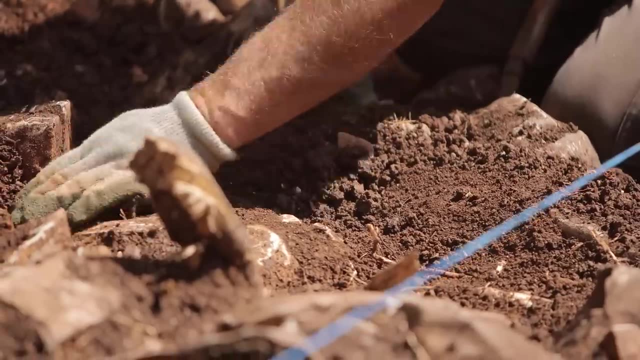 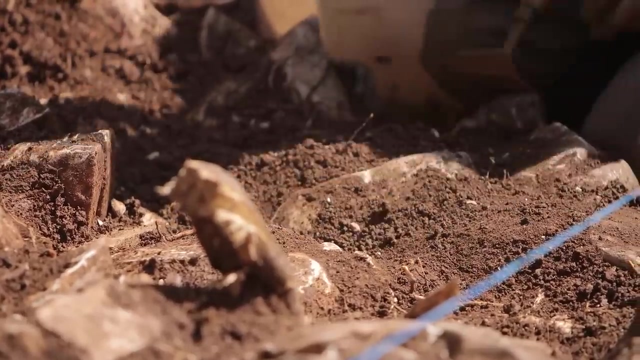 Homo heidelbergensis is a great example of how convoluted and difficult paleontology and archaeology can be. When so many similar specimens are unearthed across the world in such a short period of geological time, it can be massively difficult for scientists to get to the bottom of exactly.